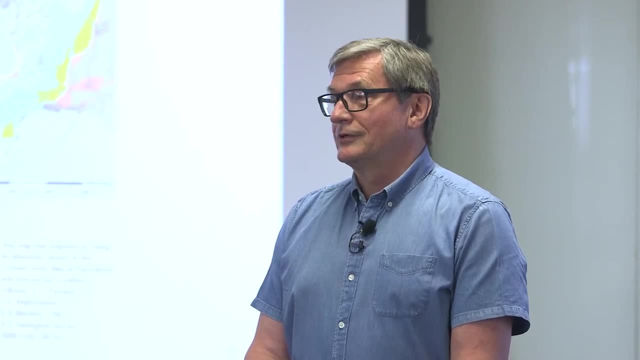 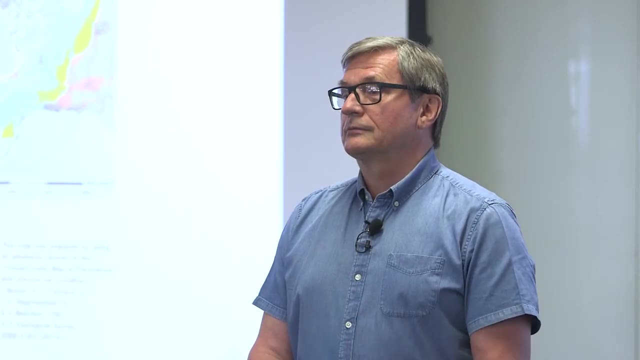 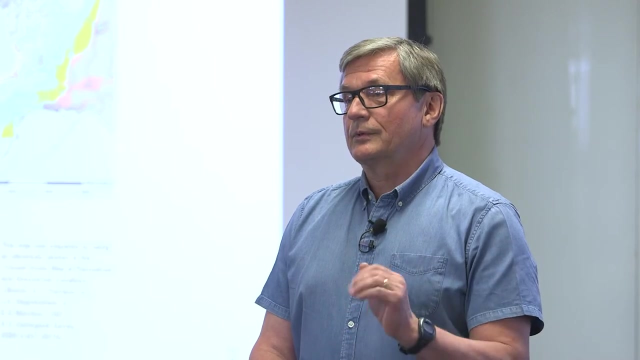 for two hours. So it's kind of a formal definition, but it's convenient, especially for geophysicists, because it's very, very straightforward. If it's below zero degrees Celsius for two more years, that's permafrost. And of course it's not the best definition, maybe because 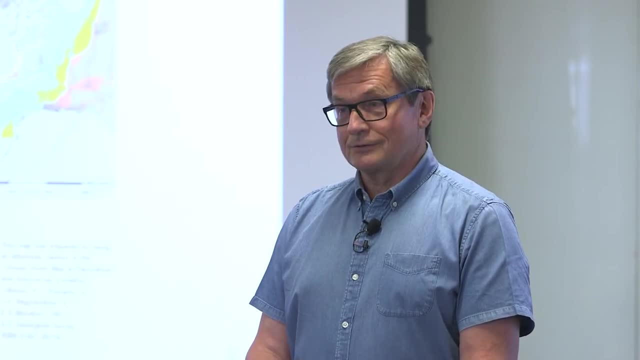 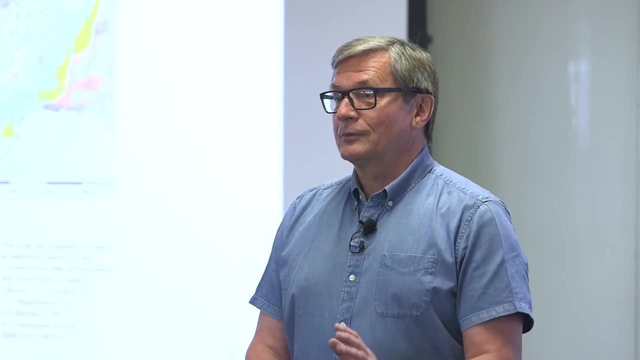 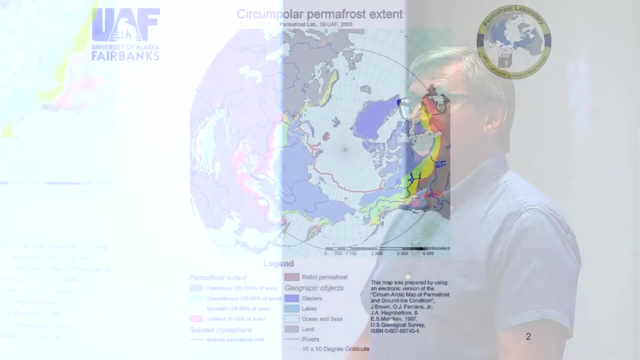 it doesn't say anything about if it's really frozen, if there is ice or not, But let's use it now and we'll talk about ice as well. So it's a product—so this is a map of permafrost distribution in the Northern Hemisphere- Everything. 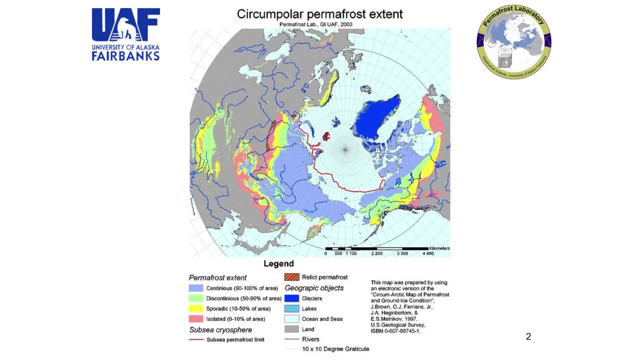 colored is permafrost and gray is non-permafrost areas And the different colors just say some of the permafrost is continuous. That means you will find permafrost pretty much everywhere in that area, which is kind of bluish and discontinuous. other colors—green, yellow. 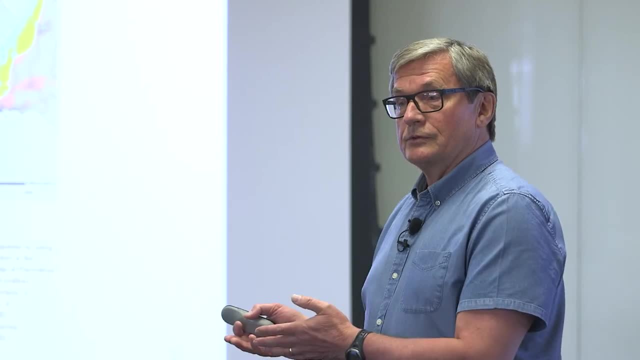 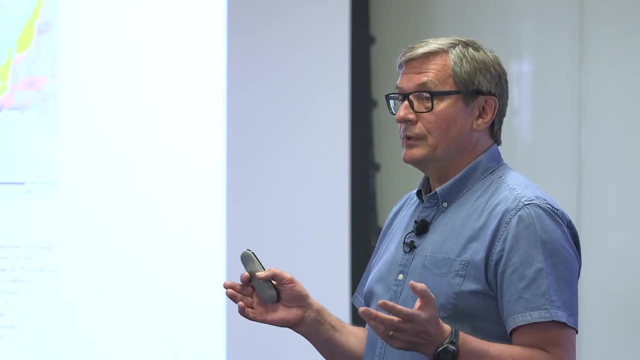 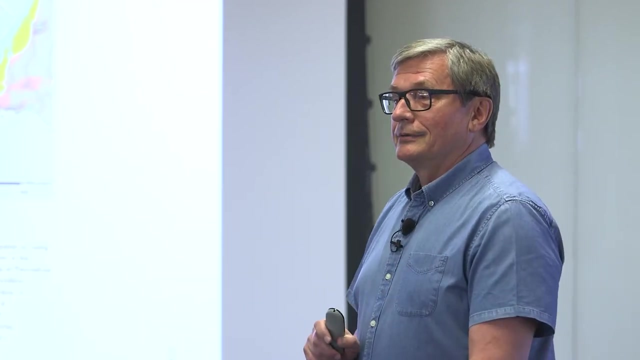 red It means like Fairbanks area, So it could be permafrost in one place and non-permafrost in another place, And it's normal. It doesn't mean that permafrost is disappearing. It's just because of climate as such and conditions—surface conditions, vegetation and so such that in 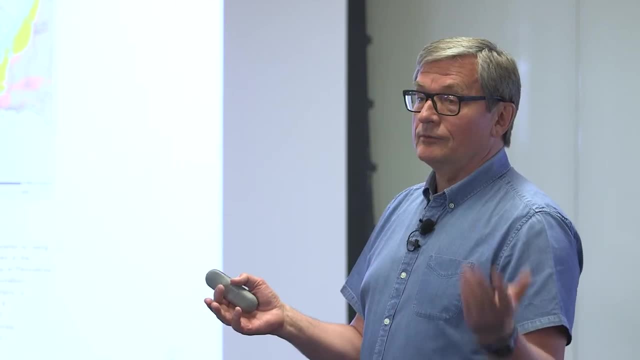 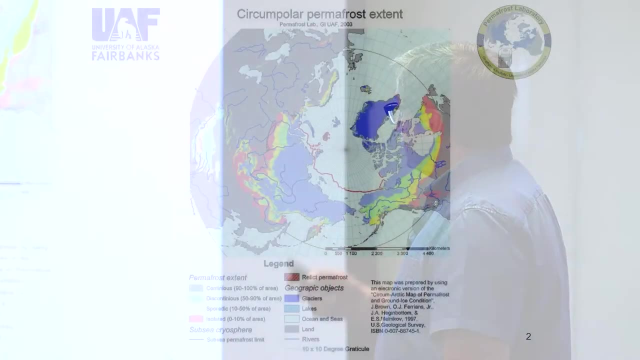 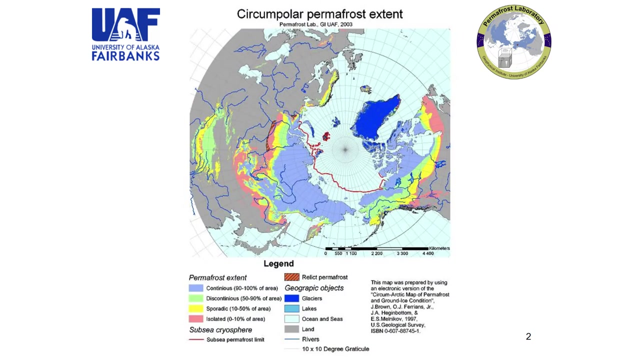 the same climate. because of this variety of conditions you can have permafrost in one case or in one place, or non-permafrost in another place. So obviously we can see even from here that permafrost is a product of cold climates. 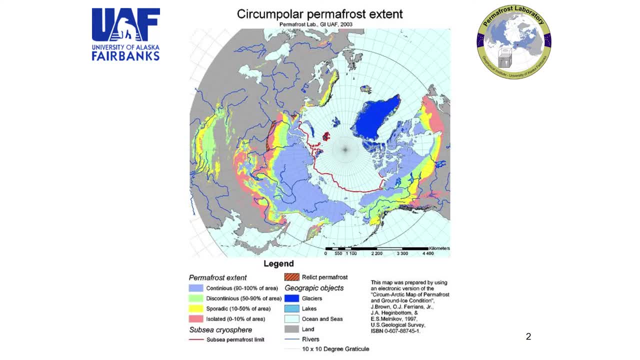 So most of it in high latitudes or high elevations, but for the same reason—low air temperatures. That's the key And because of that, permafrost is well depending on cold climate And because of that, when 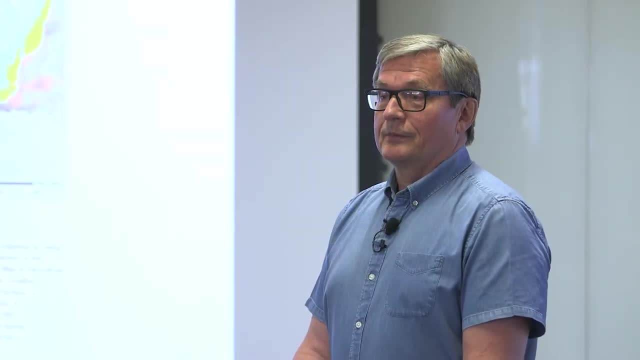 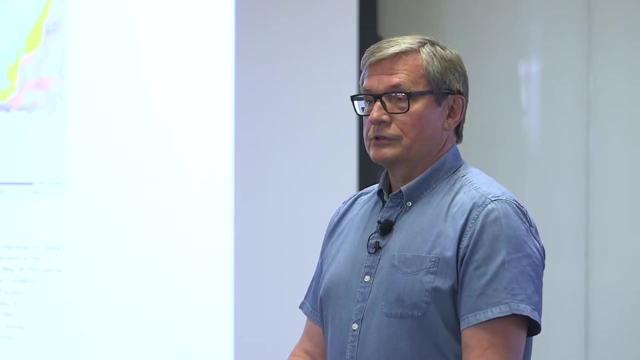 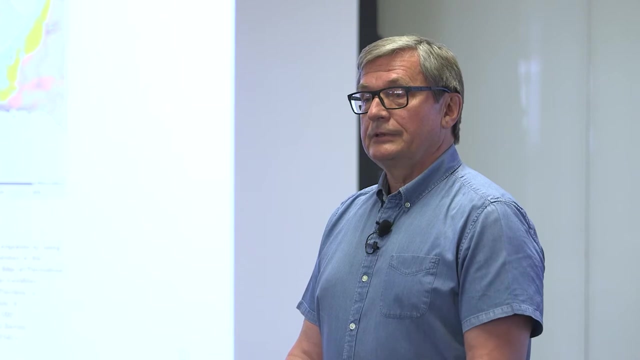 climate is changing, permafrost is changing as well. So if climate is cooling, permafrost feels good extending. If it gets warmer, then permafrost is shrinking, not stable. So it's following climate, not directly, not one-to-one. There's definitely some delay. 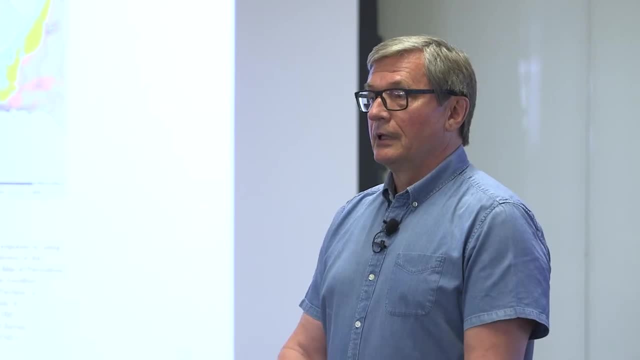 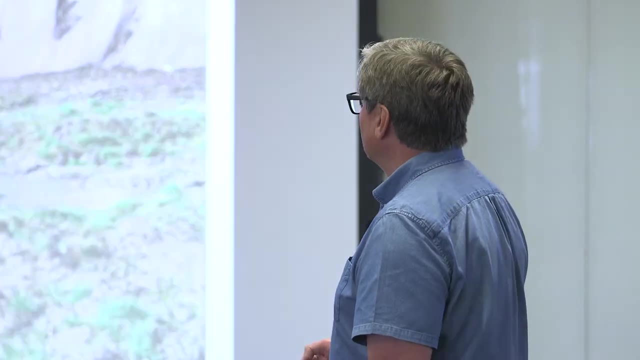 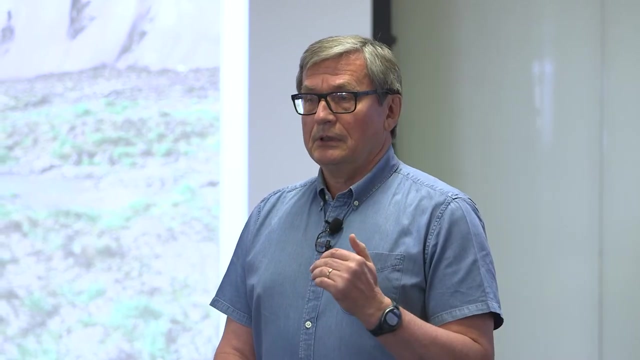 but on a big kind of scale, time scale, It follows climate pretty good. So that pretty much is enough for definitions. but that's about temperature. Temperature is, like I said, very convenient and a very important parameter of permafrost. 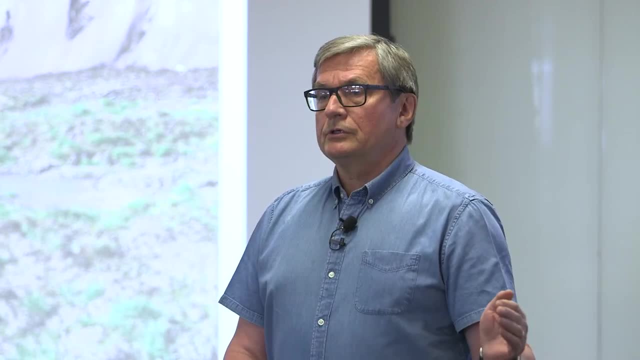 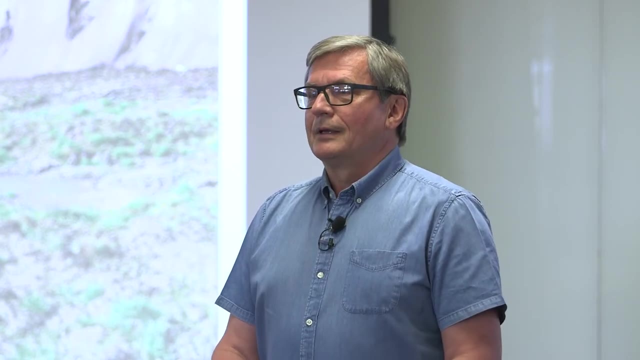 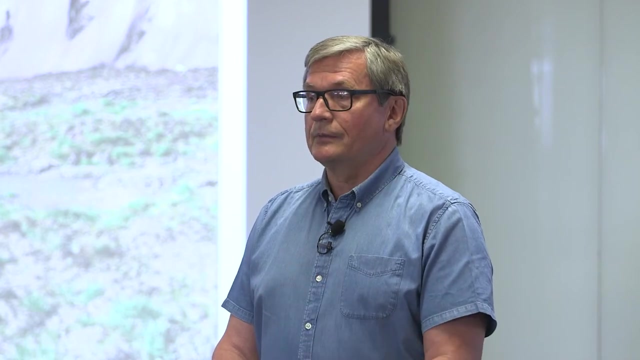 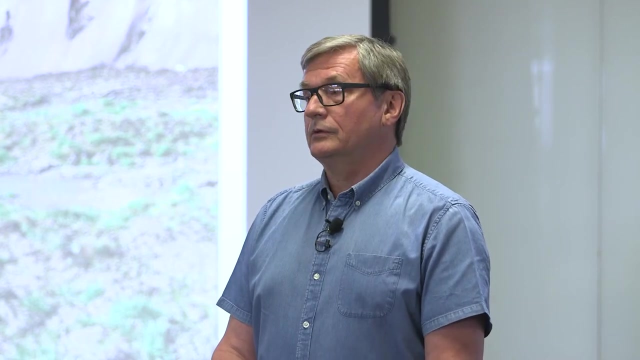 because further below zero, like minus 5,, minus 10, it means that permafrost is stable and you shouldn't worry about it too much, But temperature is rising close to zero degrees Celsius. that's something alarming happening and permafrost may become unstable and start to thaw. So that's why temperature is a very good 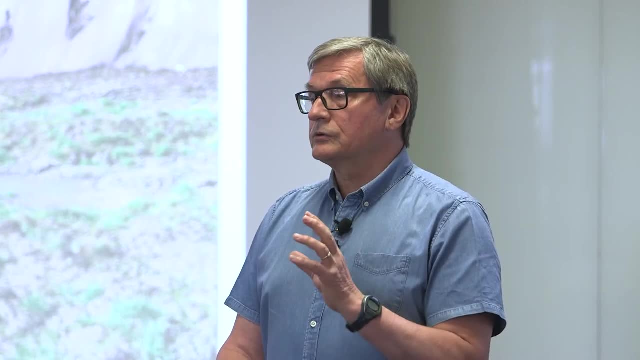 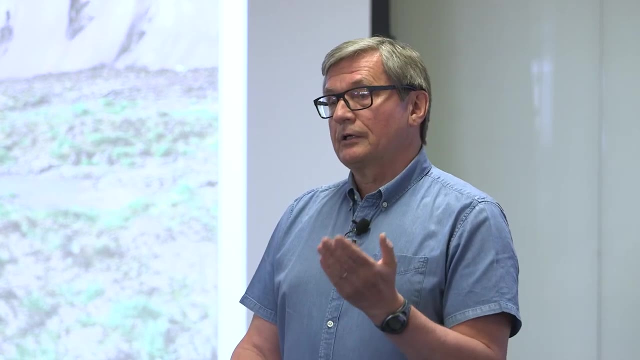 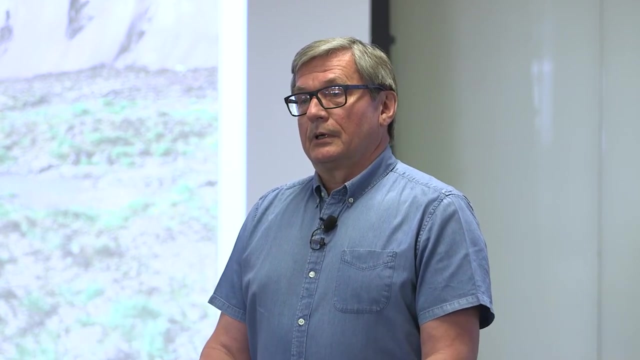 parameter to follow and to estimate how stable permafrost is and how it's changing in time. So temperature is important, exactly to recognize what is stability of permafrost. On another hand- I mentioned about it- there are very important other properties about permafrost. 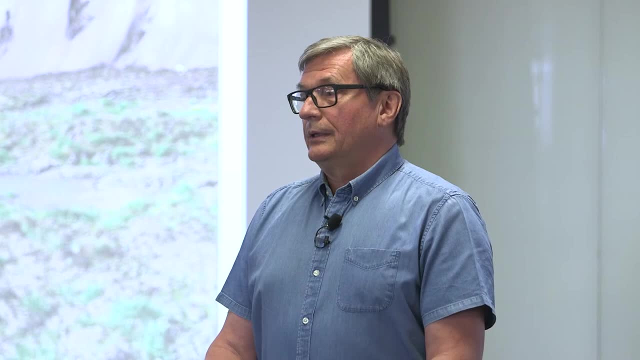 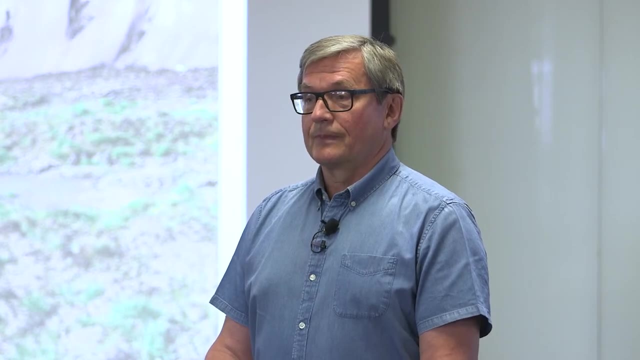 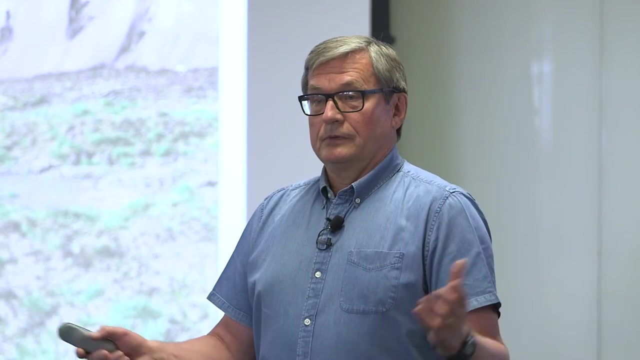 which is how much ice is in it. How much ice is in it is exactly very important for consequences of permafrost disappearance. So if there's no ice in the material, it doesn't matter. if it's below zero, Above zero, there is almost no difference in physical properties and you will not notice. 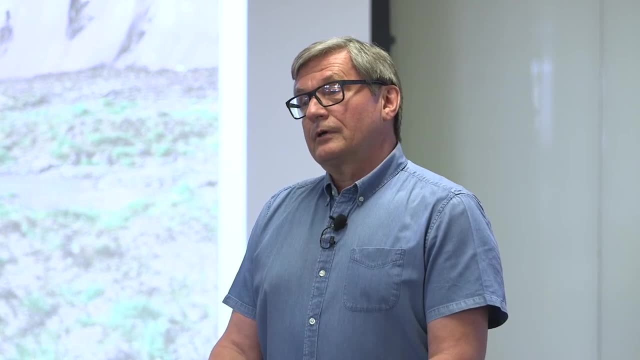 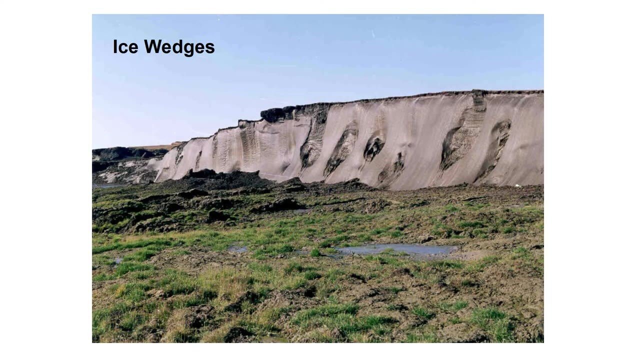 pretty much almost anything. However, if there is ice and if it's lots of ice, for example, on this photo, so this photo is all. this white stuff is ice and dark is frozen permafrost or frozen ground. In this case, of course, ice is included in permafrost, so it is all permafrost, but the 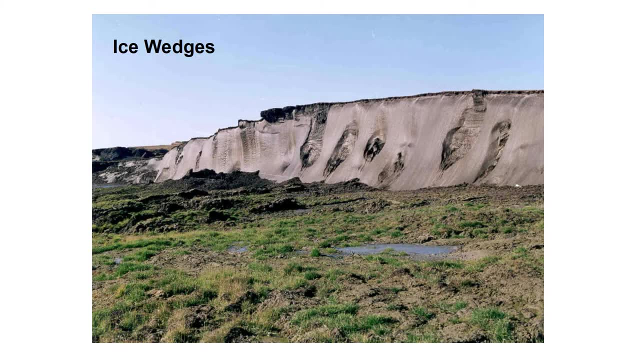 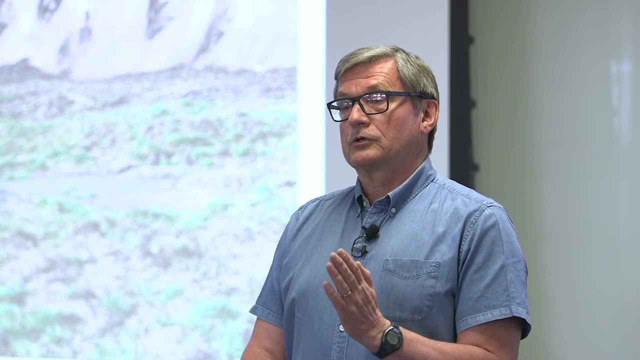 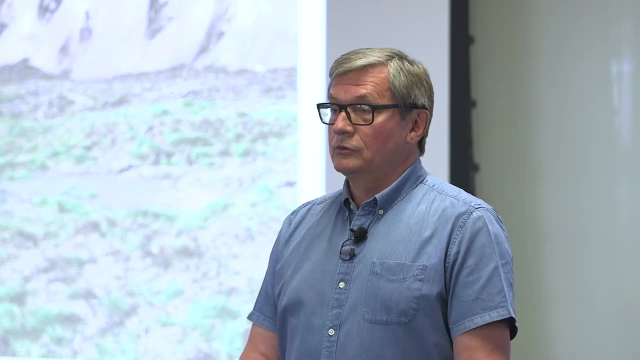 white is almost pure ice. So in this case, if you have lots of ice, of course, the zero degree is really crucial threshold, because, well we know, ice will melt when temperature will come close to zero and try to exceed zero degree Celsius. It will not exceed, though, till all, ice melts. 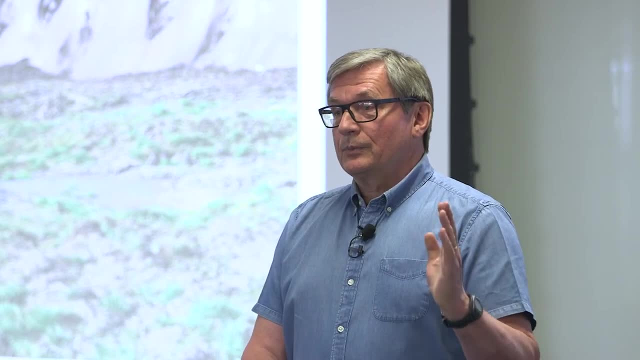 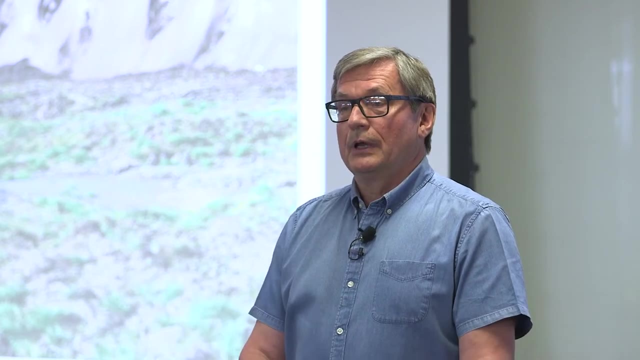 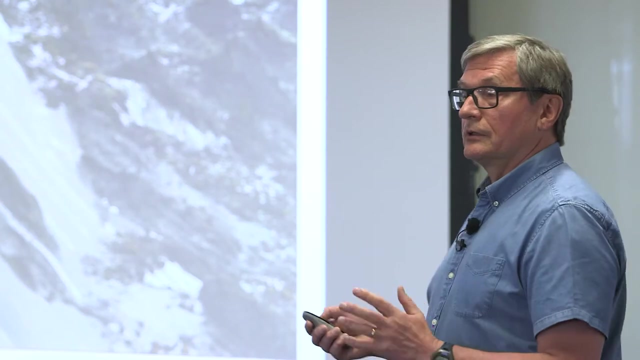 Okay. So temperature is important for stability and understanding where permafrost is going. The amount of ice is really important to understand what will happen if permafrost will be degraded. So I just would like to show several more slides where show the almost like ultimate. 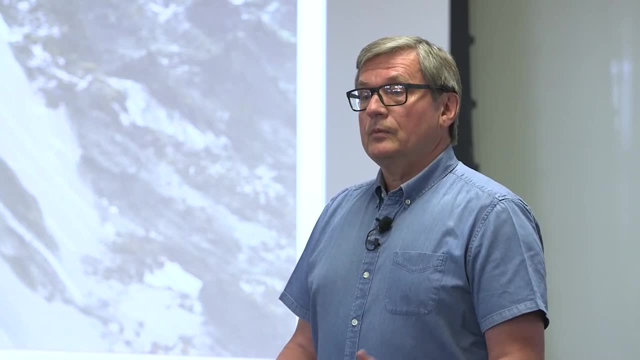 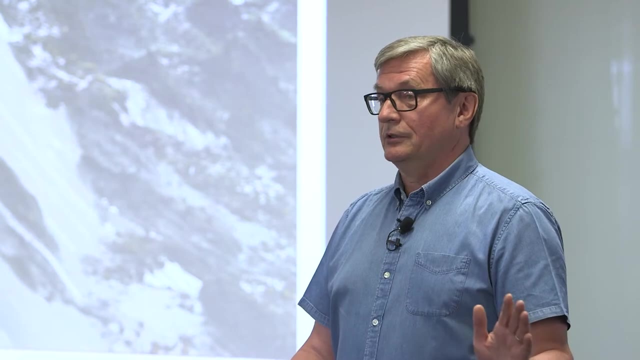 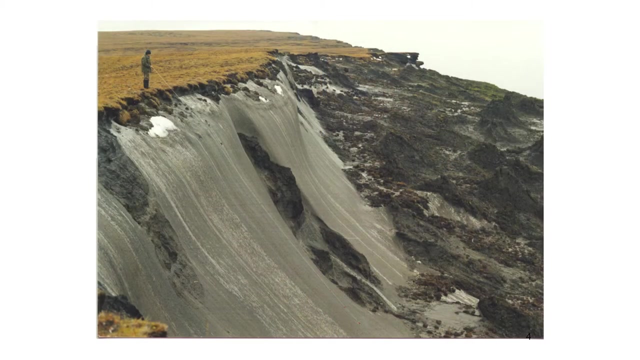 case how much ice it could be in permafrost. So how much ice it could be in permafrost? Well, from pretty much zero. Pretty much zero in bedrock, because by definition, by temperature definition, it's still permafrost if it's below zero degree Celsius to 90-95% by volume. 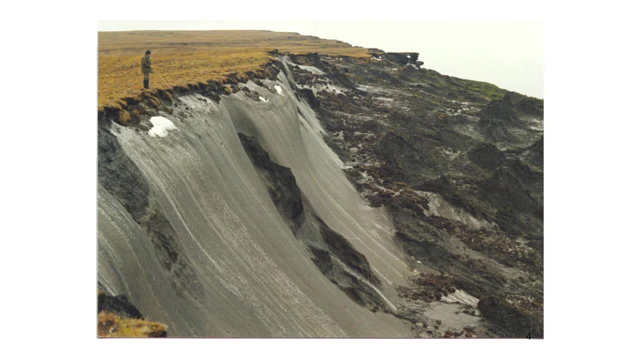 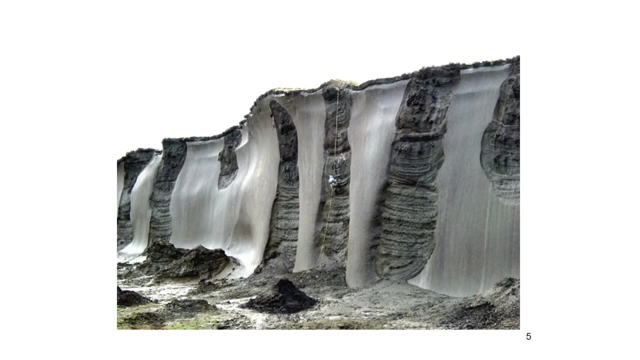 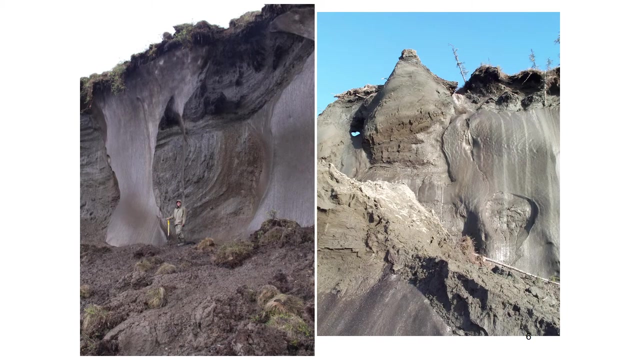 And that's what several. I would like to show the slides which will convince you that it is the case. Like this, all white is permafrost and between it's frozen ground, which at least another 50% of the volume. Some of these pictures taken from Alaska, some from Siberia. 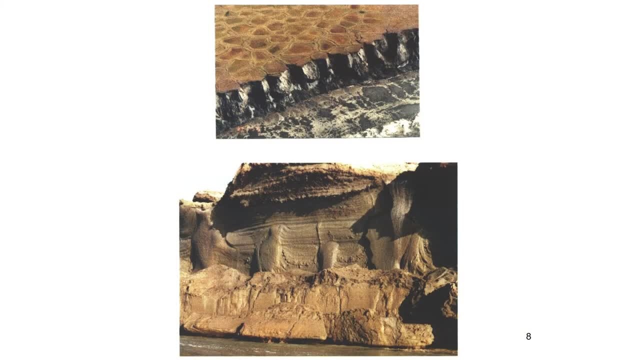 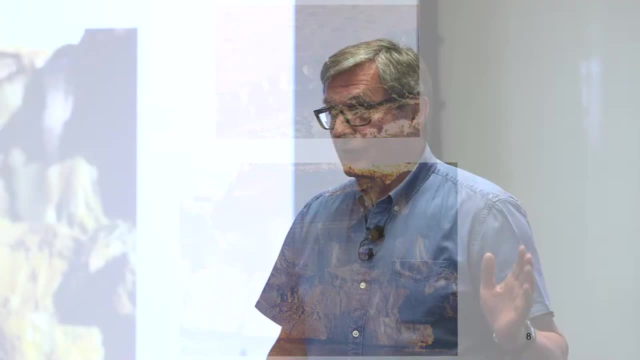 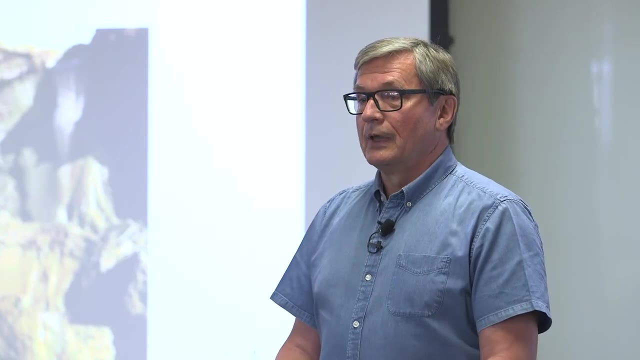 This is Siberia picture. This is also very interesting photo showing that. well, it's whole another lecture how these ice got into permafrost and what shape it could be. But one of the most common, especially in Alaska, Form of crust Classic. 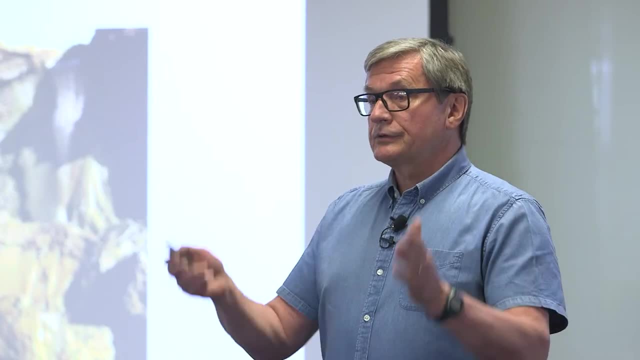 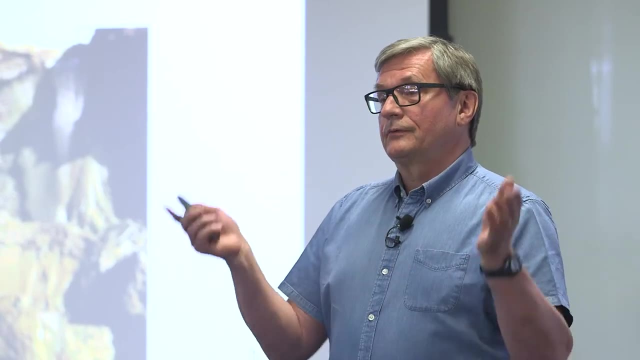 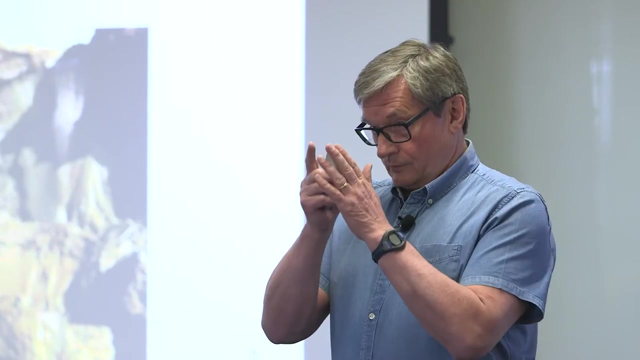 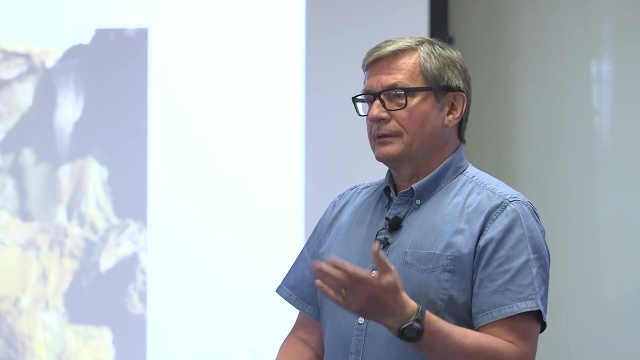 ground ice- more or less pure ice, is ice wedges. So an ice wedge is formed because of cold climate cracking the ground, filling these cracks every year summer with melt water from snowmelt, developing small lengths of ice vertical which goes down to five meters. 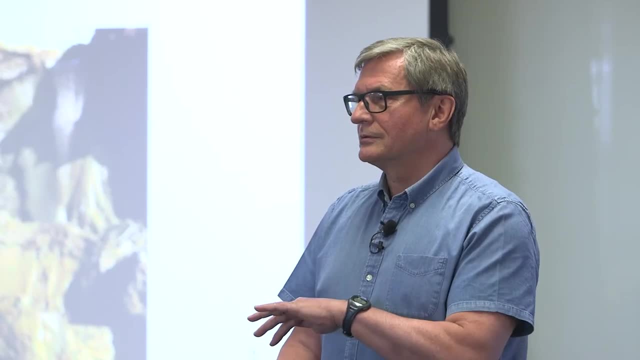 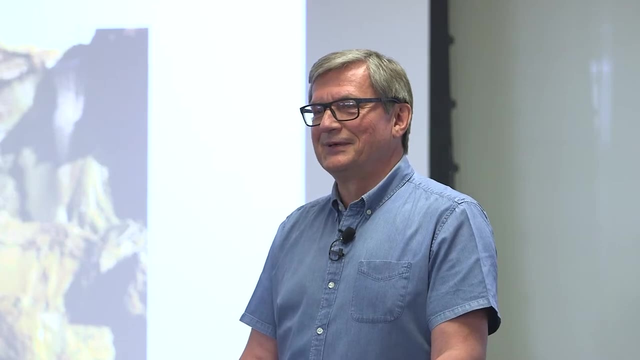 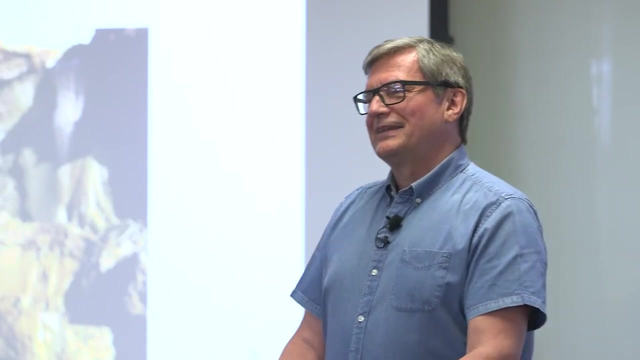 I will mostly say meters. If you like, I can switch to feet, But as a scientist in European origin, meters are still more convenient for me. But you can do it. If not, I can try Fifteen feet, How about that? And every year very, very tiny, like maybe two centimeters. 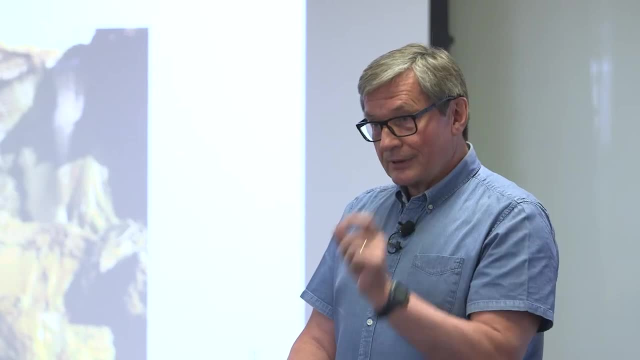 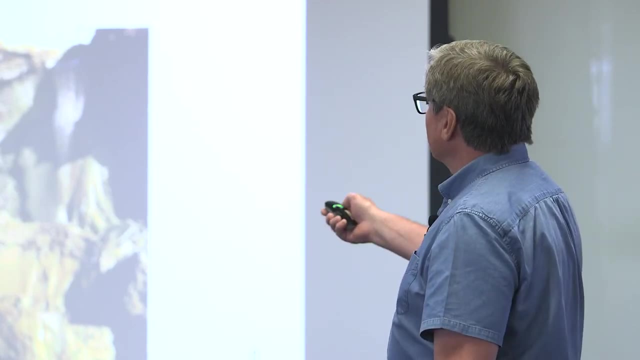 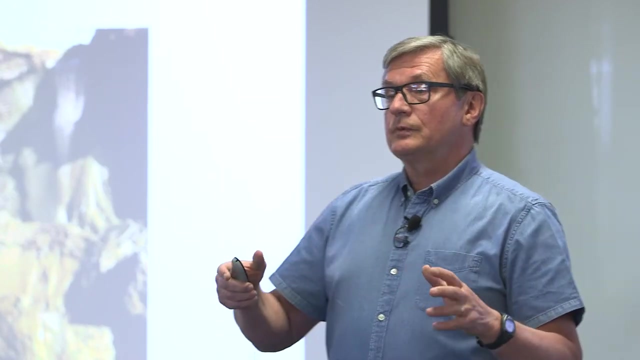 ice wedge will appear, And then next year, and next year, and next year, And eventually it can become ice. It can grow like this, But what is interesting? that oops, sorry. If you look from the surface, these ice wedges develop so-called polygons- ice wedge polygons- And they could be different. shape: rectangular or maybe hexagons or pentagons. It depends on property of material really, and thermal conditions. But from the looking from the top, it's actually formed some sort of like a honeycomb thing, where the you know honey is actually less ice And the borders are it's ice wedges. 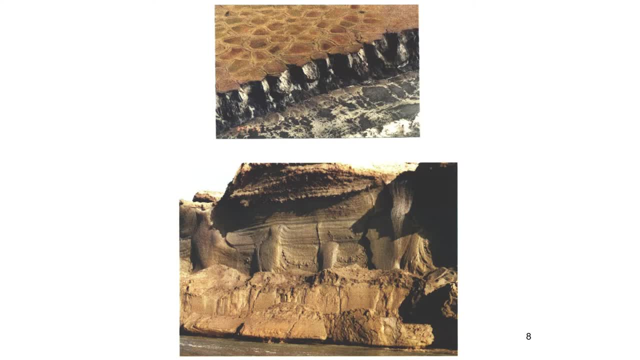 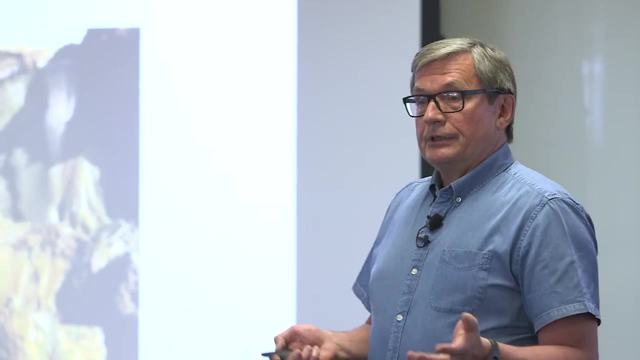 so lots of ice there And you can see this is taken from the same place. This cliff is that's what you see is a cross, But on the top it looks like this. So ice wedge polygons- And I will mention about the ice wedge polygons- We will be talking about degradation, maybe. 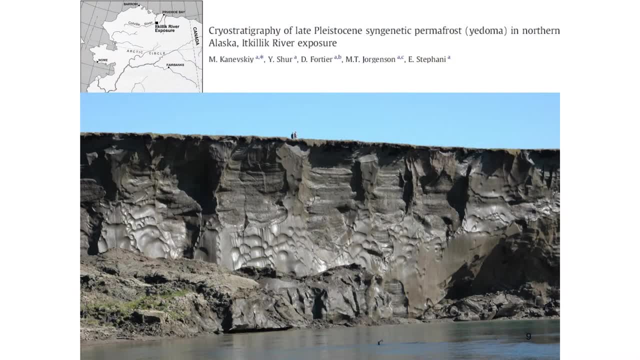 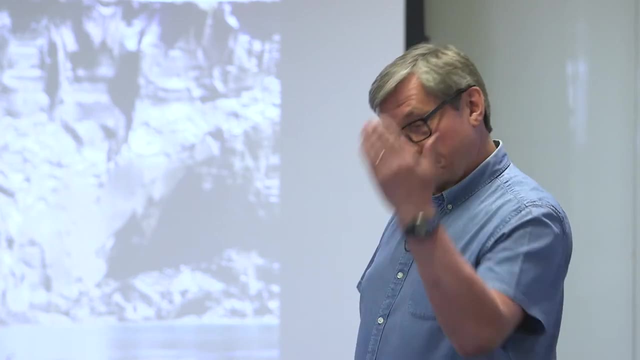 or it's good to know. This is actually from Alaska, published by Misha Konevsky, Yuri Shura and co-authors. This cliff is about 30 meters, almost 100 feet tall, And you can see that from there. 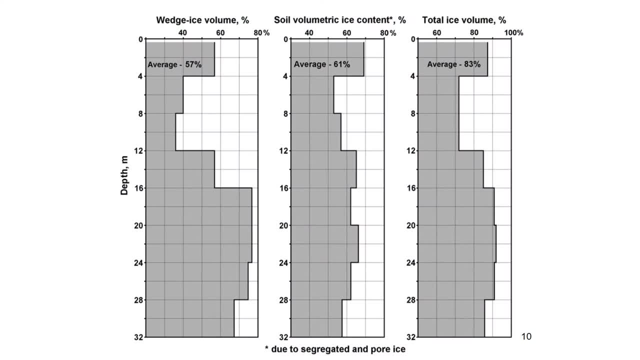 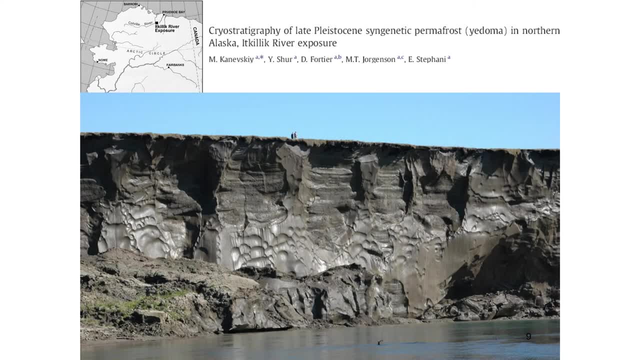 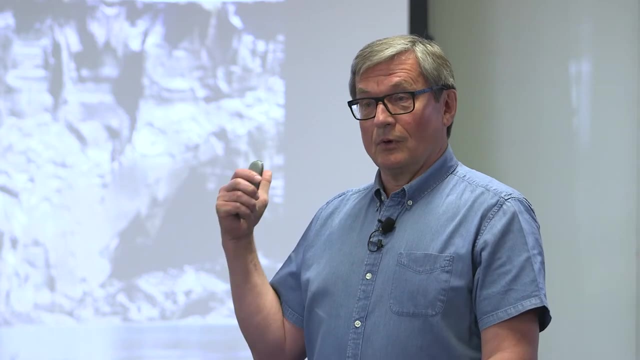 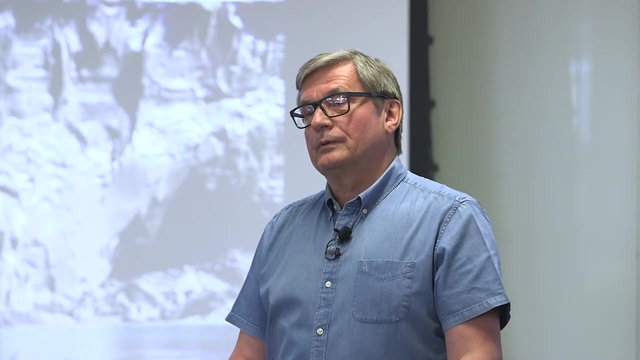 There is sediments involved. So now imagine 100 feet all ice melted, 90%. So only what 10 feet will be left out of the ice? And all this, all this big cliff. So that's kind of keep in mind when you think what will happen to the landscapes. 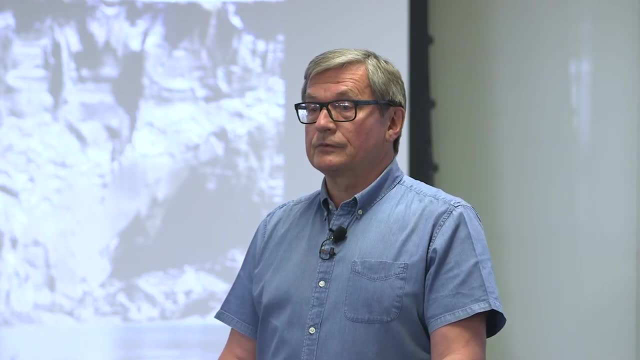 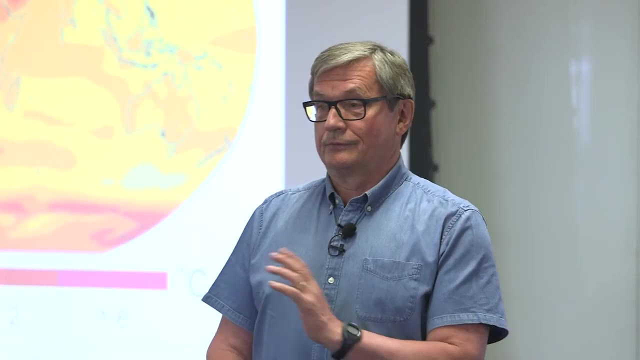 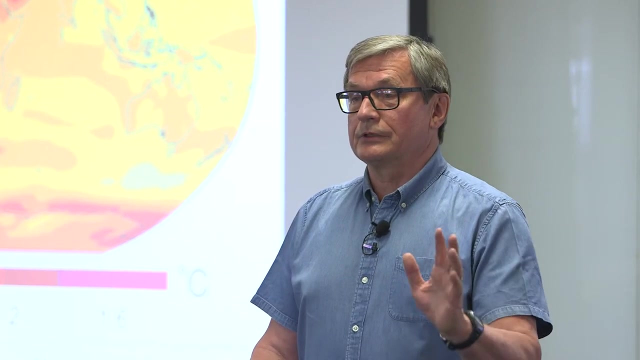 when this kind of ice-rich permafrost will be thawing and ice will be melting. All right, Now go back to temperature first. So in the past, when I started to study permafrost in mid-70s- 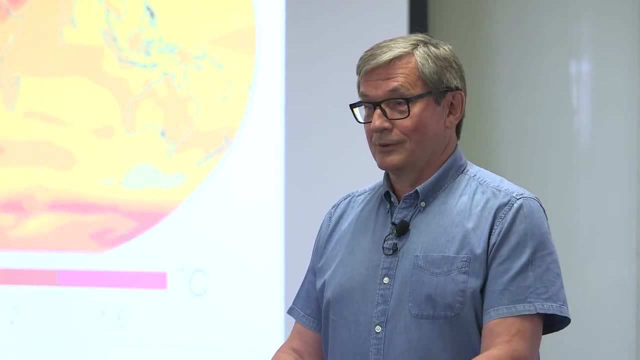 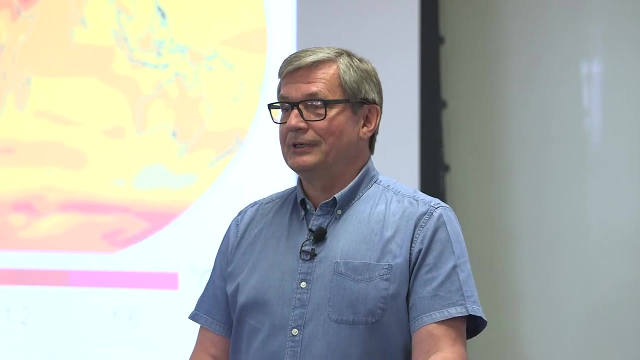 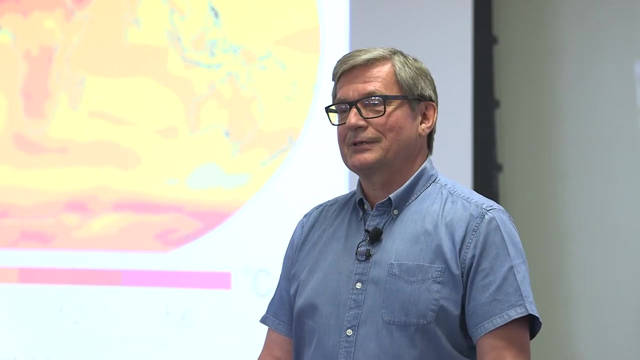 there was no global warming, It was actually global cooling. you probably remember, And all media was excited about new ice ages coming. Well, at that time we were still excited about studying permafrost as a geophysical kind of matter. subject: 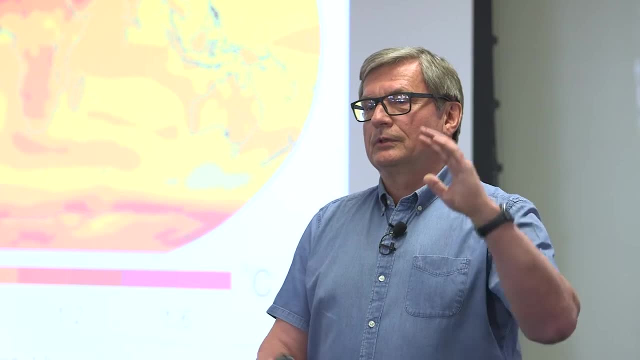 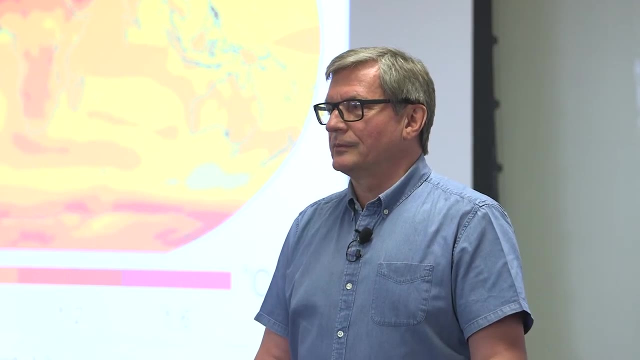 But in that time we were thinking about big changes between glacial periods into glacial periods like tens of thousands of years. So it was a very, very long time frame. It's still very exciting, But it's mostly kind of academic interest. 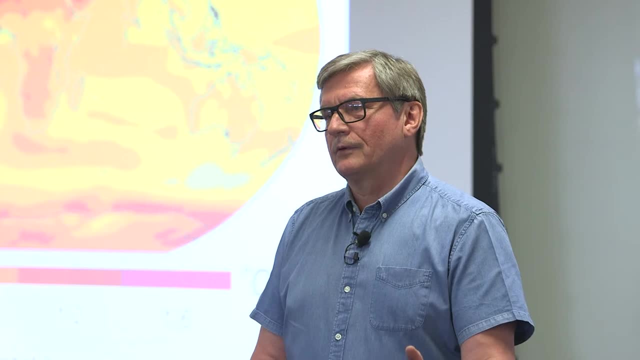 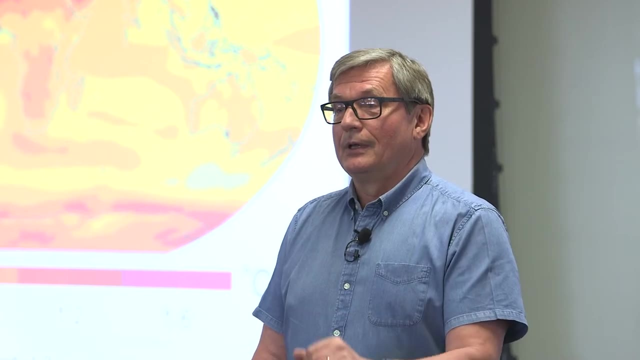 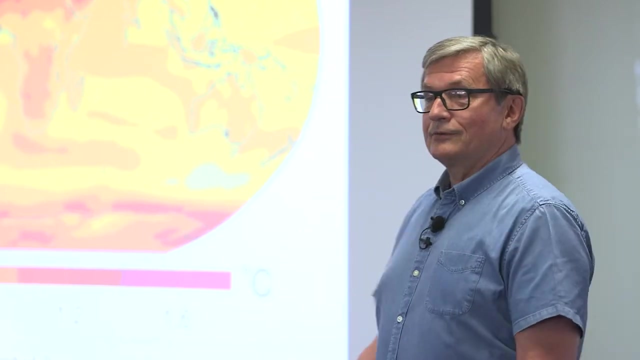 But all permafrost science was developed during this, from 50s to 70s, most of it- And the assumption was that permafrost is permanent. That's why permafrost was its abbreviation of permanently frozen ground. Well, fortunately for us, to make it more exciting, even climates started to change. 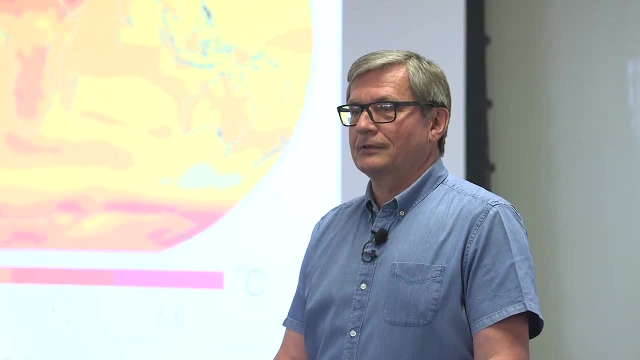 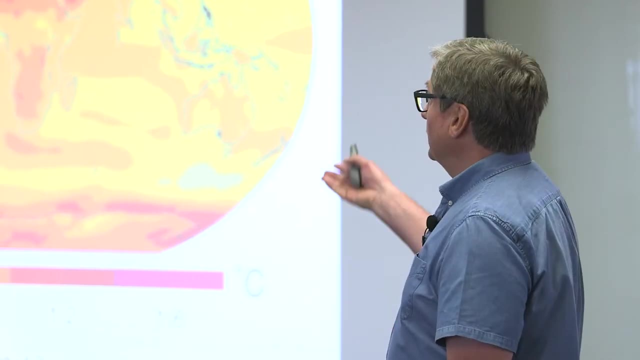 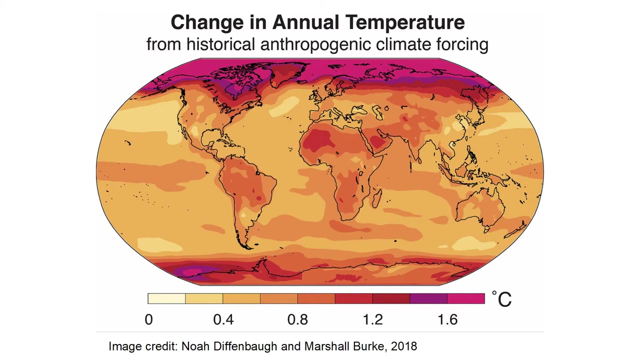 And change in the direction which is definitely not in favor of permafrost. So warming which up to now already very well established and exceeds some one, one and a half, two degrees warming in the high latitudes, globally maybe one degree Celsius. 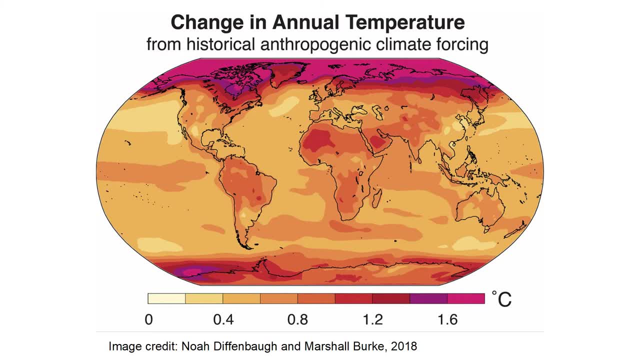 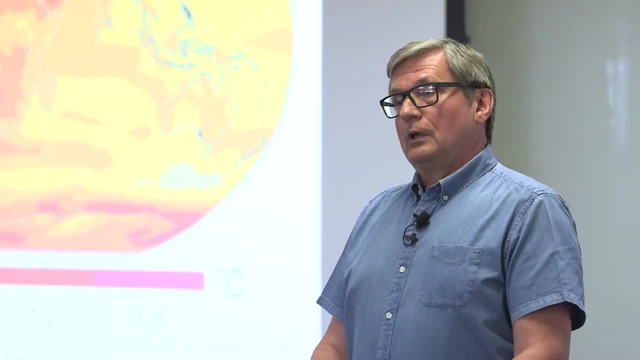 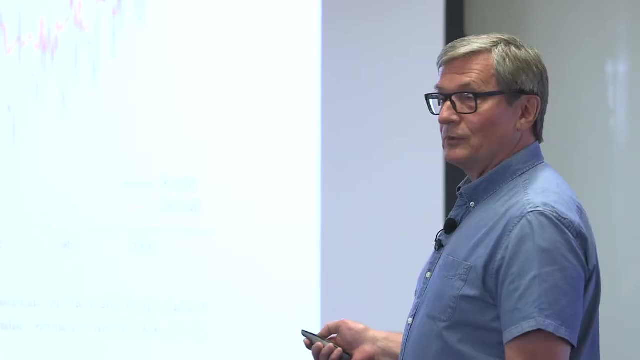 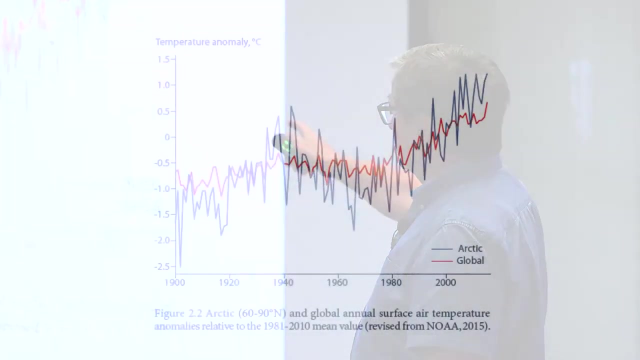 warmer now than it was in, say, mid-20th century. And, of course, permafrost. Yeah, Permafrost reacted to this warming, So how do we know about it? Well, one more slide here, But now it's kind of all averaged by global. 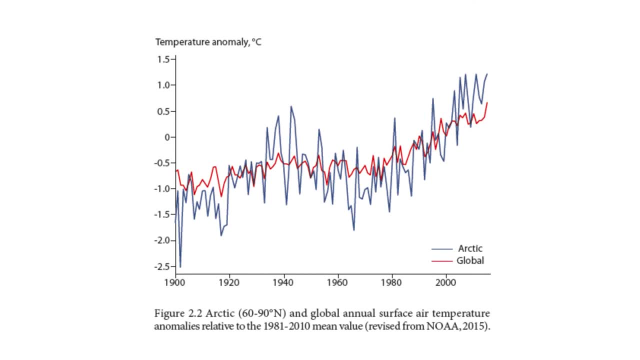 It's red And Arctic is blue, And that's what I said about how much warming happened. And you can also see that higher latitudes are reacting to this warming, This warming more actively, more amplifying so-called polar amplification in climate. 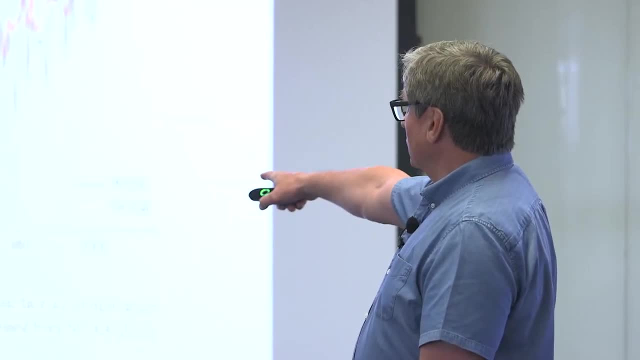 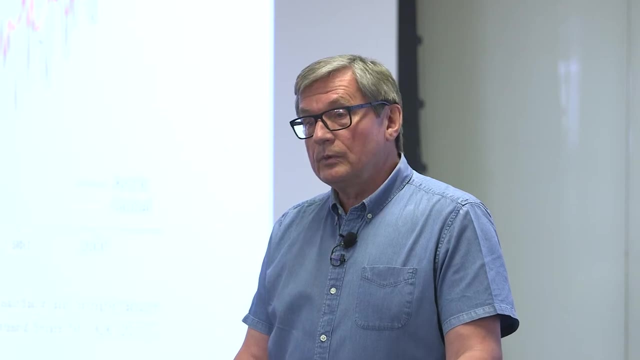 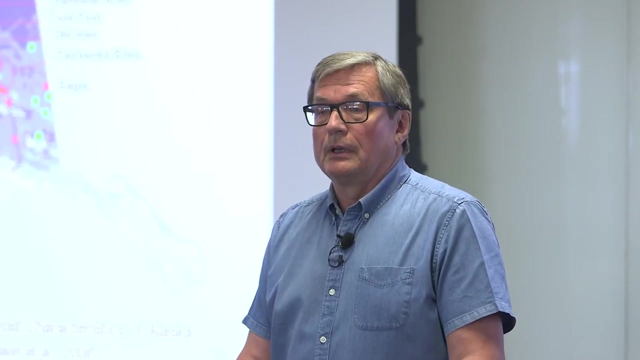 So that's why, for high latitudes, compared to those 70s, we are like two and a half degree already warmer than it was then. Globally it's still one degree warmer. So how do we know? Well, fortunately, in the University of Alaska Fairbanks, the University of Alaska Fairbanks. 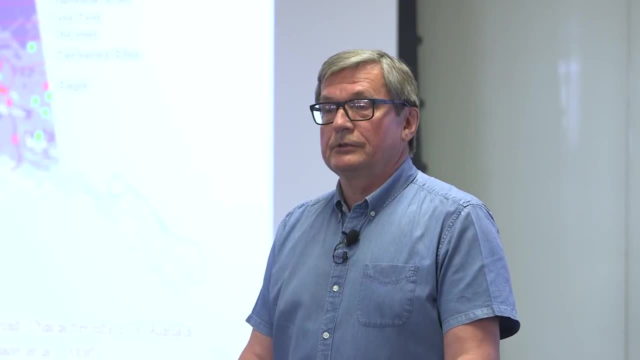 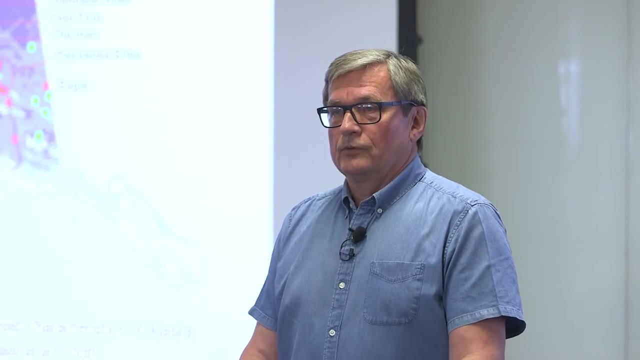 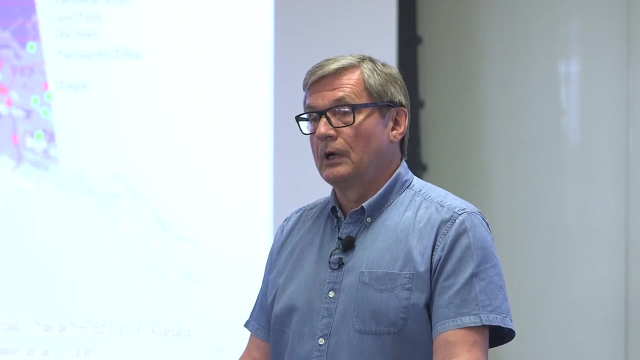 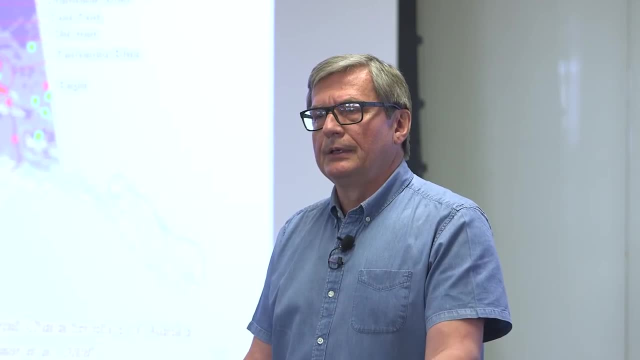 Emeritus Osterkamp. He established at the very, very beginning of this…first kind of observations that we are showing the climate is getting warmer, So he established a transect of relatively deep bore holes, like maybe 60 to 80 meters. 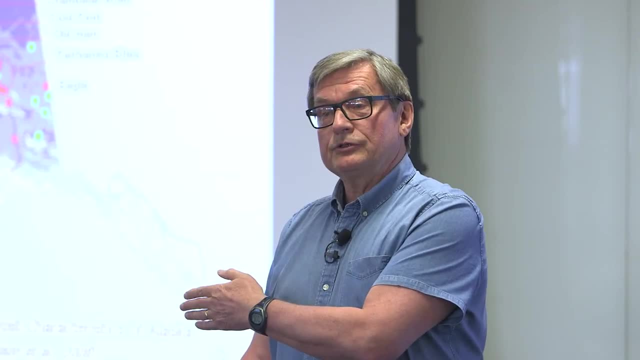 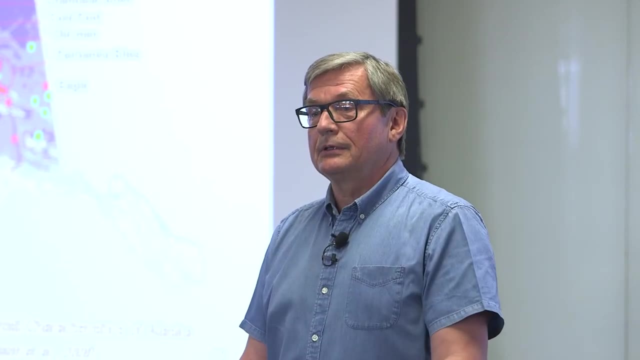 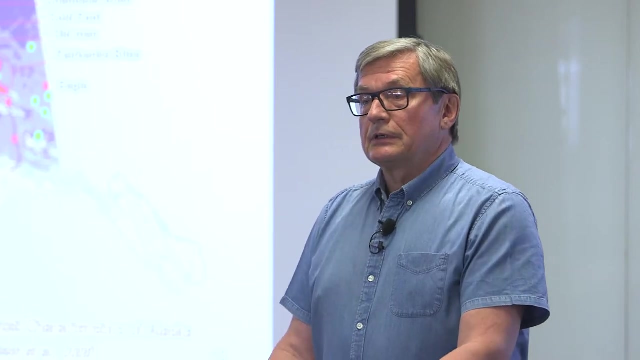 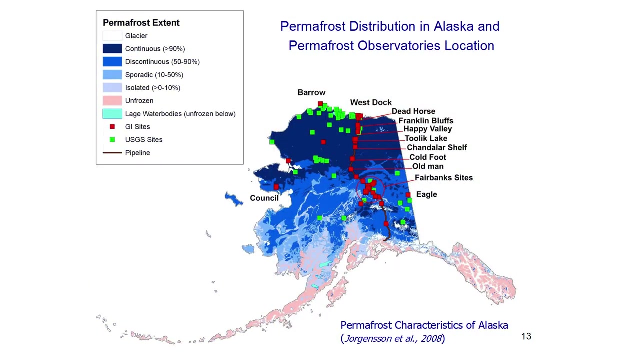 about every 14 miles from southern edge of Promo Frost somewhere in Glenallen, Kokona to Prudhoe Bay very conveniently along the highways Richardson and then Dalton Highway. And it was established in early 80s And since then on this map this borehole is shown in red red square. 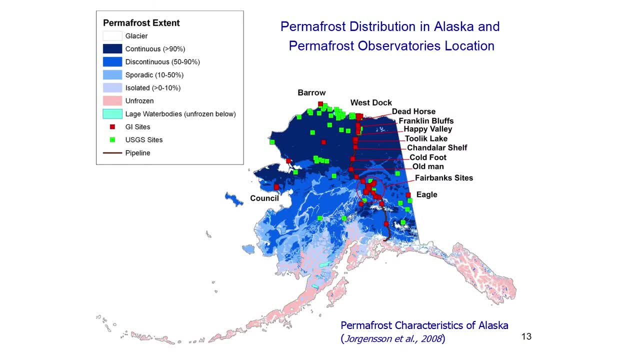 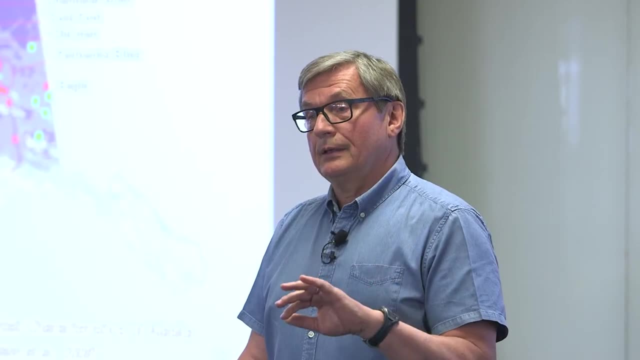 Another big player in this game was US Geological Survey, which used geological boreholes much deeper, like 50, 500 meters and even deeper, which were used for geological purposes, But then, after they were drilled, the temperature started to measure in these boreholes. 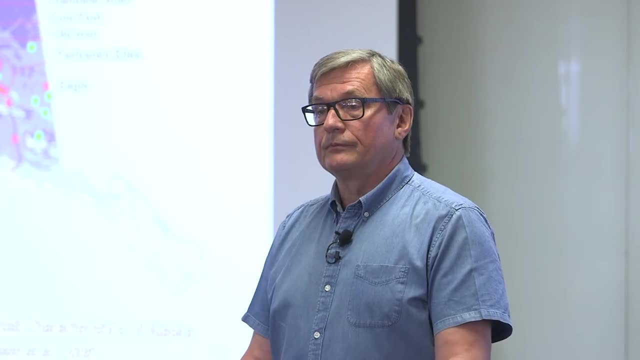 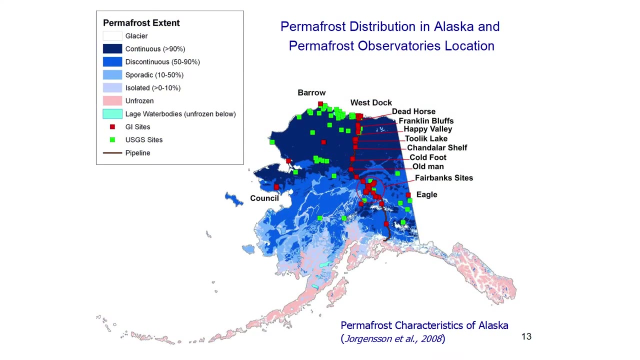 And we also have a very long record about the same time, Some of them actually even earlier than that. In the early 80s, at some places like Barrow there was some very good records of Promo Frost even starting in the second half of 50s- 1950s. 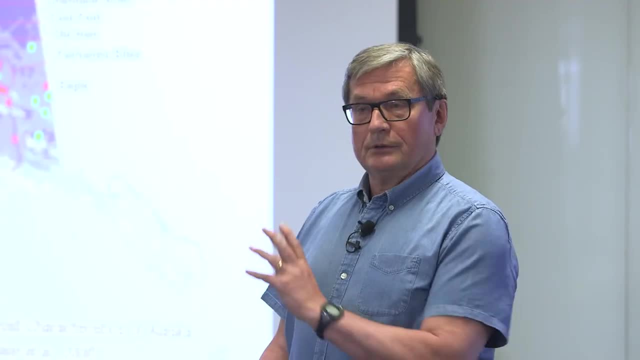 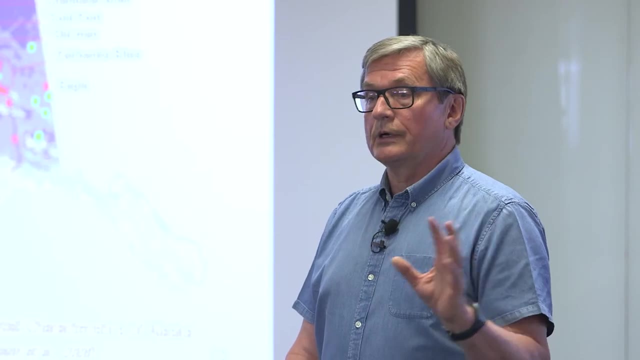 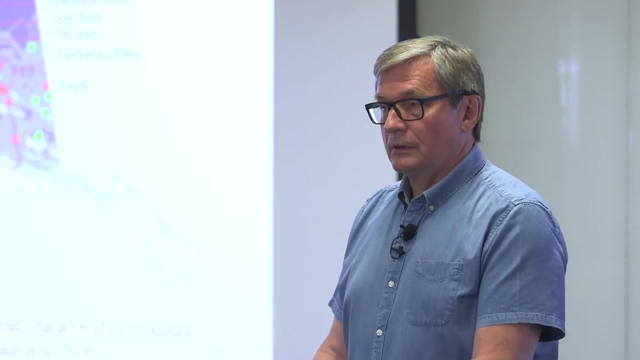 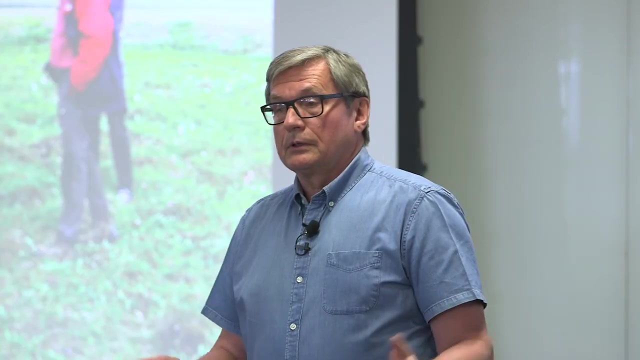 So, since I will be talking about our set of data- and now there's more players involved, There's more organizations- federal and state organizations start to measure temperature in the ground to see what's happening, to Promo Frost. So we use some different sensors and different technique to record this temperature. 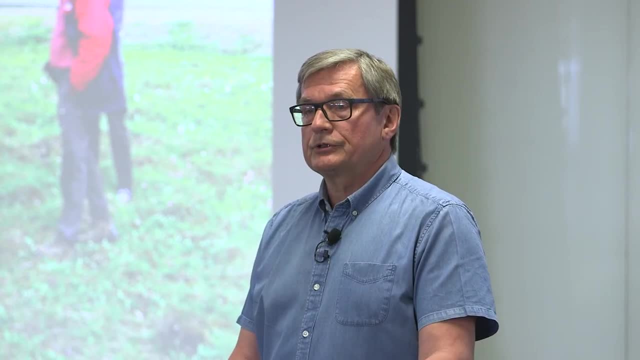 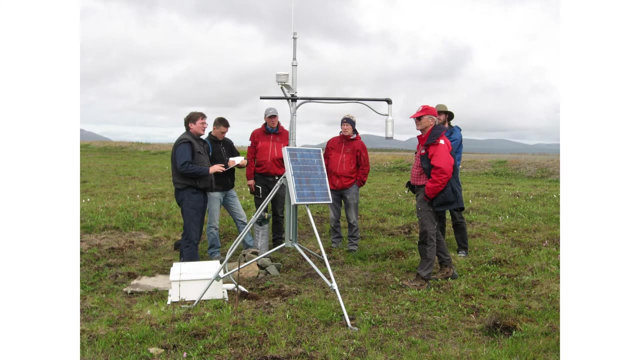 But it's more or less standard. So we do this pretty much the same way in all these boreholes- And we have not only deep boreholes- which is here, It's about 65 meters borehole- But also we measure temperature. 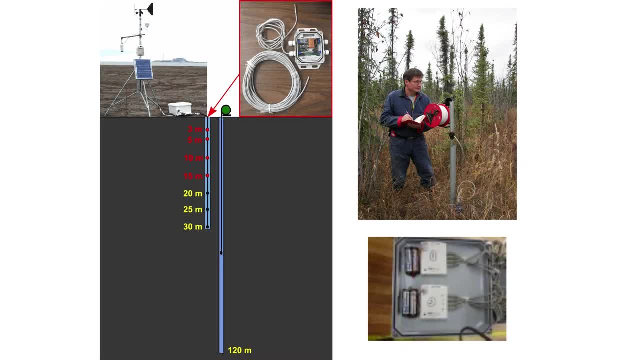 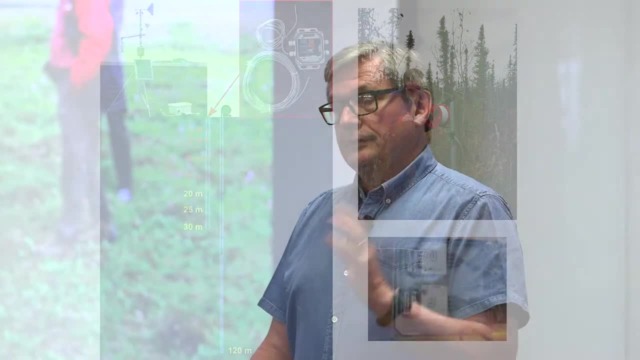 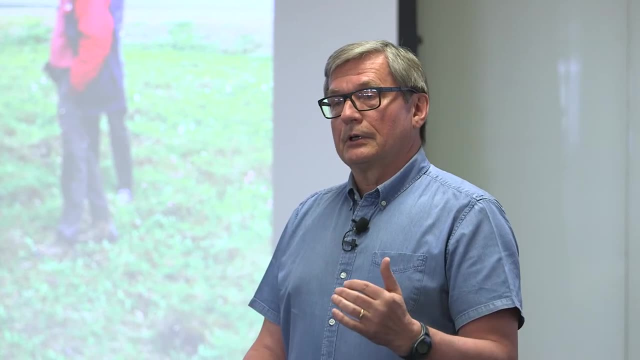 But it's every hour actually, in a shallower depth, down to 3 meters, 10 feet, And also we measure other things like air temperature, snow depth, soil moisture And all these records. we collect this data to understand well, first of all, how this. 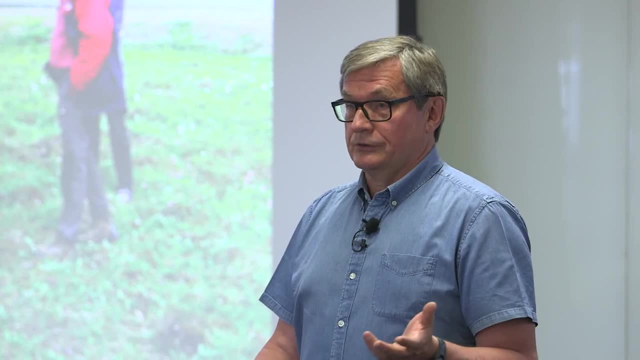 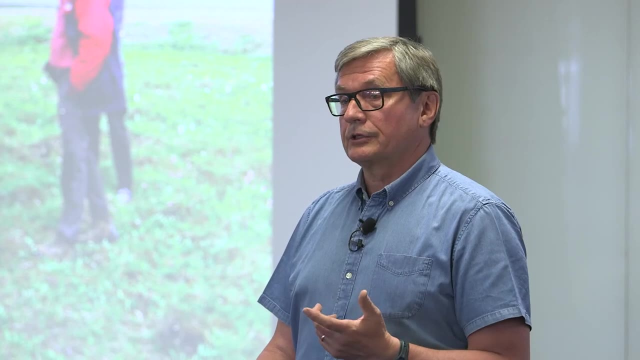 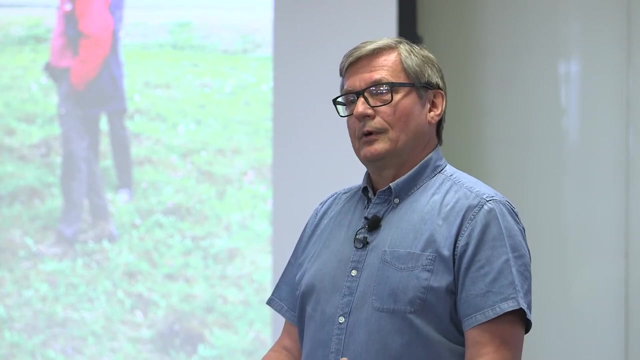 temperature changes and then why it's changing, And then when we understand why we can actually monitor. So in our lab we're not only measuring temperature but we also do developing pretty sophisticated Promo Frost models which you can predict well project how Promo Frost will change. 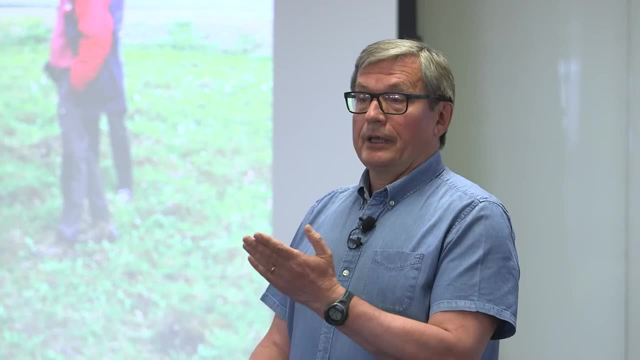 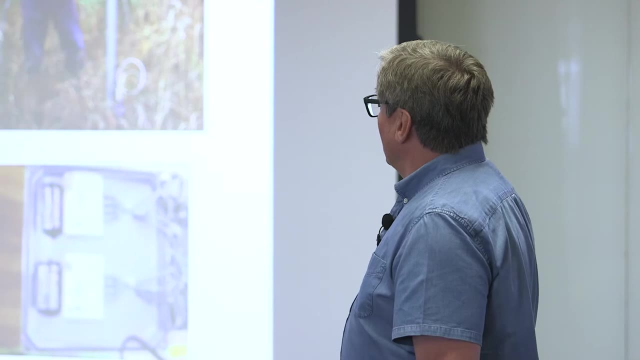 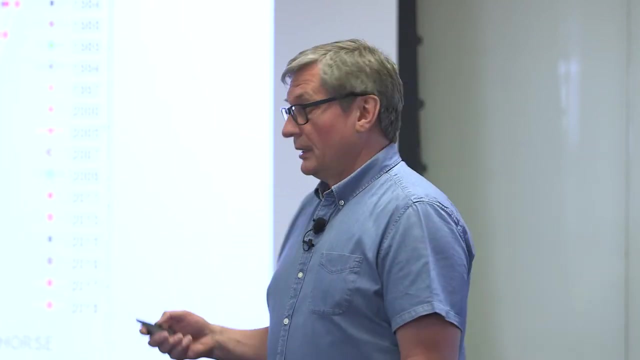 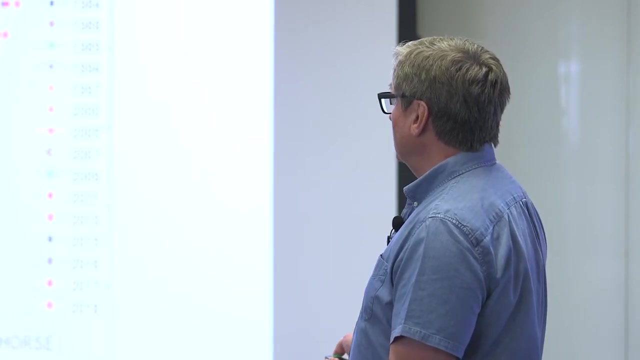 in the future, assuming one or another climate change scenario, of course, Because, again, climate is the driving force of these changes. So what kind of results? How will they look like? So a very, very typical presentation of this data will be: so every year we do these measurements. 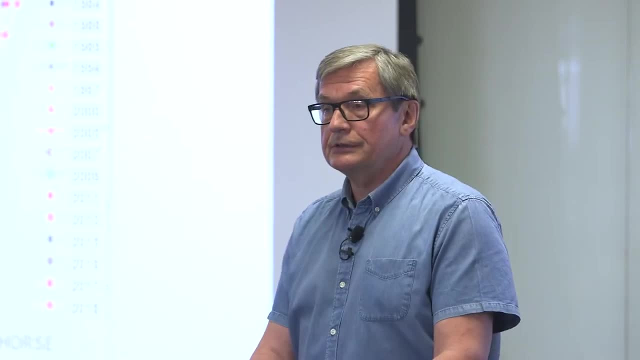 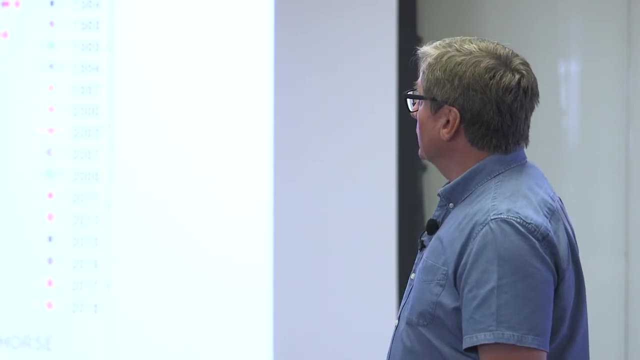 This is in meters, so 20 meters to 55 meters. in this case It's Dead Horse Borehole near to the airport, like 5 miles south from the airport in Dead Horse, Prudhoe Bay, And temperature was measured every year. 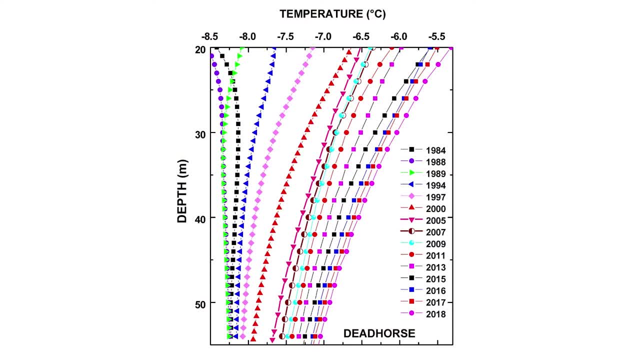 But once a year. That's why we interpret only this data. That's why we interpret only this data, This part, Because above 20 meters there is some seasonal variations of temperature, But below 20, there is no seasonal variations. 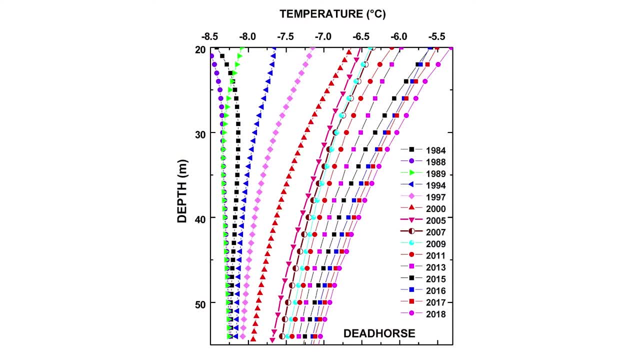 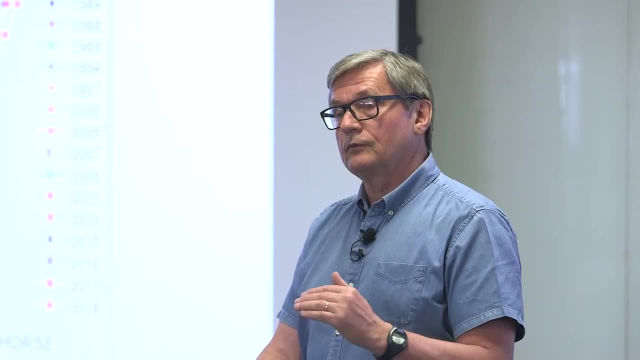 All seasonal variations disappears in the upper part And we can see this as a reaction to climate change, So it's kind of long-term changes. So it's very good for us because Promo Frost is a natural kind of low-pass filter, So it filters all. 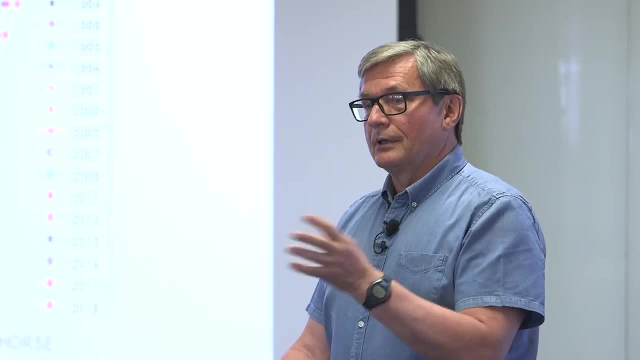 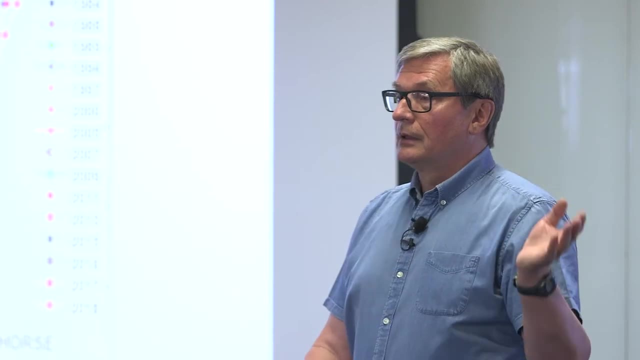 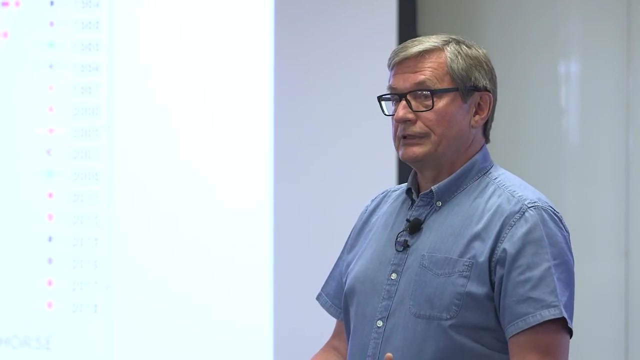 Yeah, So we can see diurnal seasonal variations and then we can see the signal, the climate signal. That's why we can see it actually much sooner than atmospheric scientists or climatologists, because they are dealing with very noisy data of air temperature. 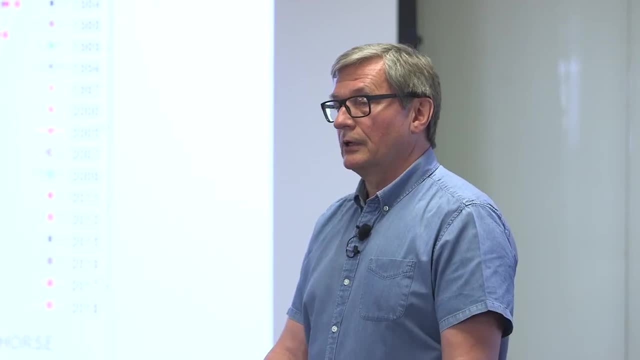 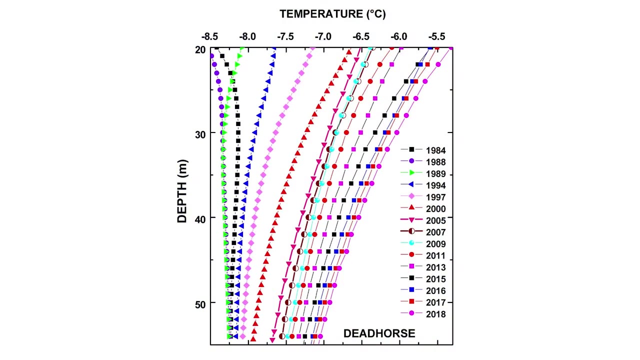 So in Promo Frost temperature all this noise is already gone and we can see very clearly what happened, what have been happening here. Yeah, So it was a little bit of cooling after we start to measure it in the mid-80s. 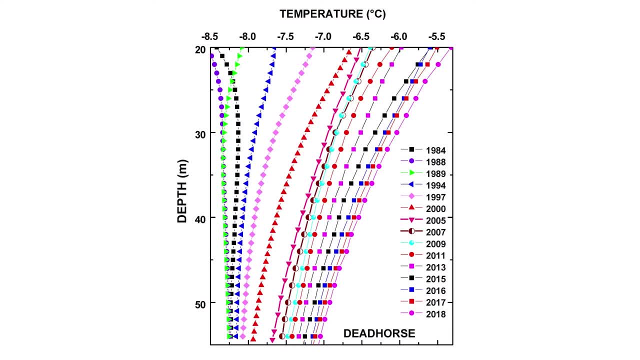 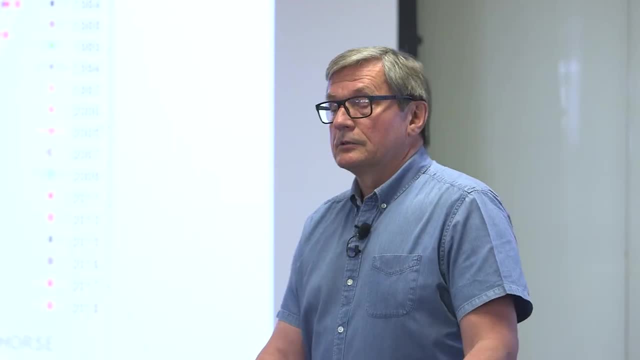 But since mid-80s it was continuously warming, and warming, and warming, And if you look at 20-meter depth, it's already by now more than 3.5 degrees Celsius increase compared to mid-80s. So which means that well, we made already at least 1.3.. 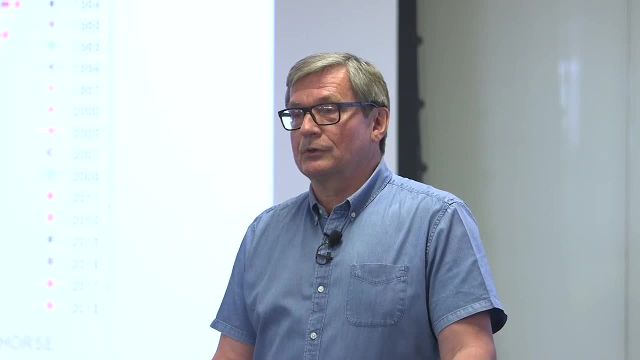 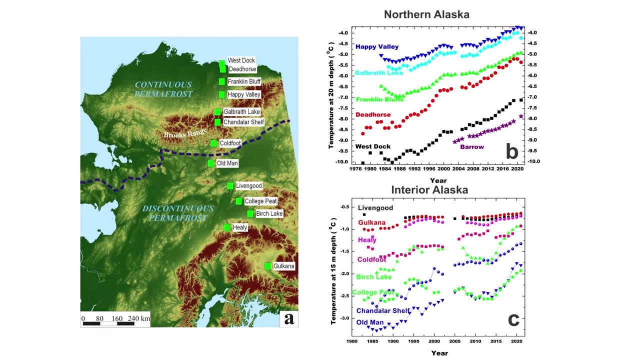 Over the way, 20 meters to that zero threshold. The same data, this is our transect and this is kind of the same data from boreholes at 20-meter depth, but as a time series. Just to see it: at one depth: 20 meters, but as a time series. 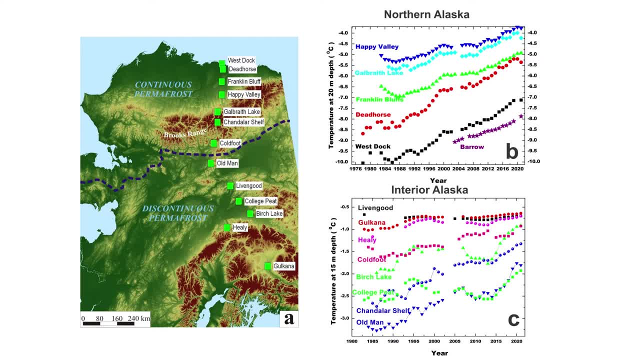 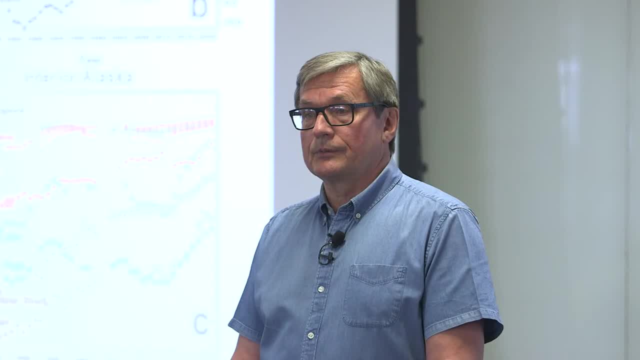 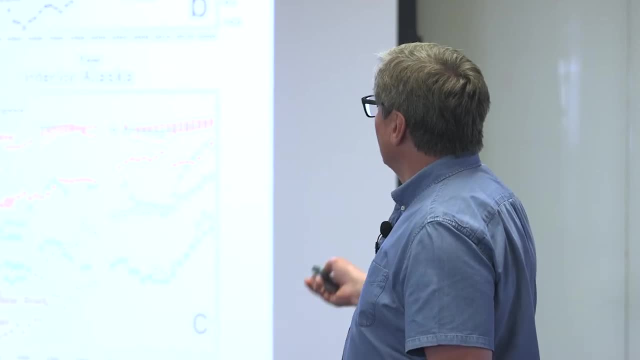 And some actually measurements started in Deadhorse and West Dock even before that. Yeah, So that's where you clearly see the increase in temperature in 20-meter depth. What we see here that in colder Promo Frost this increase is larger. In warmer Promo Frost it's a little bit lower the rate of increase. 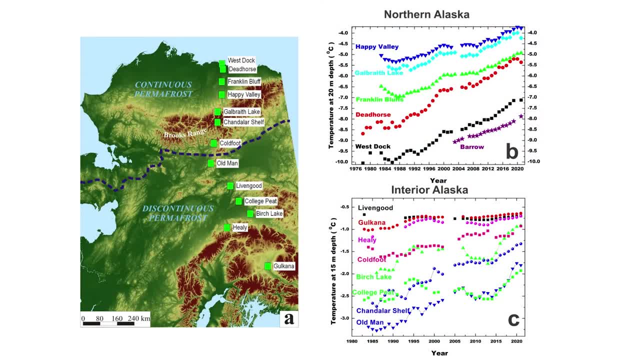 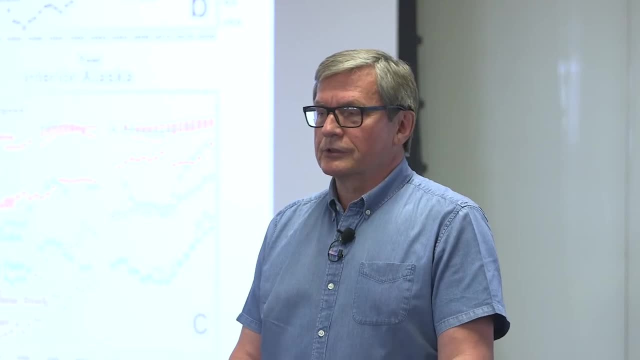 And sometimes it happen that it's not really monotonous, but sometimes it could or not increasing or even a little bit of cooling, a little bit like what we have very recently because of two consequent Consequent cold winters and cold years on the North Slope. 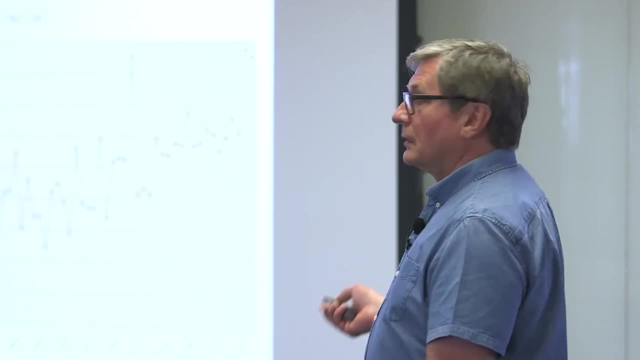 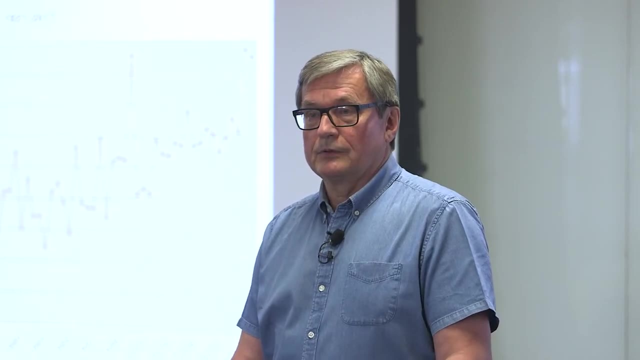 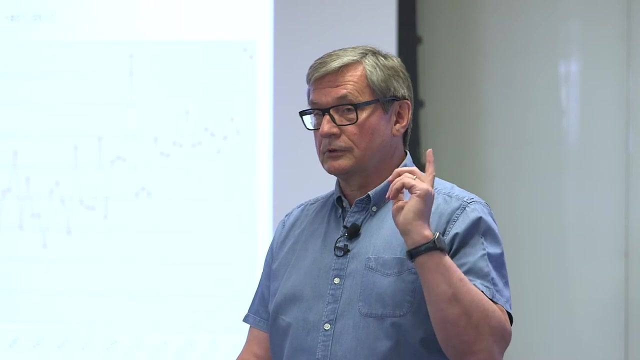 So let's see what's the explanation. So the main driving force here is still air temperature. So this is data, air temperature data from Barrow, from Barrow Meteorological Station, Actually on the first other meteorological station on the whole North Slope of Alaska. 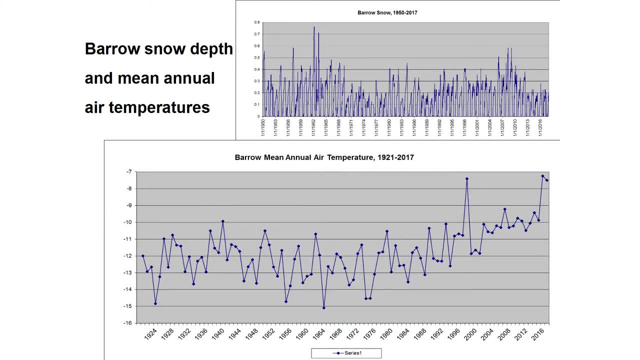 Yeah, Yeah, And you can clearly see that it was a little bit warmer in the 40s and maybe beginning of 50s, and then it was cooling. That's cooling what I was mentioning. the new ice age is coming- But since then it was very, very steady, steady increase in temperature, with some 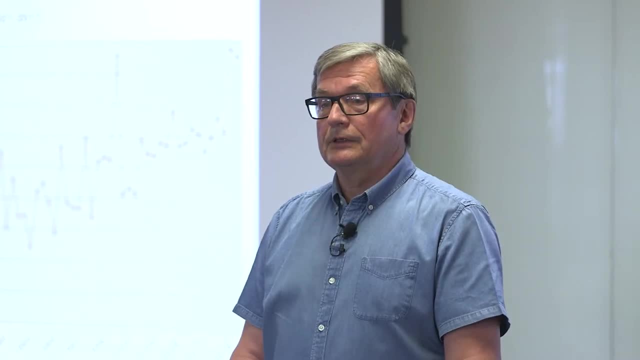 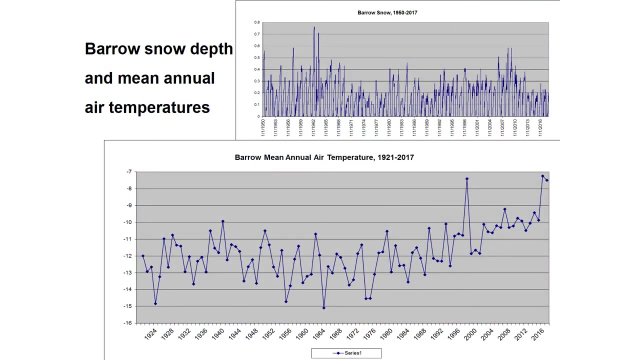 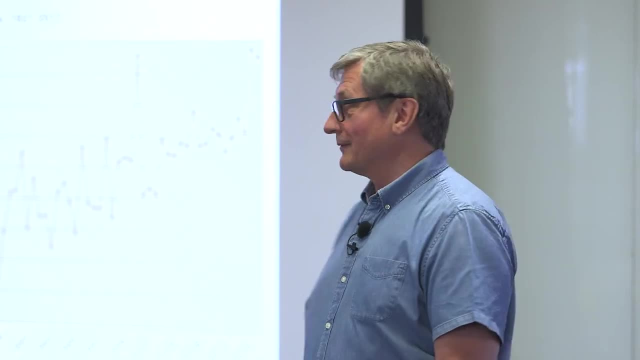 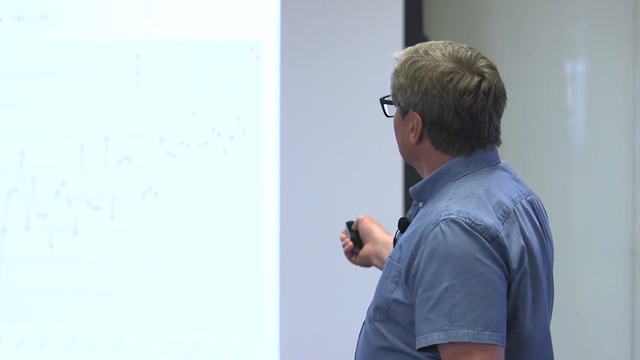 Yeah, Yeah, Yeah, Yeah, Yeah, Yes, Yes, And the temperature is about minus seven and a half for Barrow. it's definitely very warm, because typical temperature for all this period was about minus 12.. Yes, And also snow cover is another important player for permafrost, because snow protect permafrost. 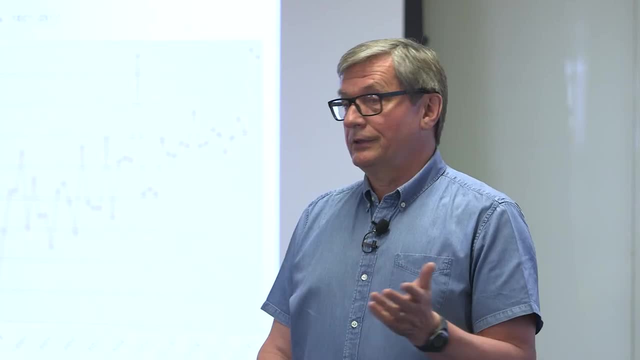 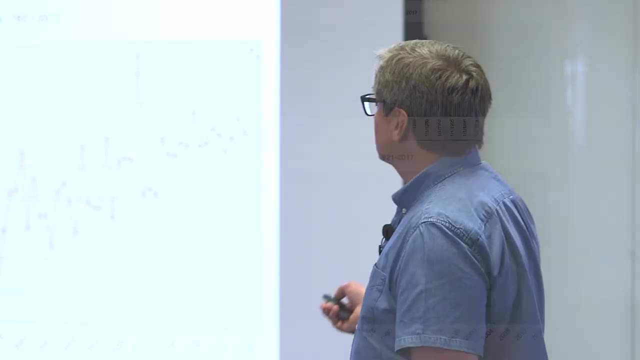 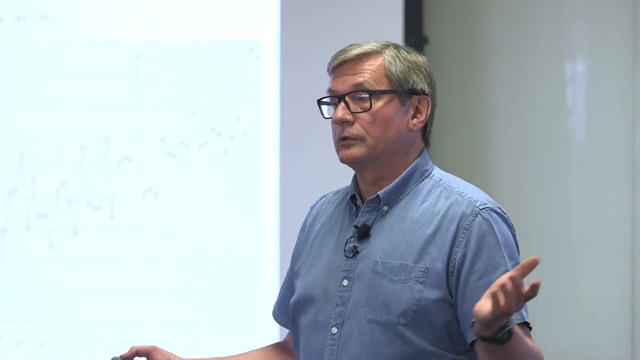 during the cold period in the winter and then during the summer is not there. So more snow, warmer temperature will be in permafrost. So you always have to look at- Yes, look at least at- these two meteorological parameters to see what should happen to permafrost. 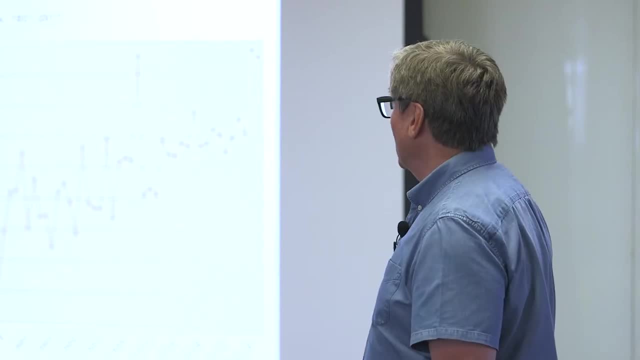 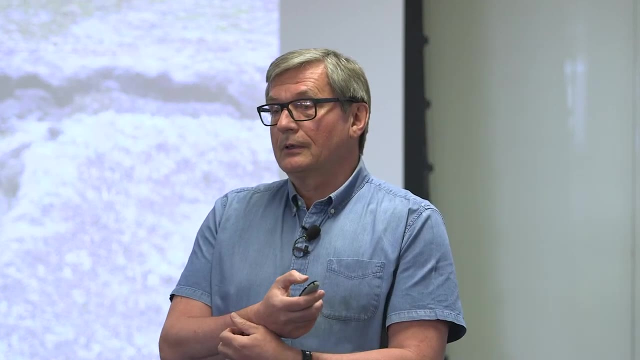 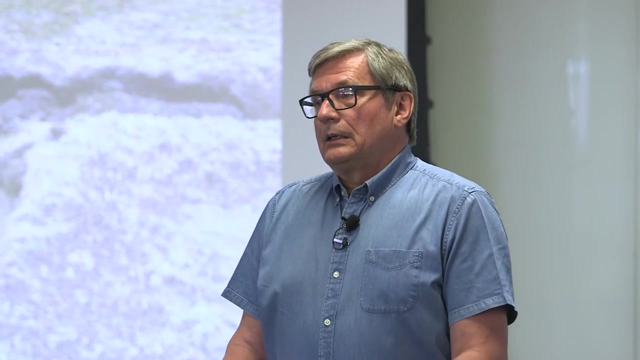 And that's the conclusion of our analyzing our data as well. Let's see. I'll skip that one Now. of course, the more exciting to see what's the result of this warming: One increase in temperature in permafrost, even if it's still more or less stable, it's. 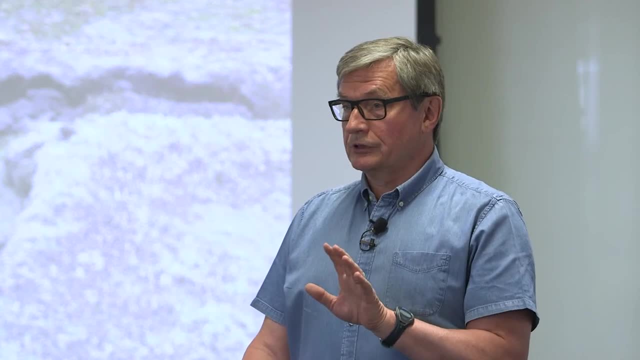 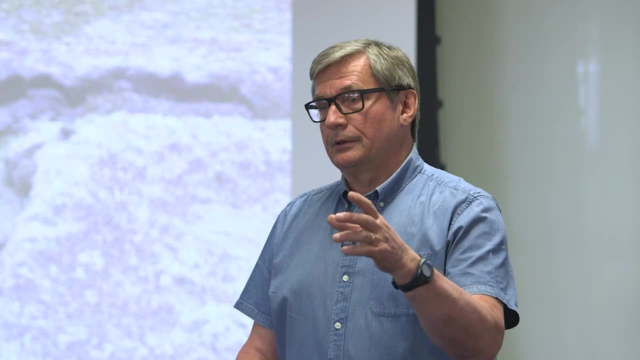 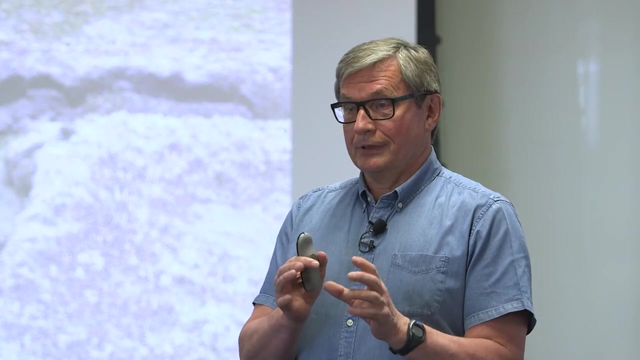 already changing its properties And in terms of engineering, it's already important because, well, if you know, that's many buildings built in permafrost region on piles, So to hold these piles in the same place, permafrost should be cold enough. 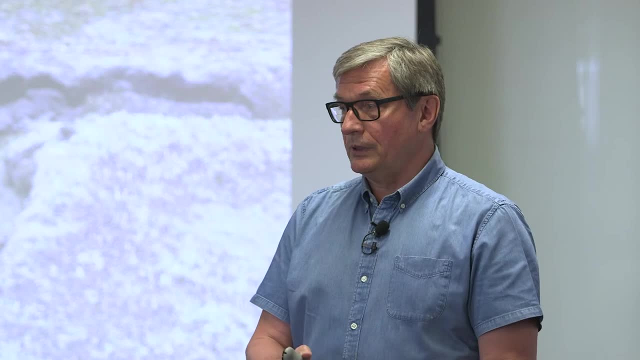 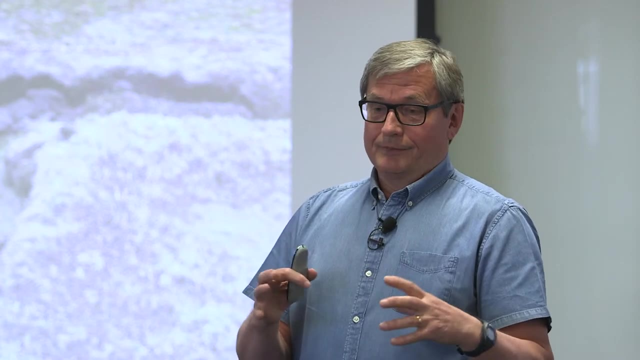 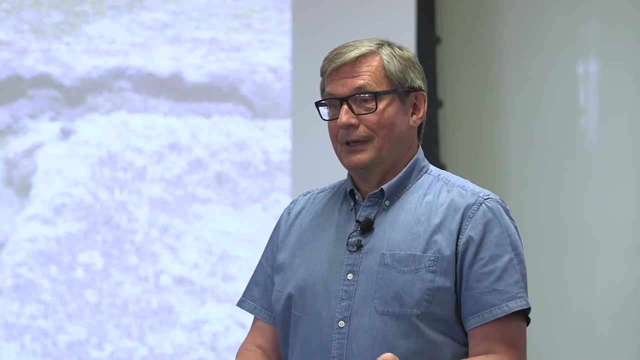 And that's how it was designed, how deep the pile should be And if permafrost temperature is increasing Like it. I just showed that this capacity of holding of the same weight is decreasing And that can make problems for infrastructure even without thawing of permafrost, just because 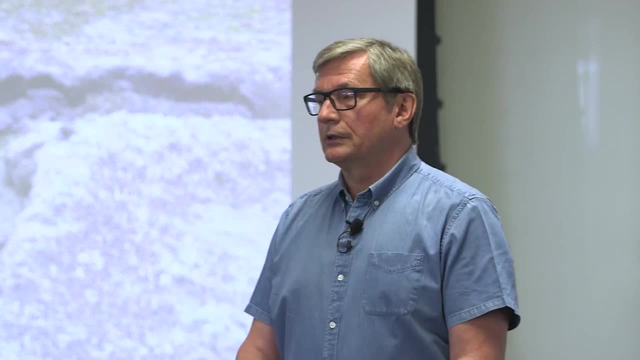 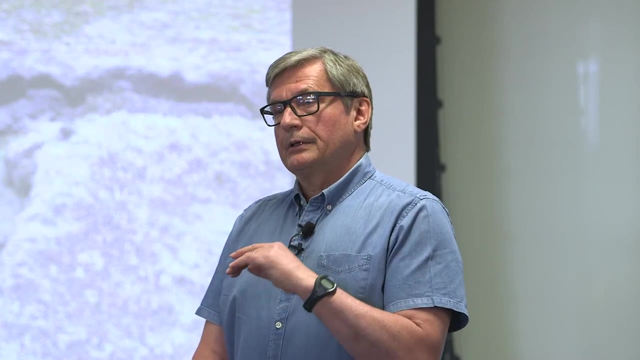 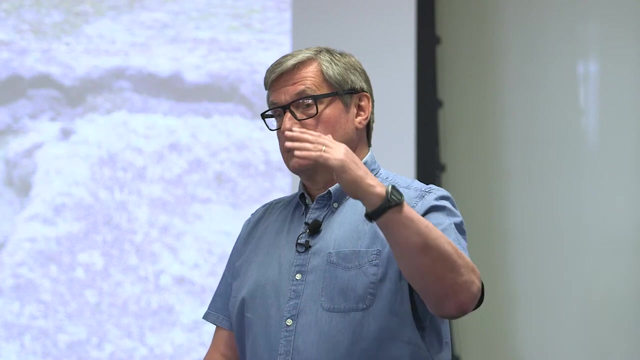 of its warmer. However, what we see also in cold, even in cold permafrost- and I will give you example- very cold permafrost that's. this warming make it not only warmer, a higher temperature in permafrost, but also increase in summer thaw depth. 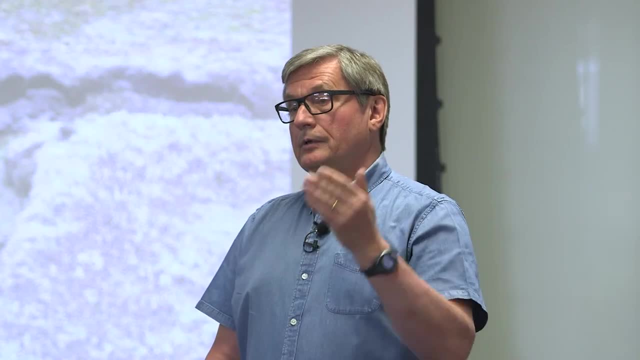 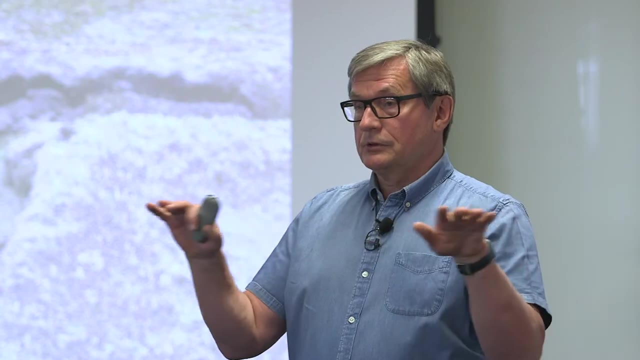 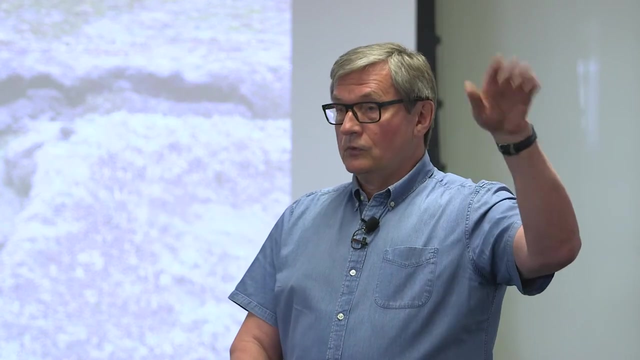 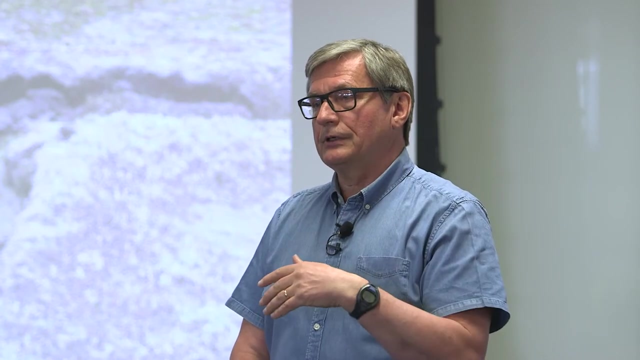 So summer, during the summer, because of warmer climate, the depth of thawing getting larger and larger And eventually remember these ice wedges, So they were sitting here, and every year, of course, and before, before this warming, active layer. so we call it active layer, the layer which thaws every summer and then refreeze. every winter was more or less, you know, the same level, say 50 centimeters. So that's why the most ice accumulated starting from 50 centimeters and down and below. Now we have deeper penetration of thaw, so upper part of ice wedges started to melt. 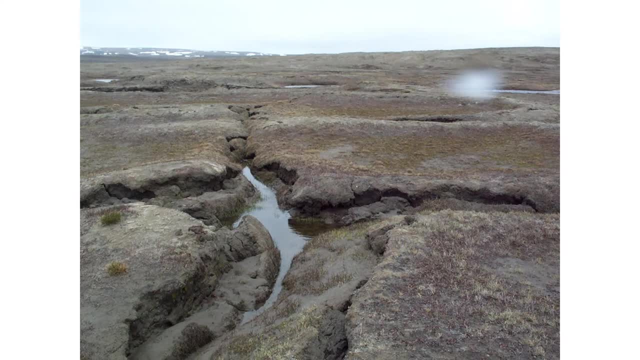 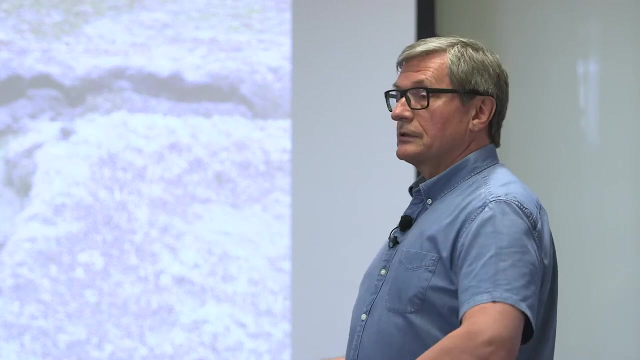 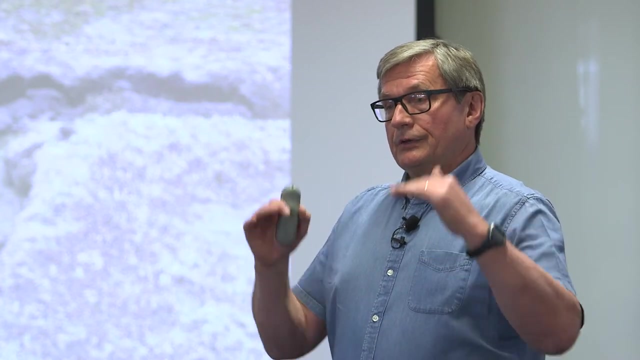 And that's very good example. this is Banks Island. actually it's even farther north, it's Mold Bay. It's in Canadian Archipelago, Where permafrost is minus 14 degrees Celsius, very cold permafrost, But because of previous, previous, during long, long time, the climate was such that 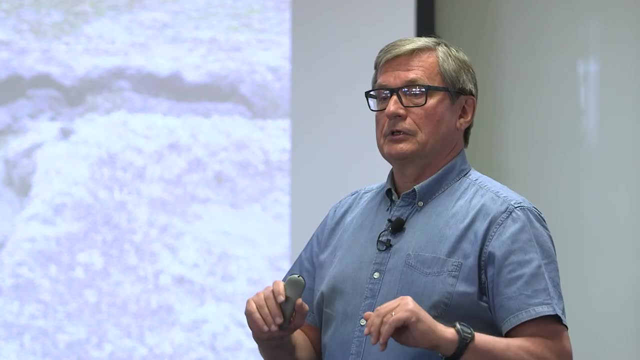 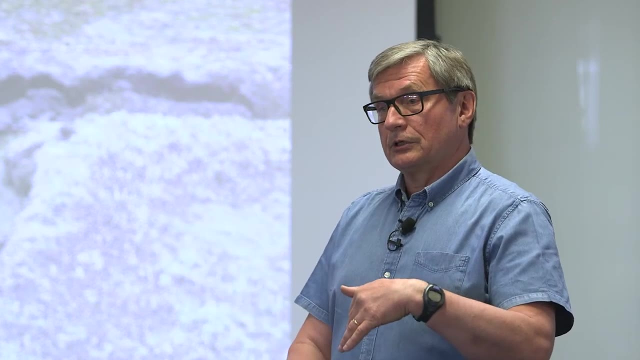 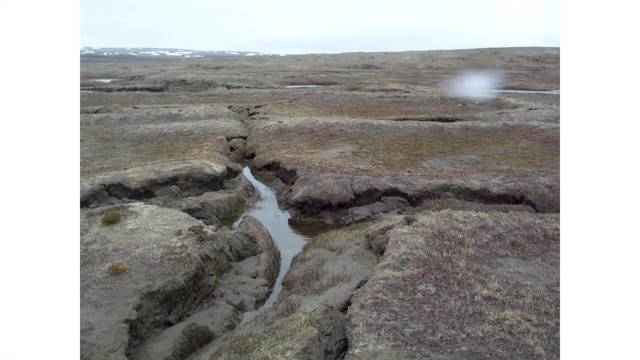 summer thaw was not penetrating deeper than, say, 50 centimeters. That's why this ice top of ice wedges was very close to the surface. And now, because of this penetration, now we start to see degradation, So degradation of thawing, melting of ice on the top and developing this kind of pictures. 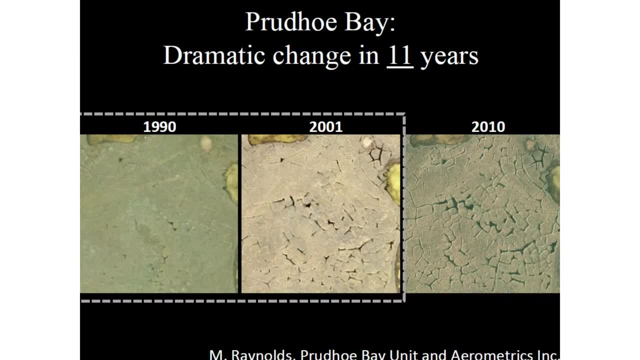 And you look from above again- and this is Prudhoe Bay area- you can see that this warming and melting of ice started pretty recently, somewhere in. actually, the first melt was described in about mid-90s, So before it was more or less stable. 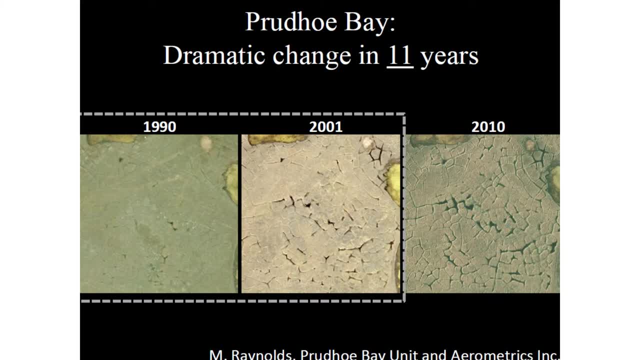 And then you compare what- it's the same exactly area, high resolution, satellite images, very high resolution- and you can see how this very nice and smooth surface with some degradation already happening- actually because it's 90s, it's not 70s- 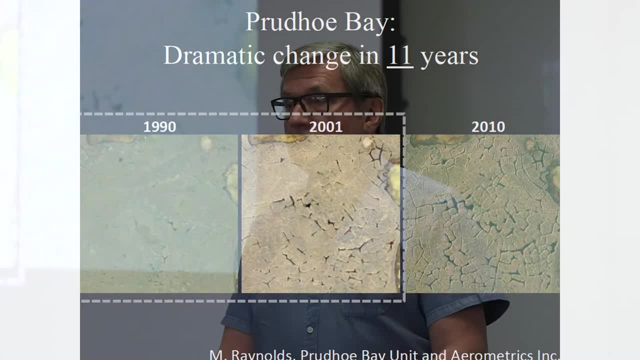 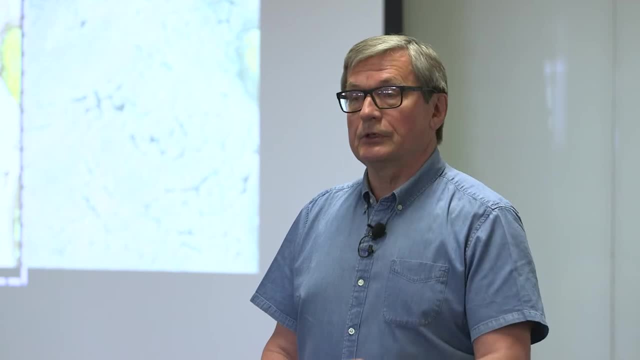 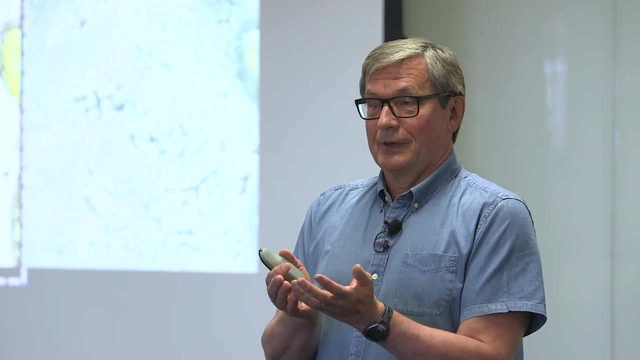 But it's progressively increasing and developing these troughs and water bodies completely changing. Well, not completely. Yes, Not yet, because it's only what we see now. it's only melting of top of the ice, wedges Only. 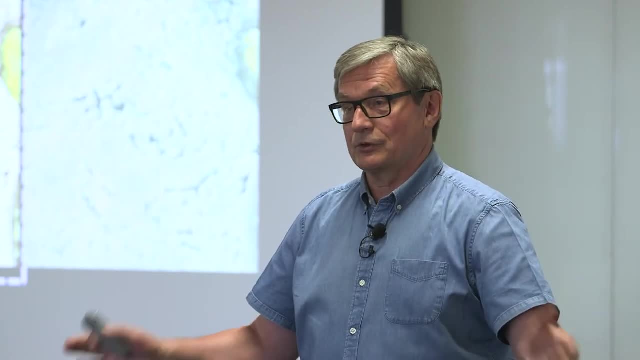 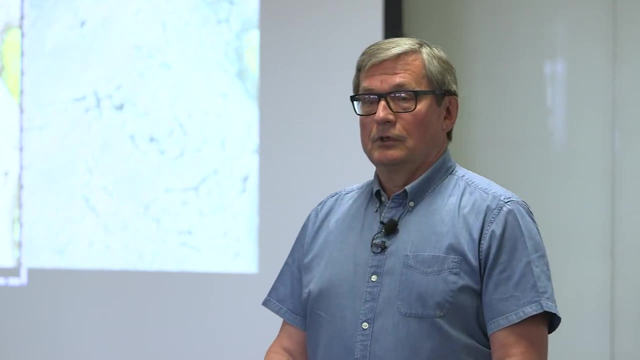 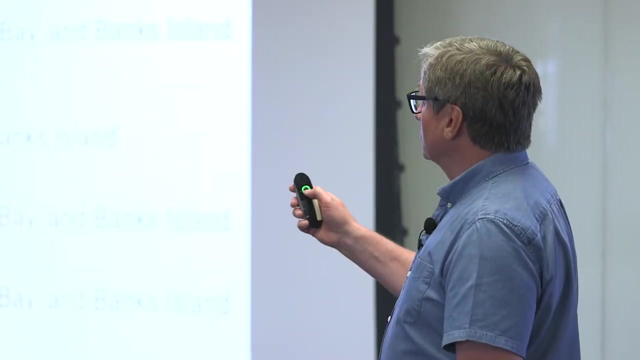 It's not, you know, degradation of permafrost everywhere, So it's just local. But even this local degradation already creates very different conditions for vegetation, for animals, for people living there, And I want to give you this example which we actually observe. 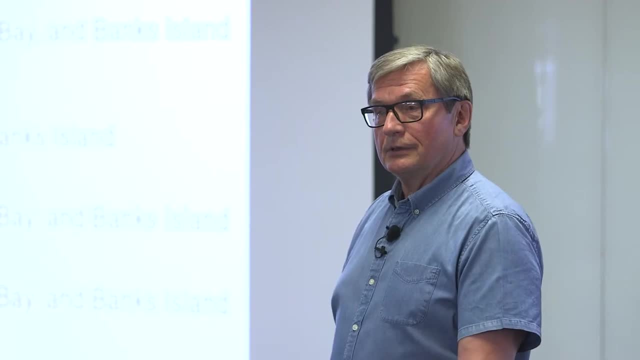 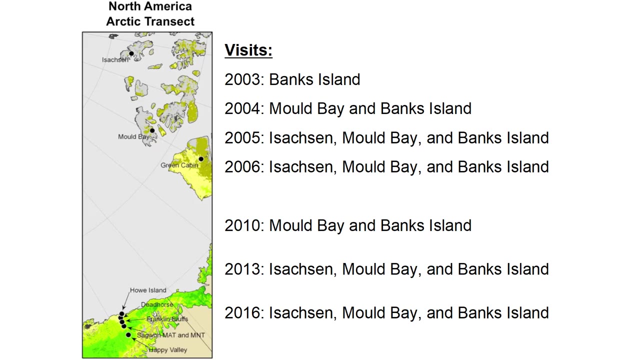 This process when it's just started in the Canadian archipelago. So we were lucky to establish these three sites. So the Prudhoe Bay is here, Banks Island and Mould Bay in Prince Patrick Island and Isaacson in Edda Fringlas Island. 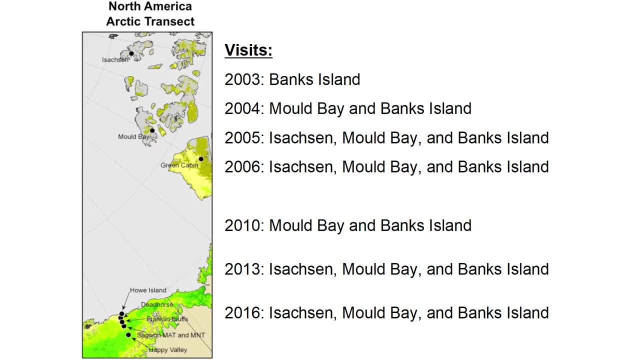 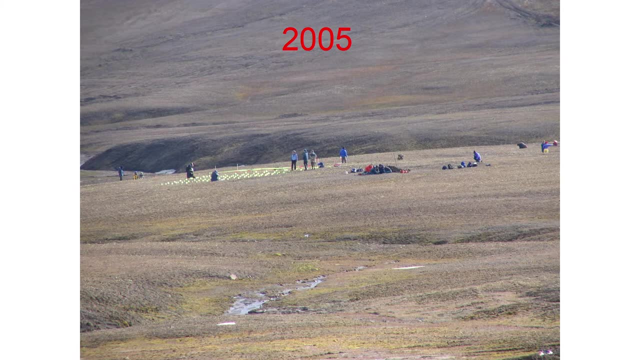 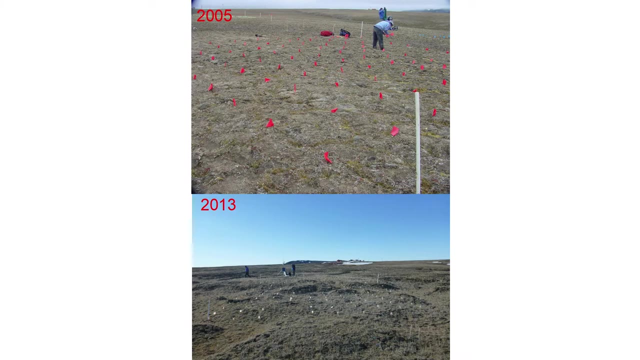 So in 2005,- this is Isaacson- the farthest north one. So that's plot said by biologists. They of course studied the whole vegetation And I was responsible for temperature measurements. So exactly the same plot here. This is the same plot, the. 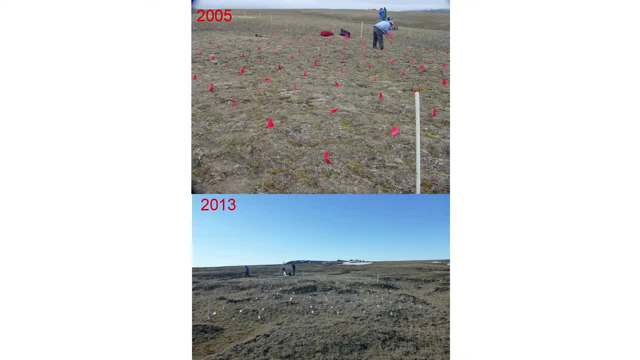 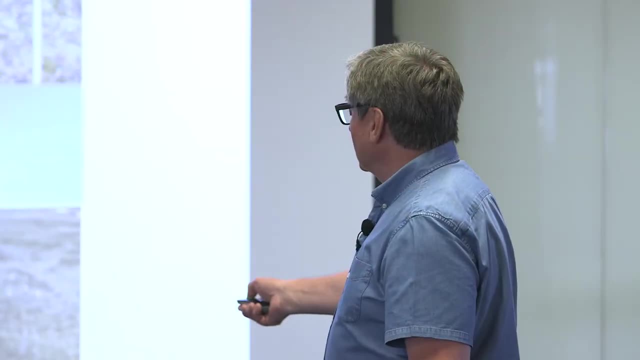 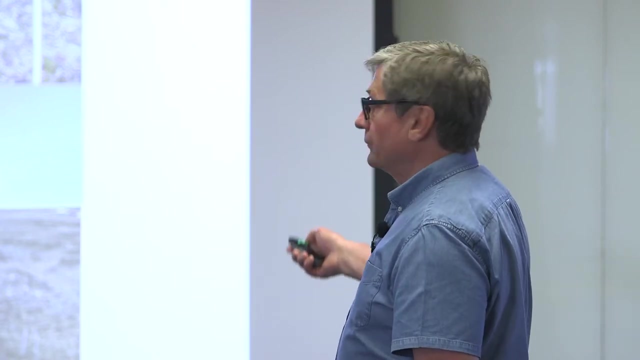 same flags. Of course, they change color because eight years changed. When we came back, when we were able to come back, eight years later, we found that surface is very, very different than it was at that time when we were there, And I will just show several of these photographs comparing what it was then. we established. 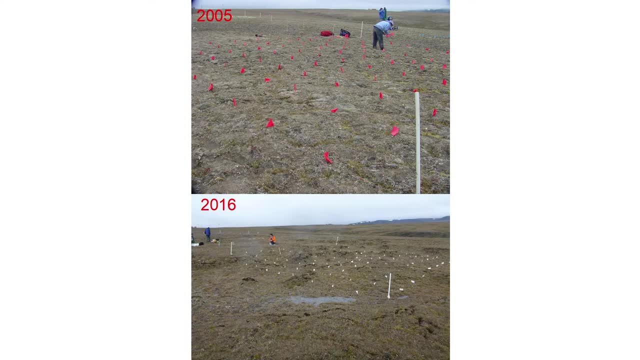 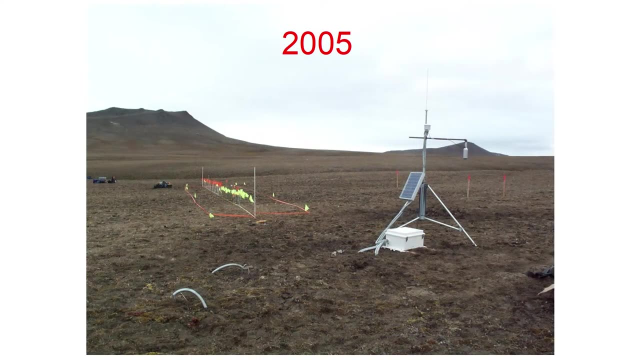 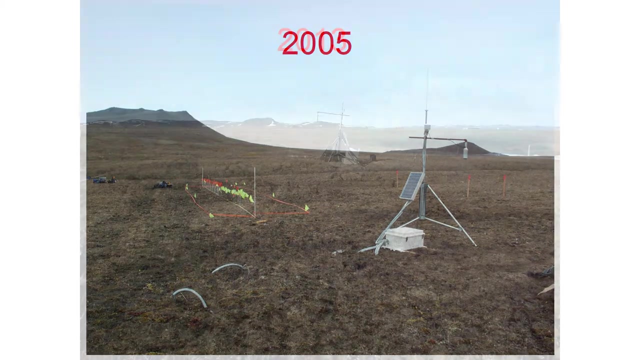 Then we revisited in the 60s and it gets even worse. There's still water start to accumulate. This is the set with my station, with ground temperature measurements, And actually it could be, Yeah, So it was like this: very, very smooth and nothing particular. Well, what happened? 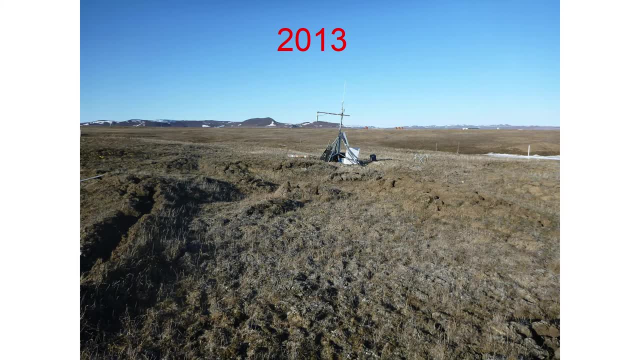 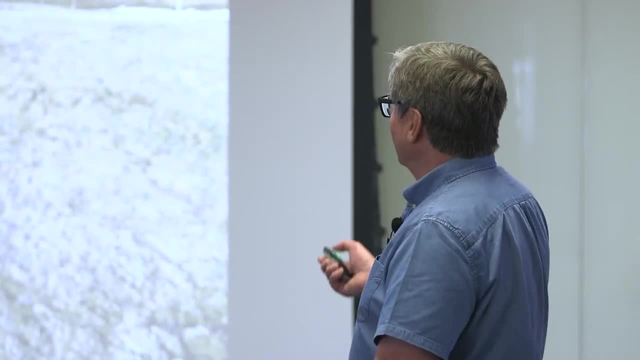 we actually put it very close to the ice wedge. Well, we didn't know even, because there was no indication there was any kind of ice wedges there. Well, and we were very worried when we put it that polar bears can destroy the station. 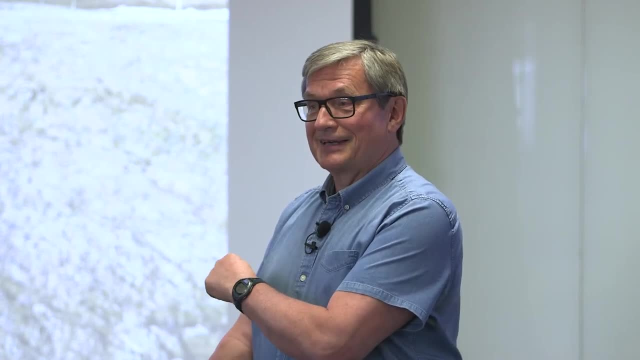 Well, no problem with polar bears, but problem with degrading thermoproces and ice wedges. It was little more than that. Yes, First of all, right, we needed to try to avoid the ice wedge because it – I am. 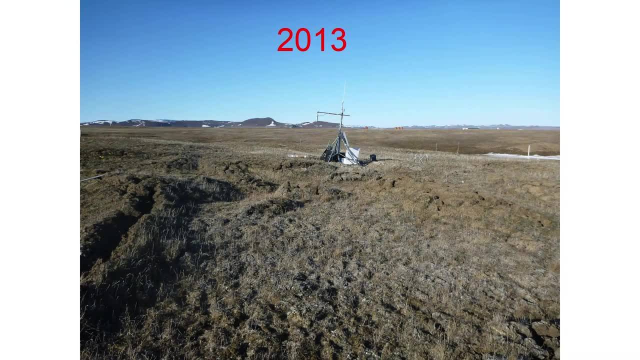 very sure of the portion of the ice that is, fortunately vertical to the side and almost horizontal. Let's see, This might be the longest ice wedge that was comb neurologically down from the ground. all right, I was actually trying to avoid climbing and sometimes try to sit on it. 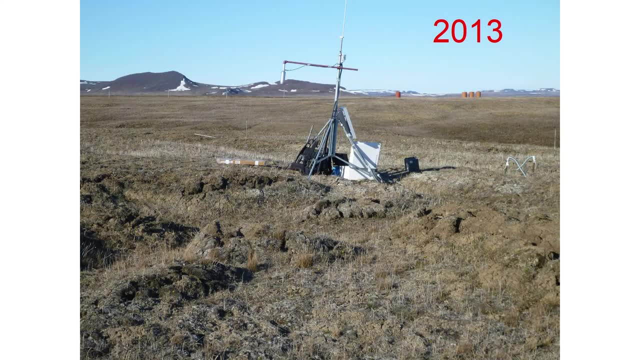 Hopefully it could, but it would ruin Because it start to kind of See it's already leaning on one side And eventually- this farther development- It actually could fall down. So very, very, very rough, rough, even surfaces. 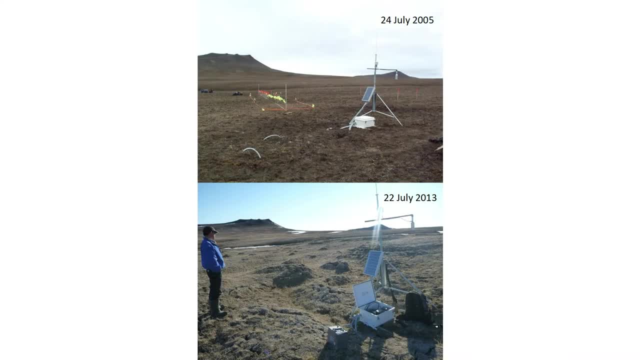 And this is, I think, very good because it's The picture was – I specilicly tried to take picture from the same position. So that's because the picture was. I specifically tried to take picture from the same position. 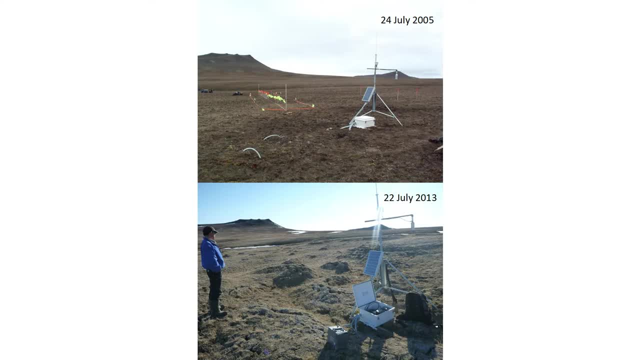 So that's two hills there on the horizon. Kenji Yoshikawa- I don't know, you may not have heard about him- was in the 13. And that's the difference. so very, very obvious, big, big difference. 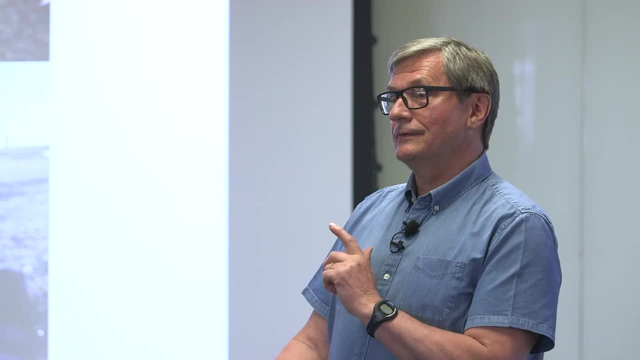 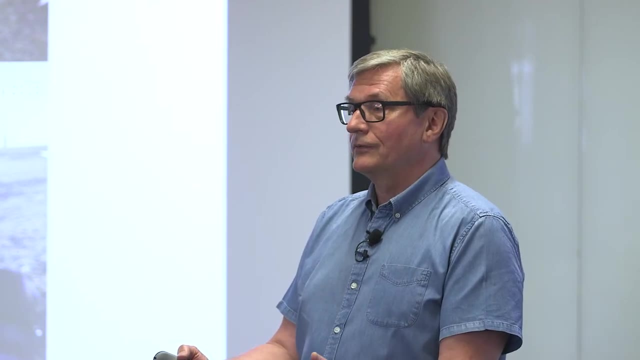 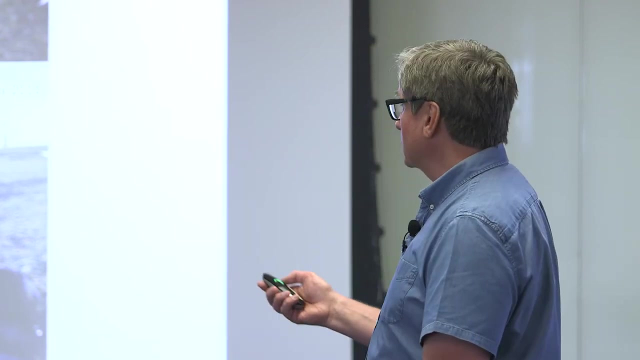 Again, permafrost temperature is minus 15, here minus 15.. So it's nothing. permafrost itself is very stable, But because of just the beginning of increase in summer thaw start to melt ice wedges and developing this kind of surfaces. 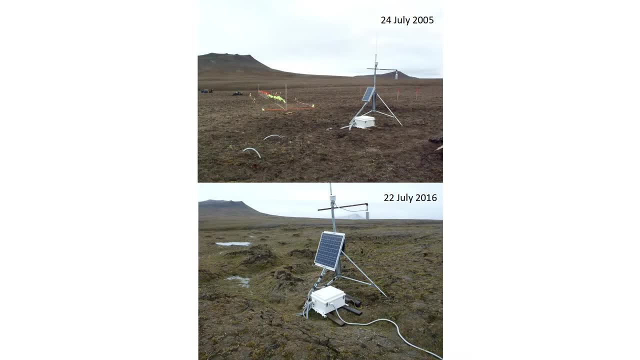 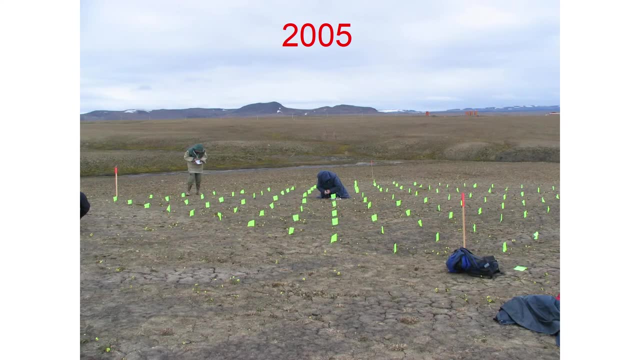 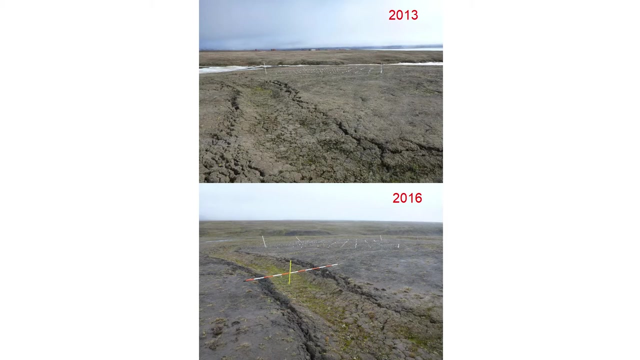 16, even more, Yeah, and see, our tower is kind of tilting. Another one in dry place actually survived a little bit better itself the plot, But big, big trough developed next to it And in this about 11 years between this beginning. 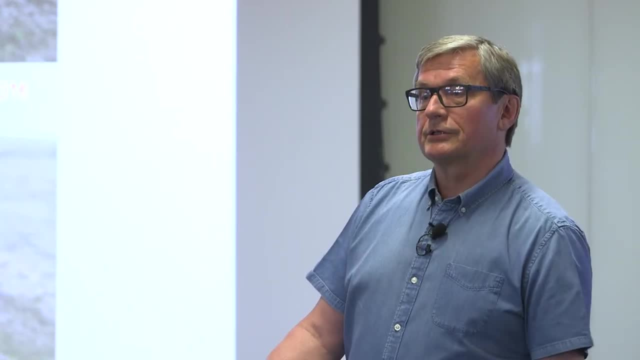 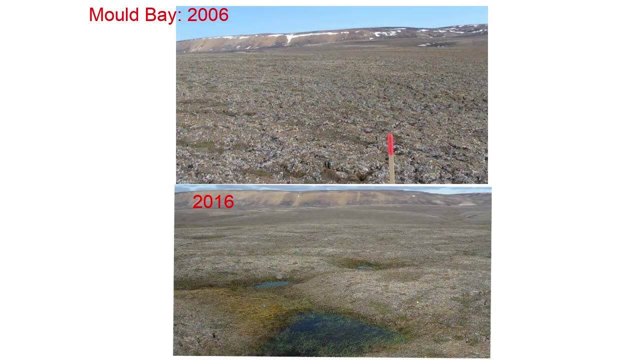 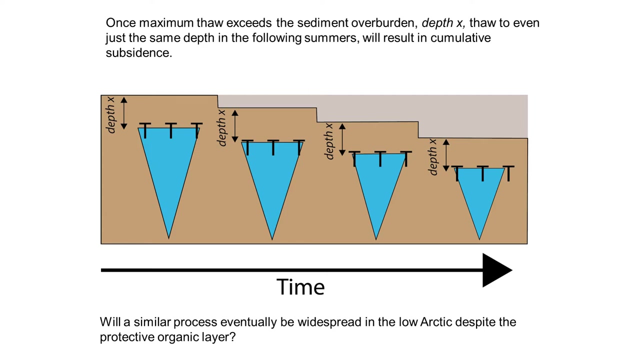 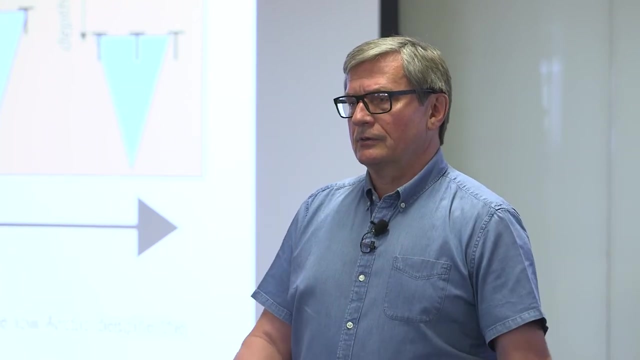 and now about maybe two feet of depression developed And the same on other sides. I will just skip that And explanation for that. you can say well how much of the thaw increase It's like if you, If you have 60 or 80 centimeters of depression. how it could happen. You cannot get this amount of thaw or melt of ice just because of warmer climate. So the problem is it's not only warmer climate, but also the surface is also subsiding And the distance between ice wedge and surface. 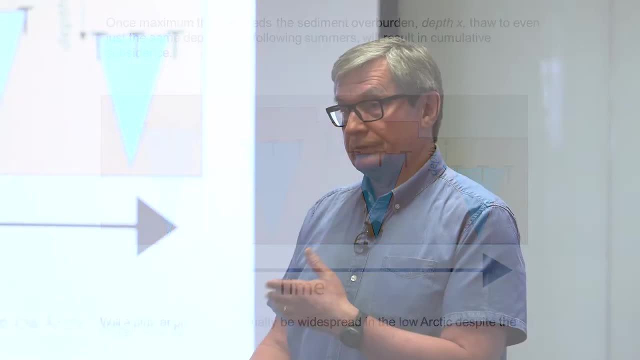 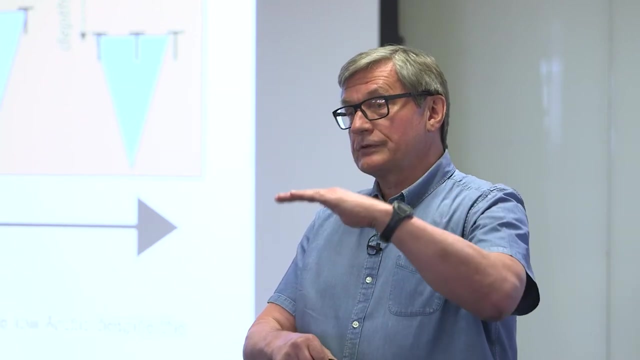 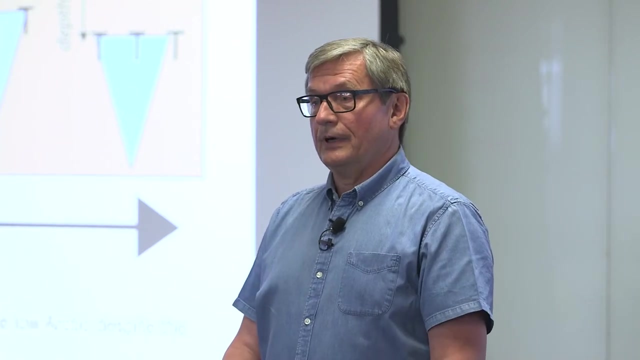 is more or less the same, Because melting ice wedge produce water. water drains because it's kind of slow. It's a sloping area And surface actually following the surface of ice wedge. That's why you can get so much of melt of ice in 10 years. 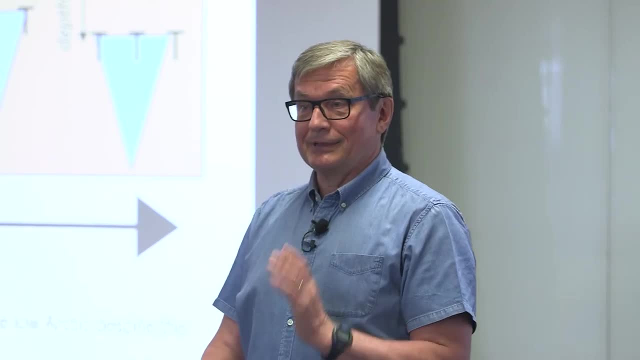 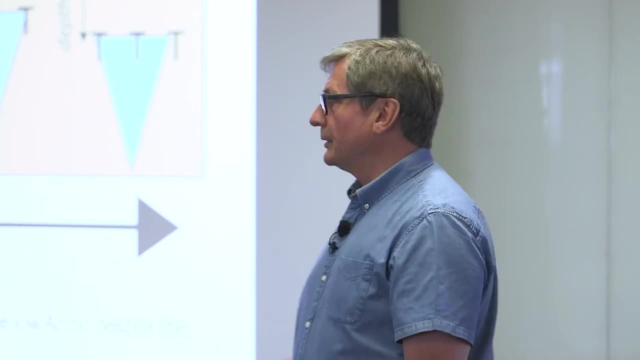 up to 80 centimeters, which is for permafrost. it's a lot Because permafrost in general very, very kind of conservative, a very inertial feature. But that could happen And that's our explanation. 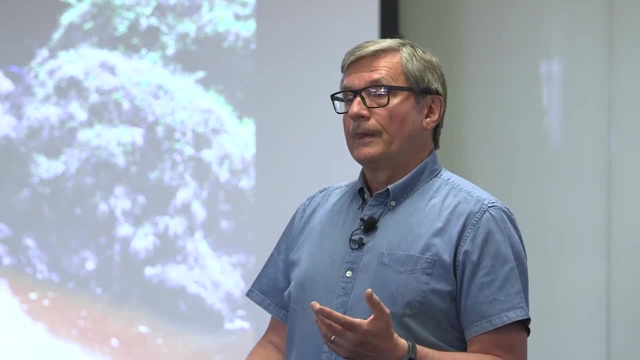 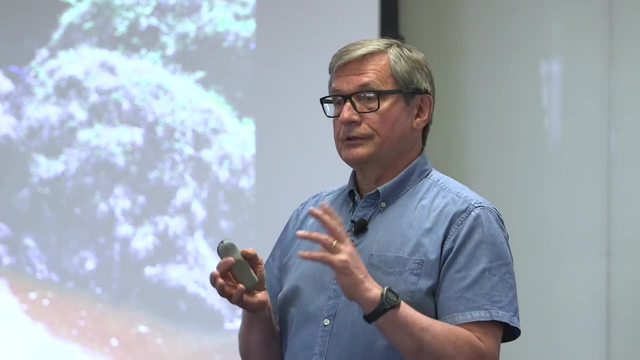 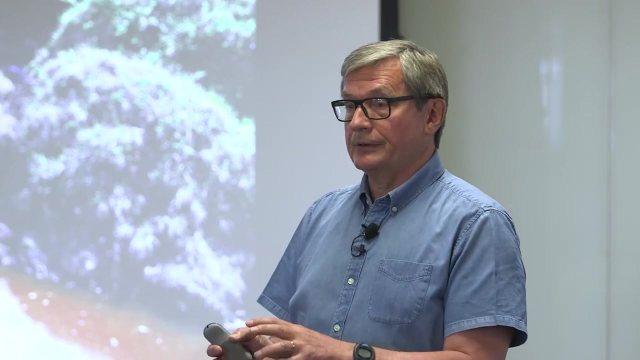 It's also because of this depression. they can trigger not only settlement because of thawing, but also erosion. We call it thermal erosion Because it's not just water taking particles, but first material thaws and ice melts and then water takes it away. 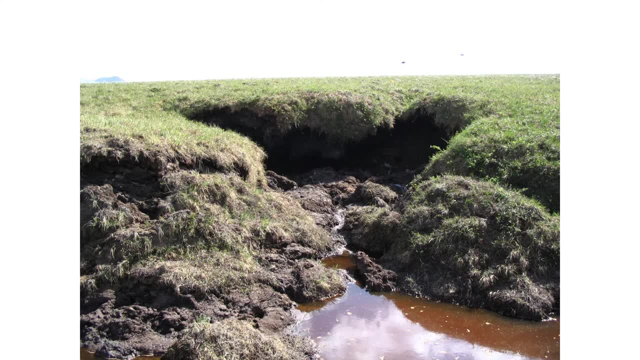 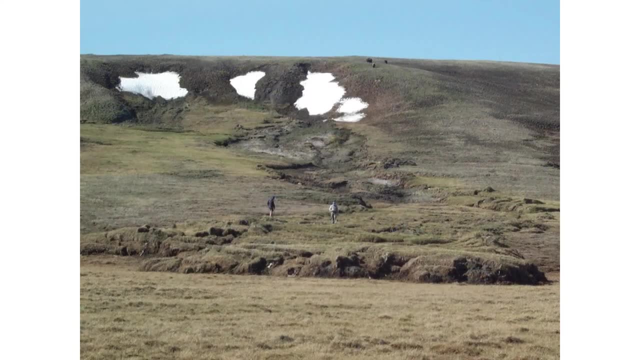 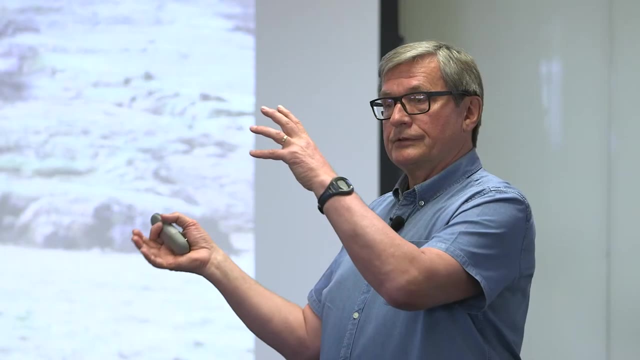 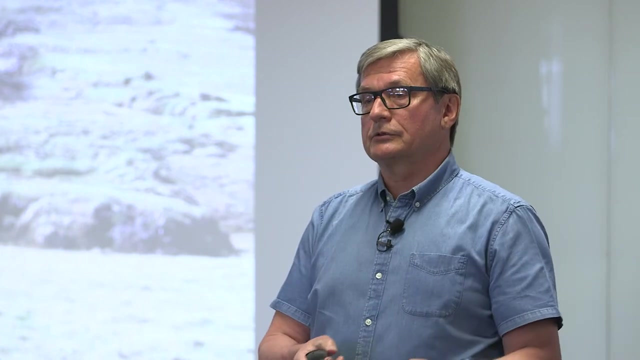 So erosion very, very common, that erosion triggered by this settlement, because of melting ice. Also, some slow processes Like this, this kind of slide, which whole upper, say, 50 centimeters of ground, together with organic layer on top, just move down the slope. 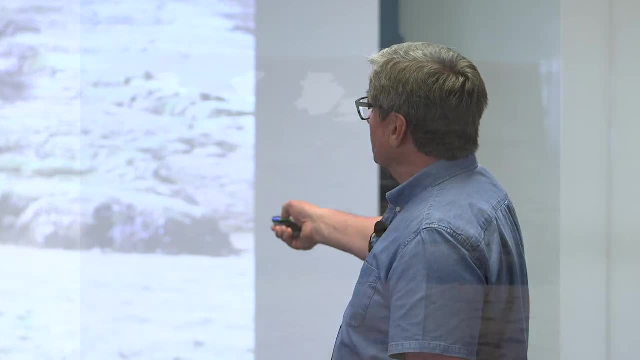 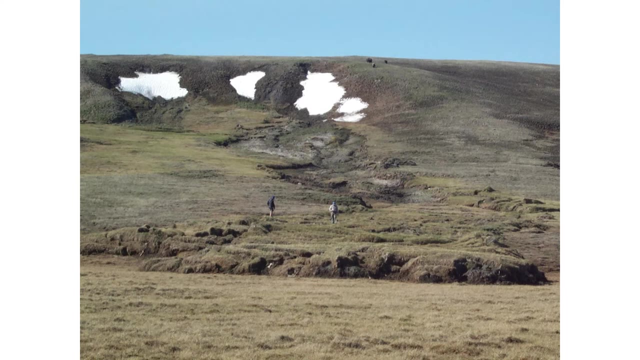 Very, very common right now- And exposing permafrost. And if permafrost is very icy, then you and I will show some examples- develop this retrogressive thaw slumps, so-called thaw slumps. Just a couple more. 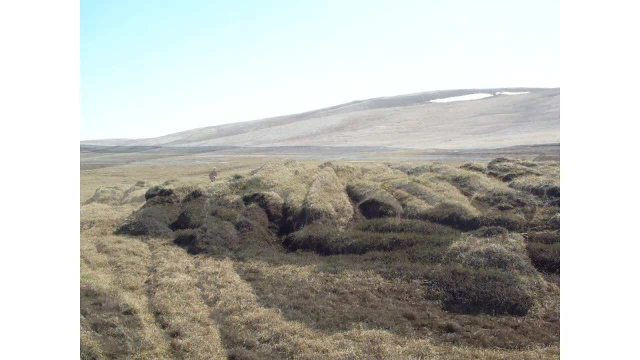 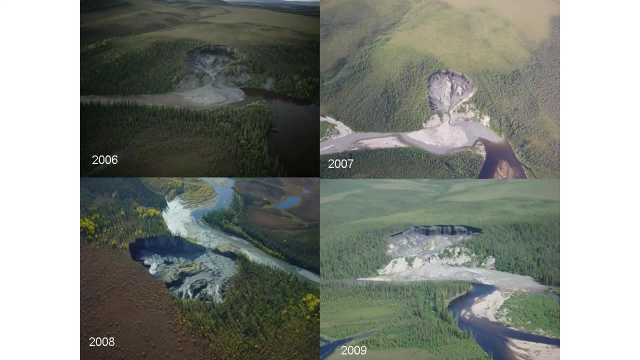 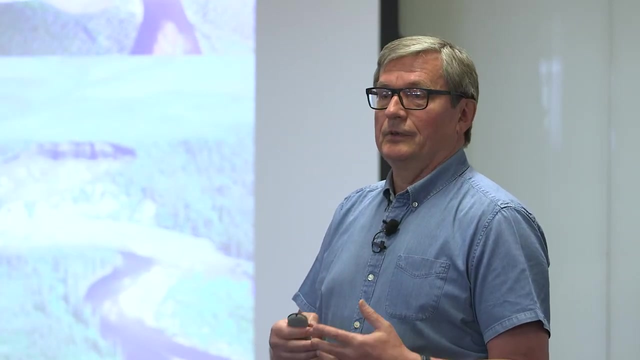 Pictures how it look like Like this, like carpet. That's retrogressive thaw slumps. When it happened first and then the ice was so much ice in it And when it melts because it's exposed, it melts fast. 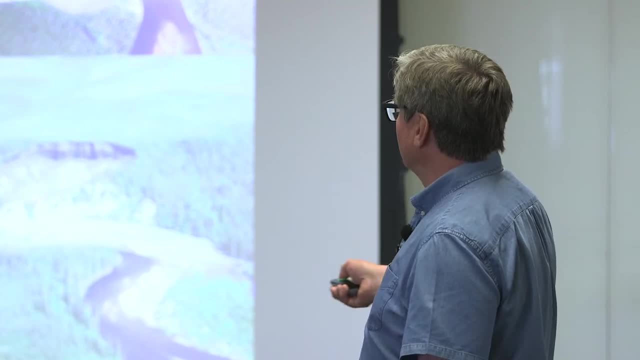 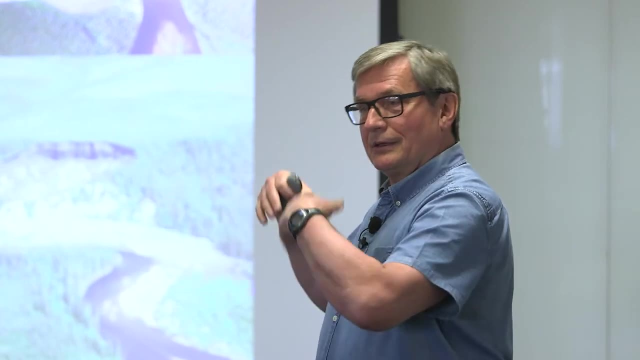 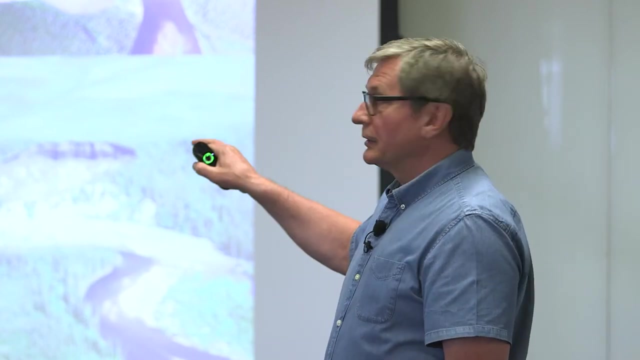 And the wall of this slump going towards the bottom, the intact area, and involve more and more and more and more in this process. And it will go all the way like this until the ice it will go, some area where less ice in permafrost. 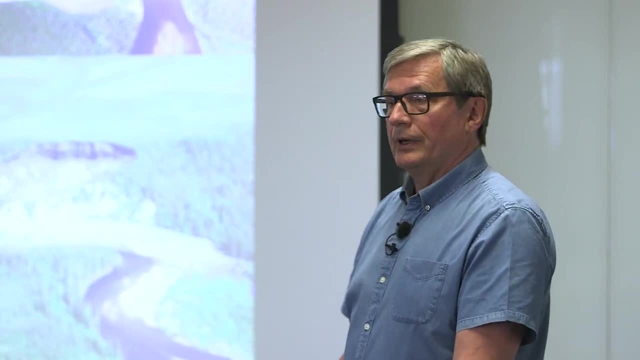 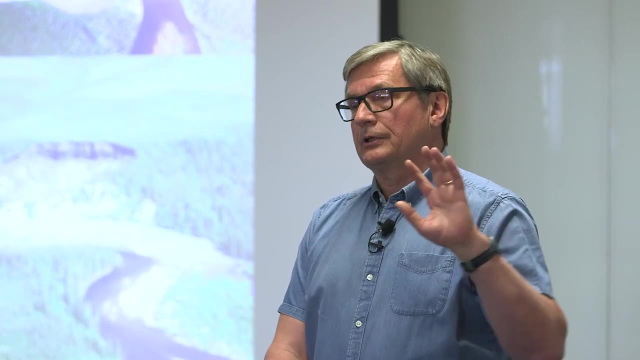 And then it may stabilize and stay. But this is very, very common process Again during the last 20 years. those kind of thing happened in the past as well, but they were kind of one and another one there and there. Now they come together. 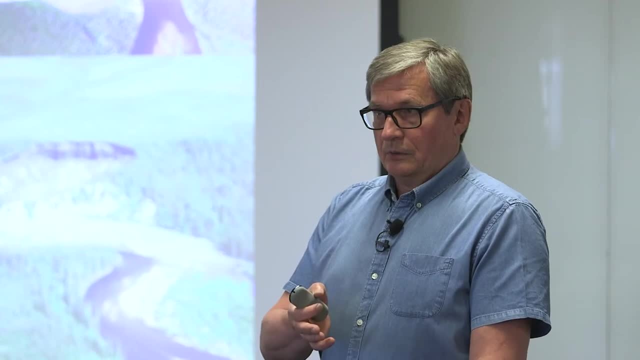 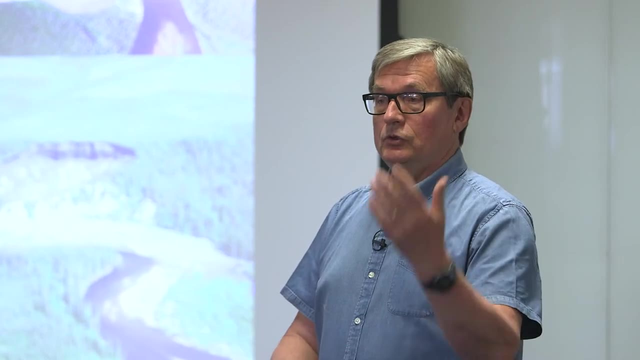 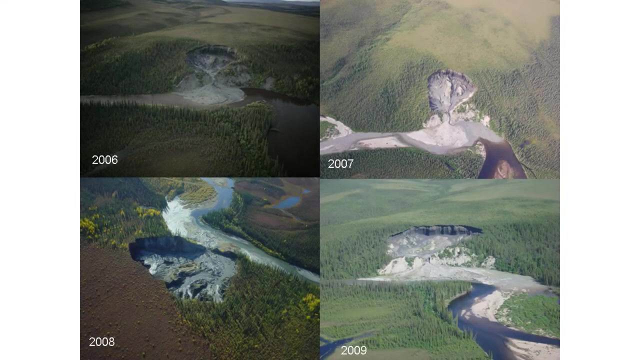 Count in this area, actually in North Slope and Canadian archipelago, by I don't know by many tons of them appeared And actually new appear almost every year, Definitely changing locally, but changing environment very, very significantly, landscape very significantly. 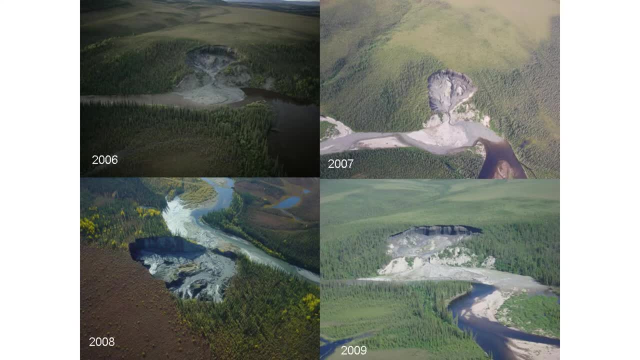 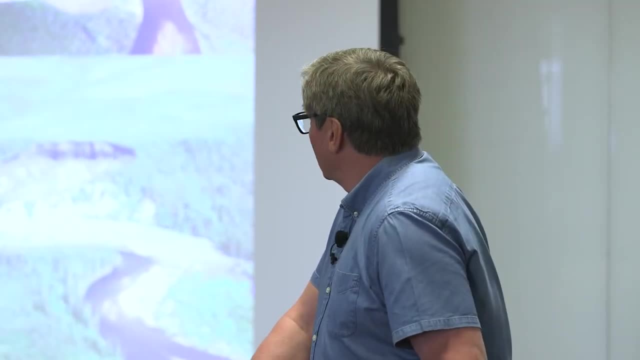 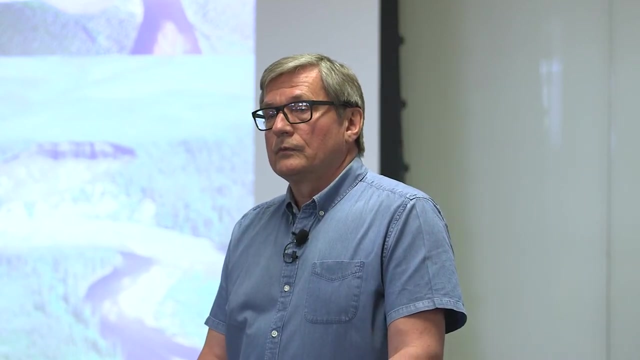 And, of course, some other negative consequences. is this silt goes into water, It's affect fish. This is actually. it's a Selawik River and Selawik slump on this photo. So yeah, it's very good fish there, white fish mostly. 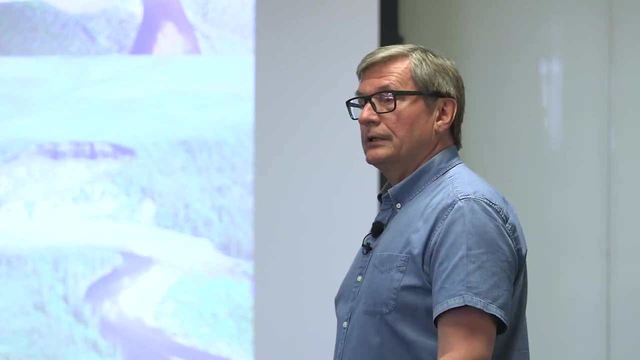 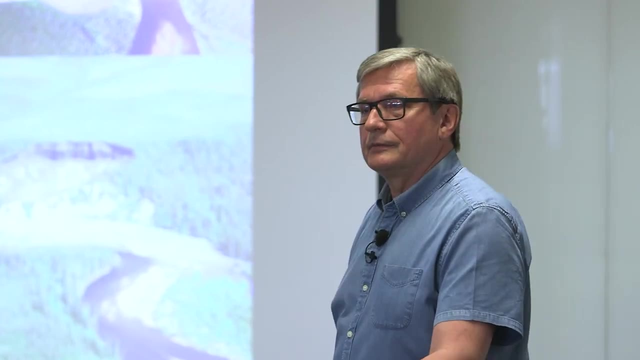 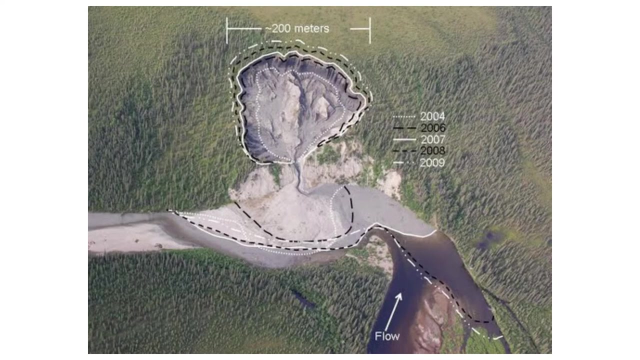 and some other she-fish, I think, And definitely it will affect some, I would say, people fishing- how much fish they can get because of the changes in conditions. Yeah, That's it. That's the development in time. 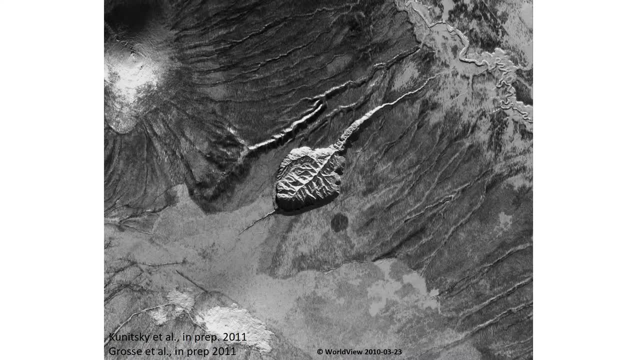 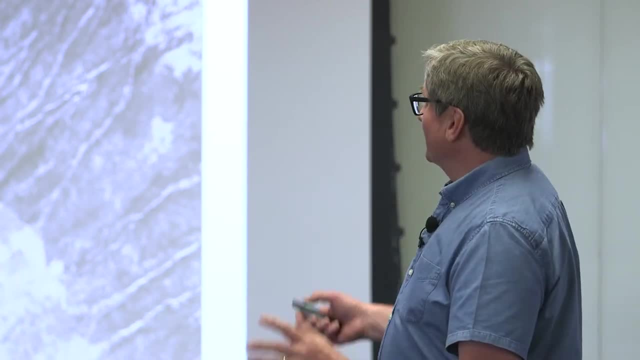 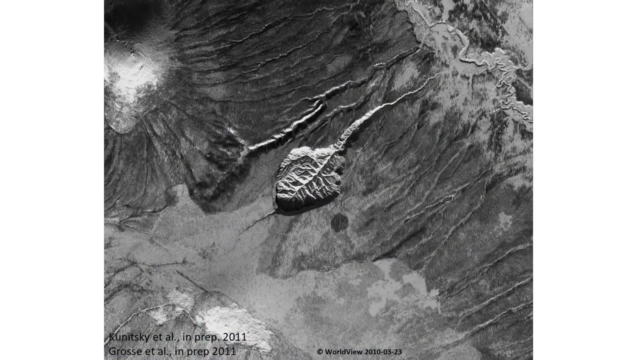 This one. there's many, many of them, So I just want to show the last one: a mega slump, mega slump in Siberia. of course, Everything is mega in Russia, yeah. So this is the satellite image of this huge slump. 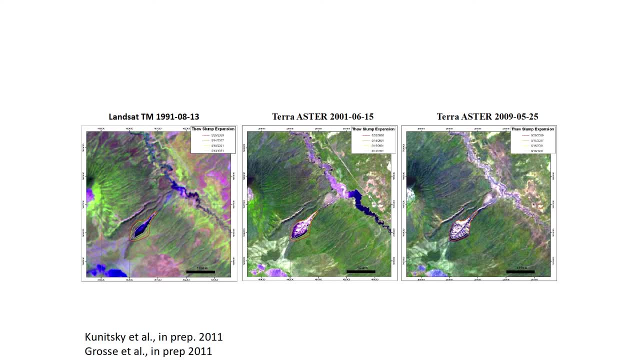 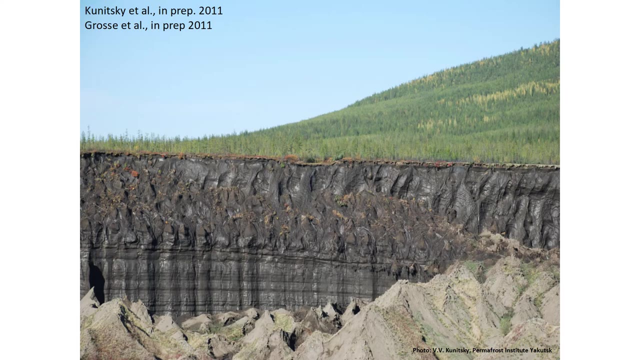 which developed again during Starting somewhere in the late 80s and beginning of 90s, And it was first it was small and then increased And now it looks like this. So this is trees. It's a large tree, but it's kind of what you have. 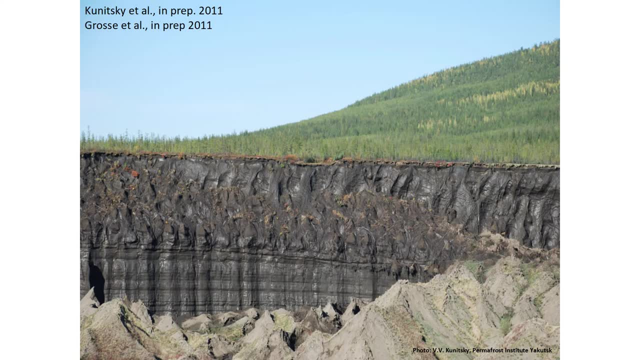 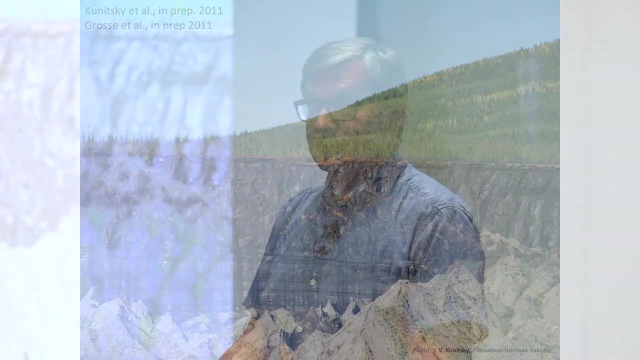 black spruce kind of analogy in this case. So it's at least five meters maybe more tall the tree And that's the slump. I mean the volume of material was removed because mostly it was ice again. 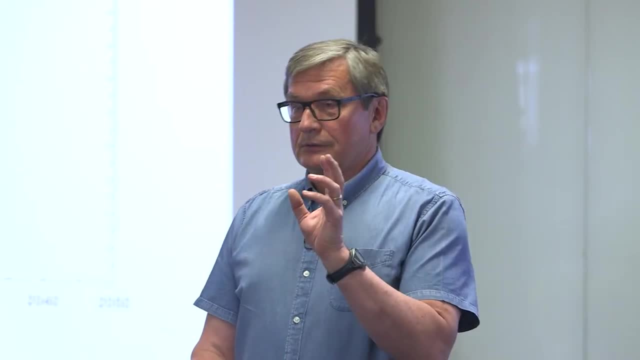 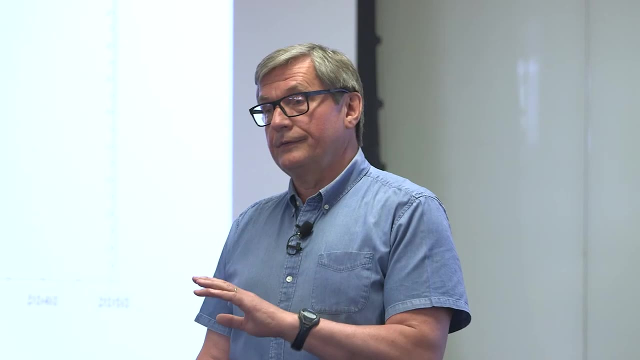 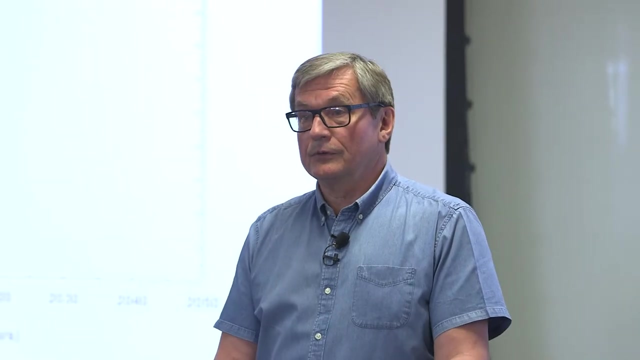 Now it's still dramatic, Dramatic, but it's still local. It's still local, locally happening because of one or another thing, because of degradation of ice, wages or development of this retrogressive thaw slumps. Well, much worse situation will be when 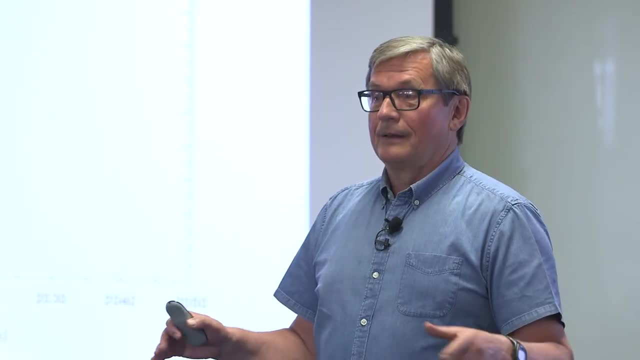 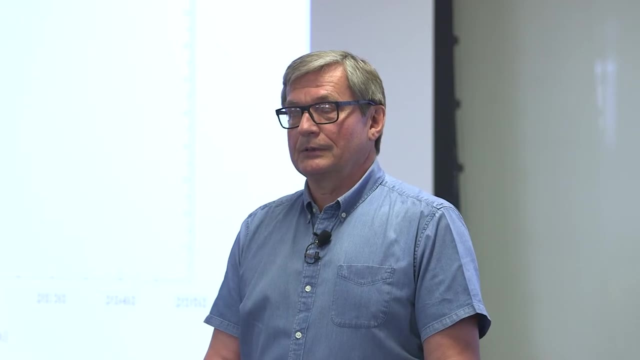 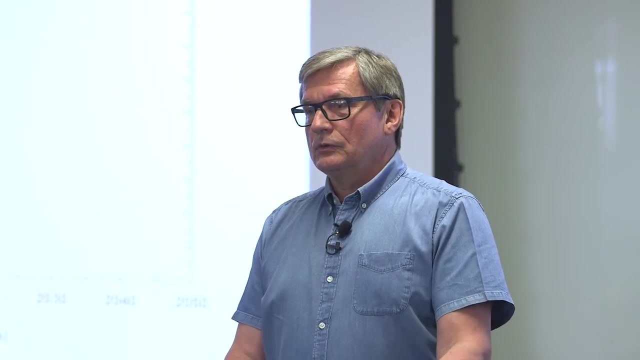 permafrost will start to thaw everywhere, So not just in some particular place, but pretty much everywhere. So in this case we have to expect much more serious consequences for landscape change. So now, what is how? when it will happen? 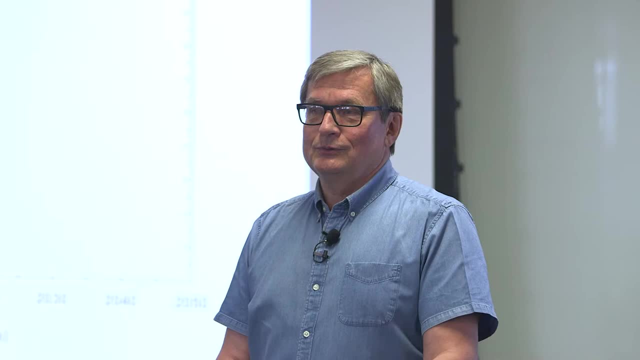 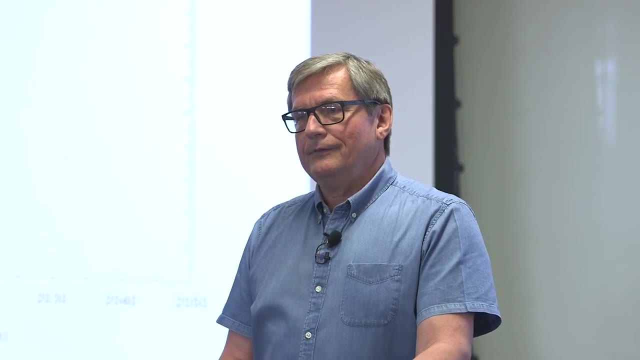 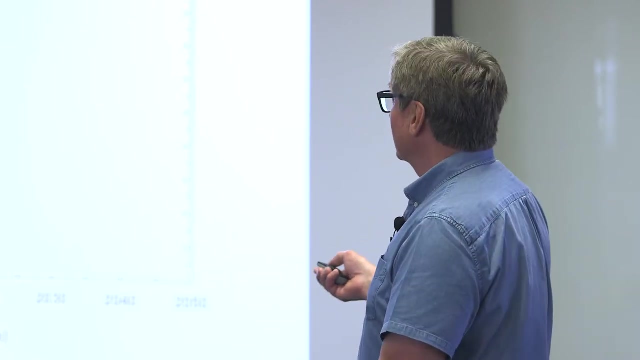 Good question, right? Well, we have enough data now to do some very simple, simple estimate, And it's very, very simple. So we have this already and I will show an example of Dead Horse location. What we see here is mean annual temperature of air air. 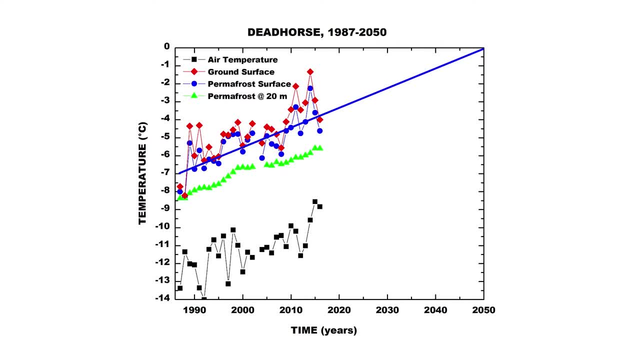 temperature mean annual since mid-80s, when the latest warming actually started, on the North Slope mostly. And also we measure, like I said, the ground surface and permafrost: surface and permafrost in 20 meter depth. So that's what we see here. Surface, red permafrost. 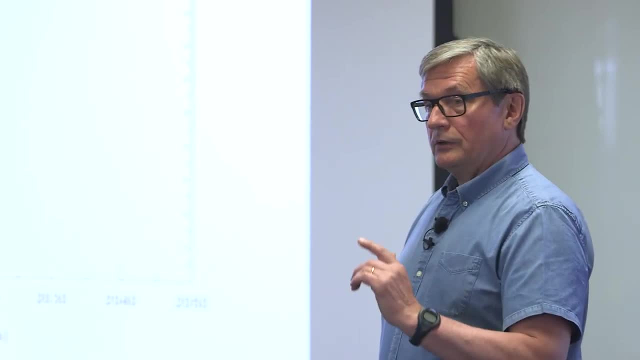 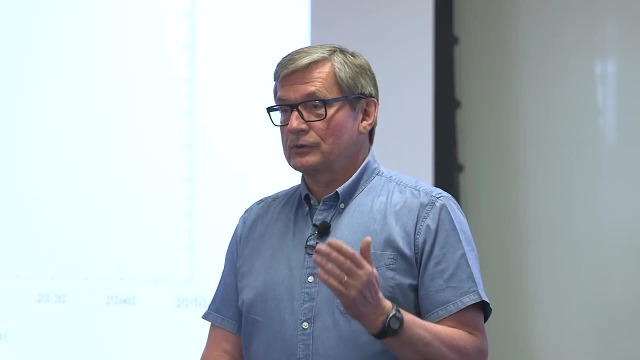 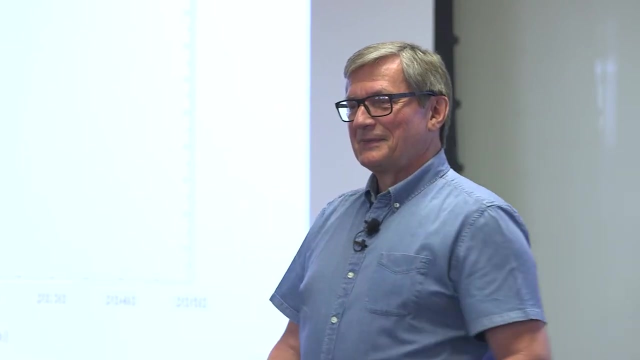 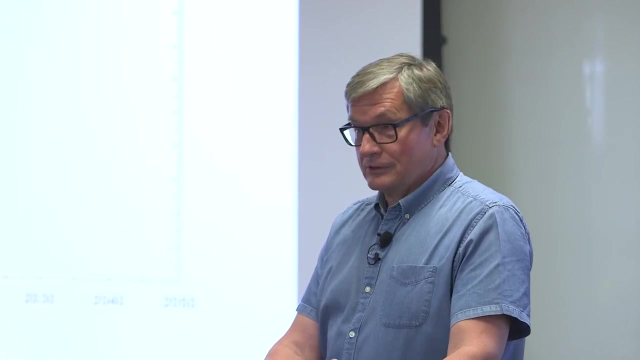 surface blue and 20 meters green Mean annual temperatures. And that's what, first time I made you know I was brave enough to put this straight line. You know, just very, very simple: model Regression, linear regression, boom, And it was. it surprised me a lot Because, say, 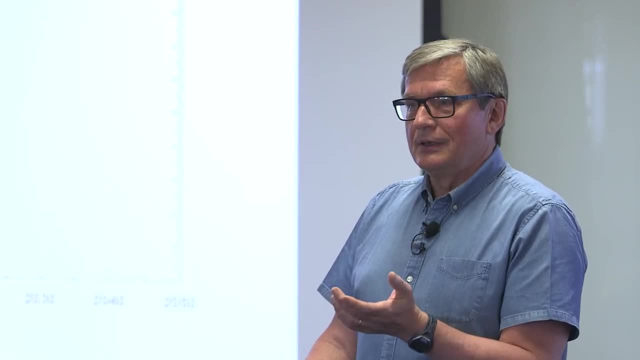 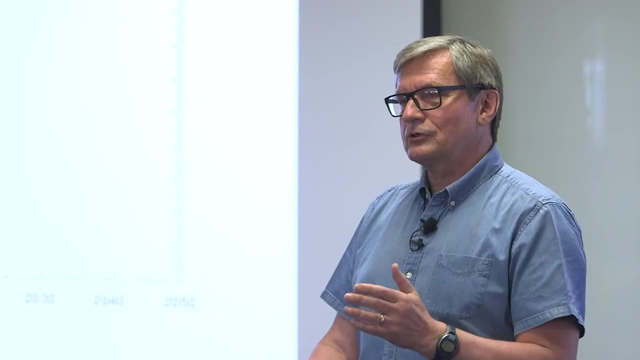 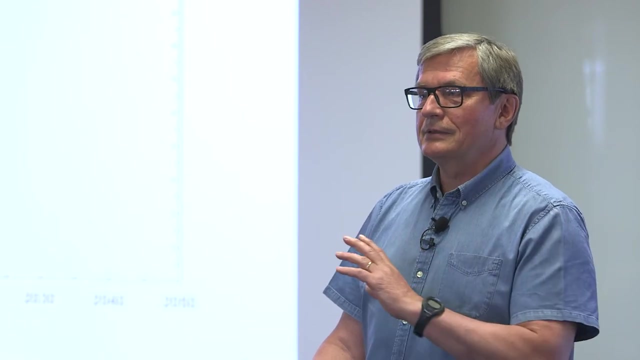 before we start to look and we collect enough data. everybody from permafrost community- they were strongly believe that permafrost on the North Slope of Alaska will be stable till the end of the century for sure. That was. that was very, very clear. 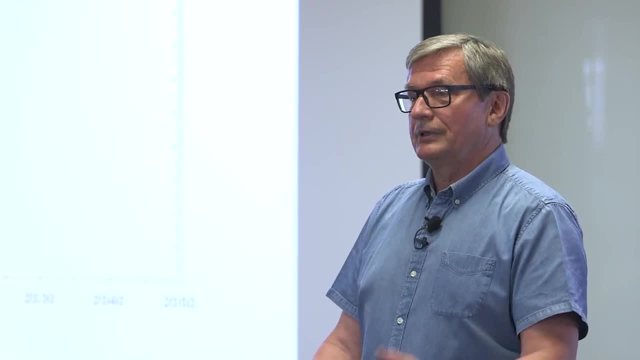 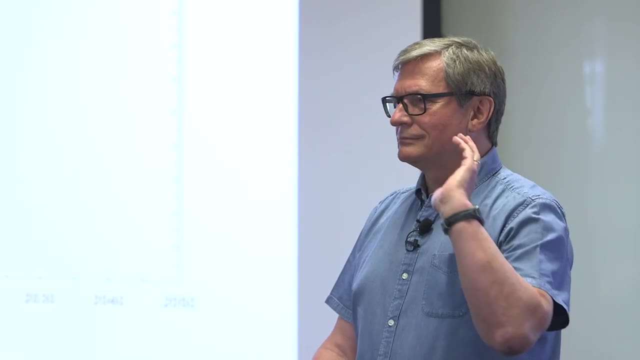 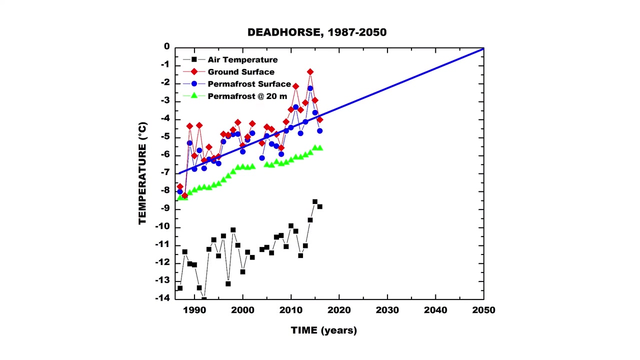 And still still common, common belief. I mean Alyeska pipeline. still, when they did some renovation of the you know permit, they said: well, permafrost on the North Slope is stable, You shouldn't worry about it. Well, I was very surprised that actually the straight 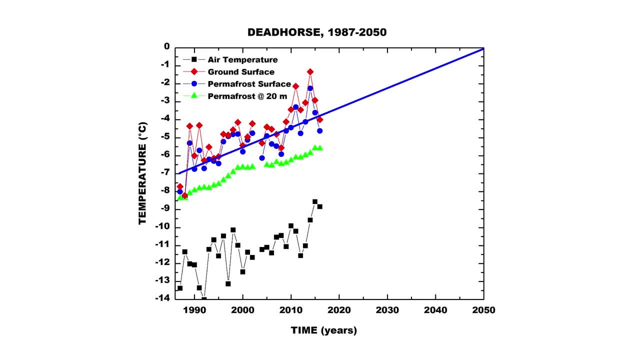 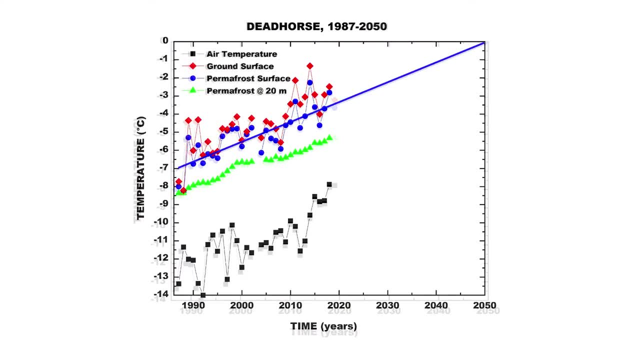 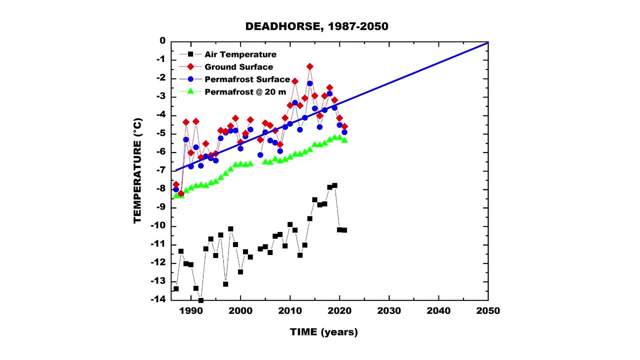 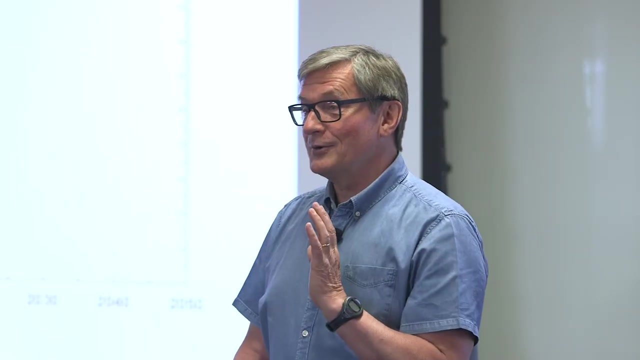 line hit zero degrees Celsius at 250, 250. And then since then, we continue to collect data and see where it goes. Well before last last two very cold years, it was going right where it should be Now. 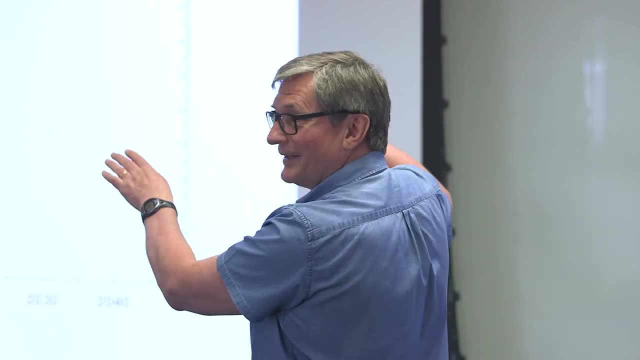 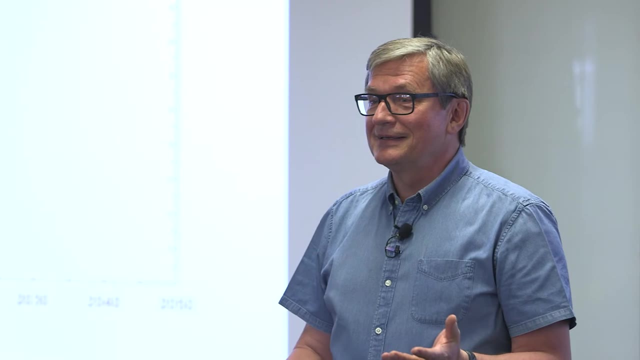 I'm not sure. Maybe we should move this, this straight line, a little bit and it will give us another five or ten years, But still, even that at 200, I mean 2060, it's, it's not. 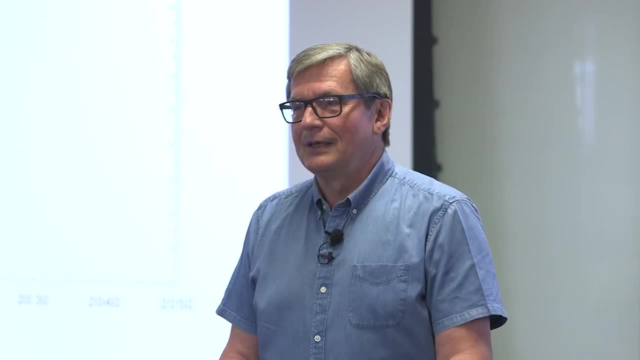 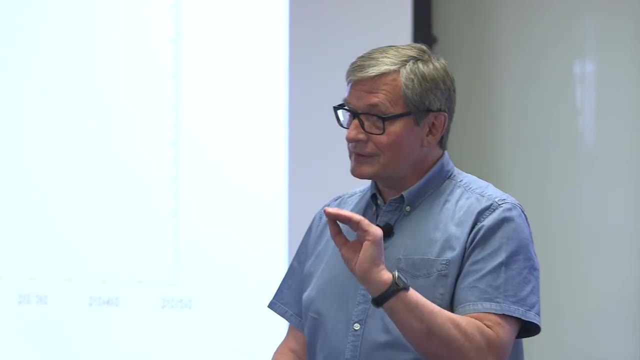 even it's middle of century, It's not the end of the century, And that's where our surface permafrost, surface temperature will be approaching zero degrees Celsius. Of course, there is some physical processes which will slow down because ice will start to melt partially. 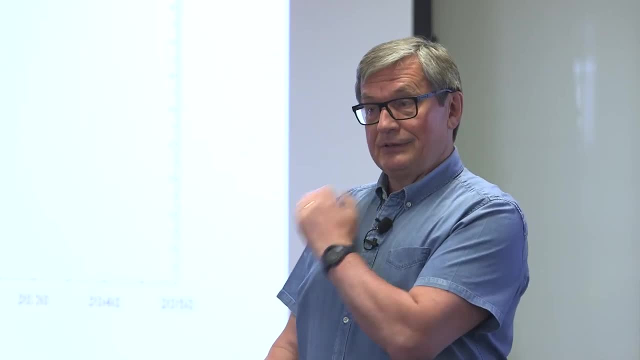 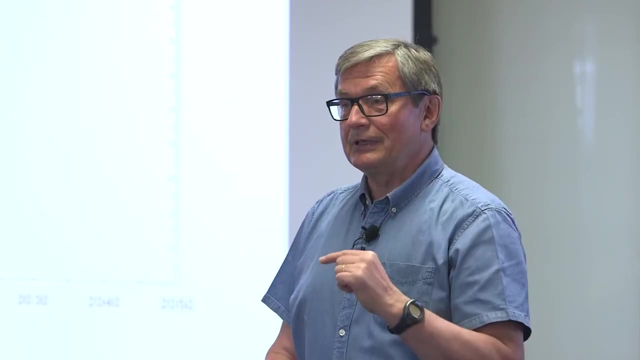 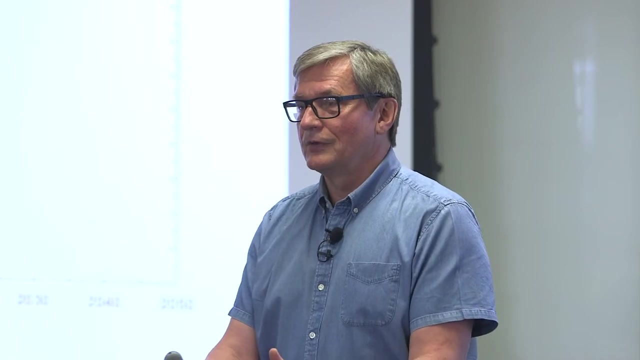 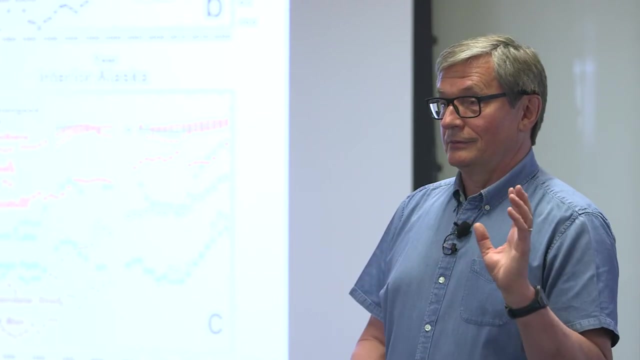 Lots of energy will go to it. It's definitely at this point the crossing zero in on my my line. Nothing dramatic will happen immediately, But permafrost will start to thaw, And maybe a matter of ten years. So now that's about cold permafrost, which we thought it shouldn't be any problems. But 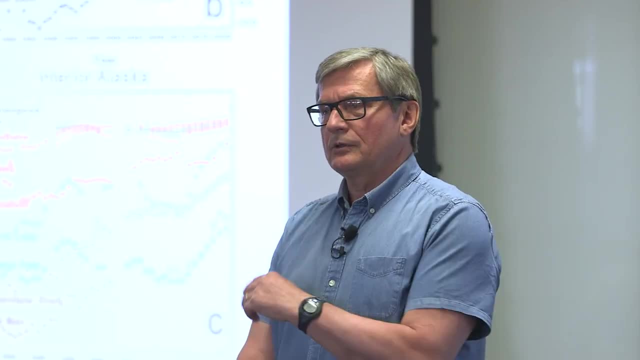 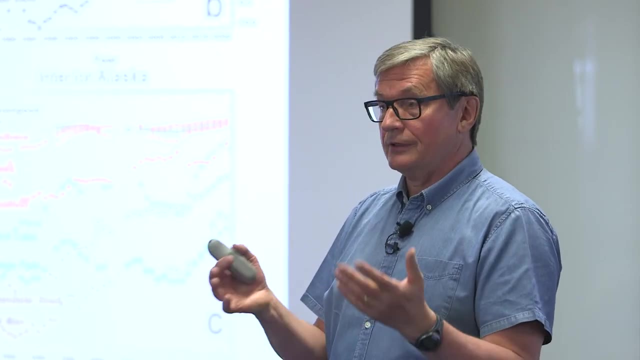 we already have some problems And, of course, on top of that- and I will, if I will have time, I will show some examples in infrastructure, Infrastructure make this problem even worse, because infrastructure itself, any kind of buildings, pipelines, roads, they add to this. warming itself. Just the construction of of this infrastructure affect permafrost in. usually if there is no special cooling, like it was done for Alaska pipeline, for example, then any, pretty much any kind of infrastructure will make permafrost more vulnerable for warming. 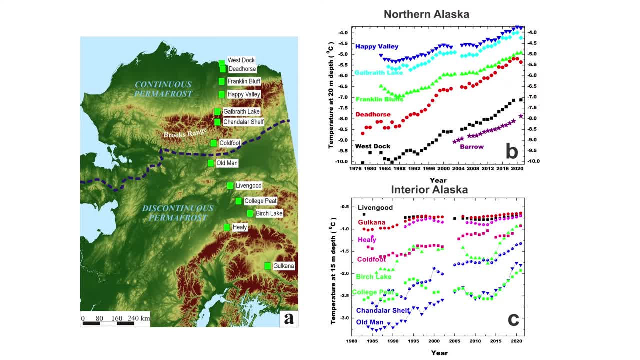 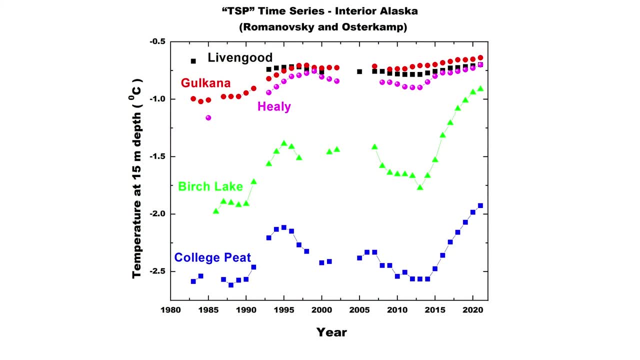 So now let's look what's happening here in the interior of Alaska. Lots of things too. So that's only sites in interior College Street it's, it's Fairbanks, pretty much Birch Lake. it's halfway to Delta Junction, Healy, you know Galkana and Livington. 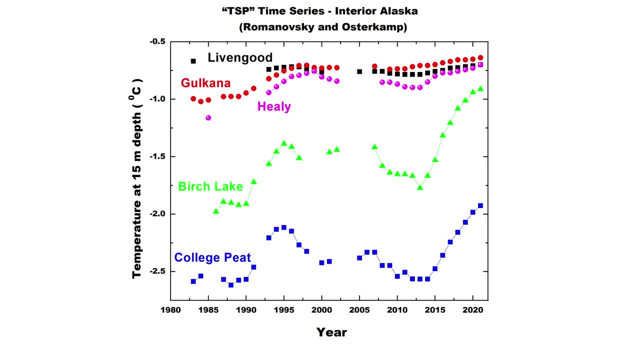 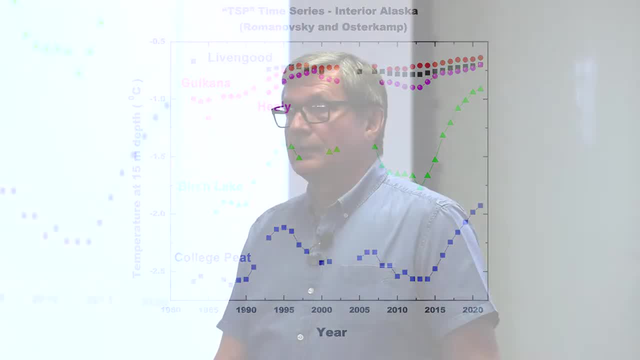 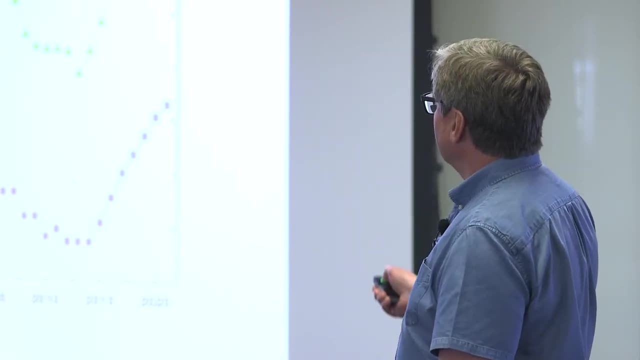 So for colder permafrost we still have general warming. It was a little bit of up and downs until somewhere like 2013,- 2014.. It was warming and then cooling a little bit And but since then we have very, very rapid warming in Alaska And that's also all right for Healy. 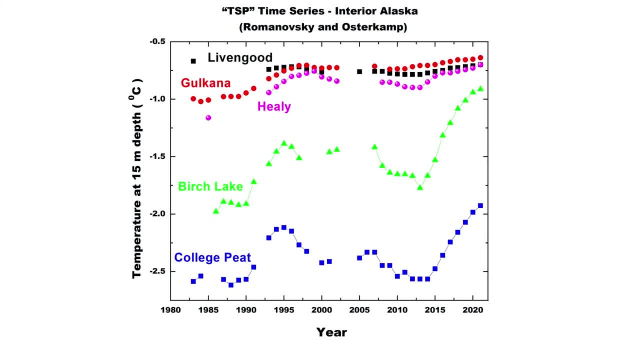 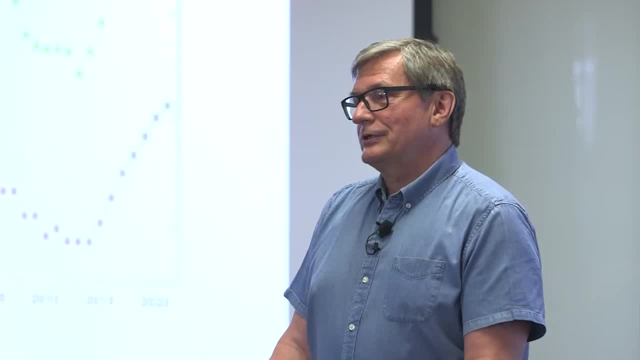 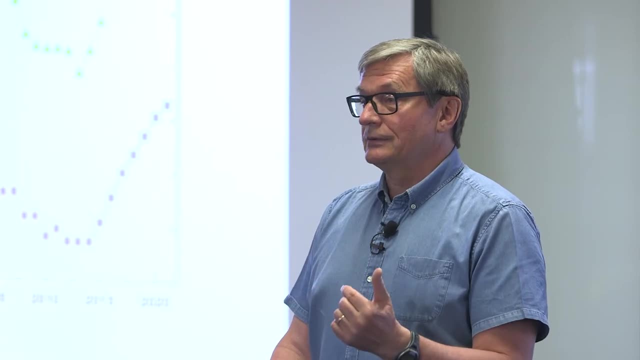 Interestingly enough that place like Livington, the temperature already was minus 0.7.. It doesn't change too much. Well, there is physical explanation. In this case, temperature is not a good indicator of changes Because at this temperature in silt, which is pretty much what it is there, 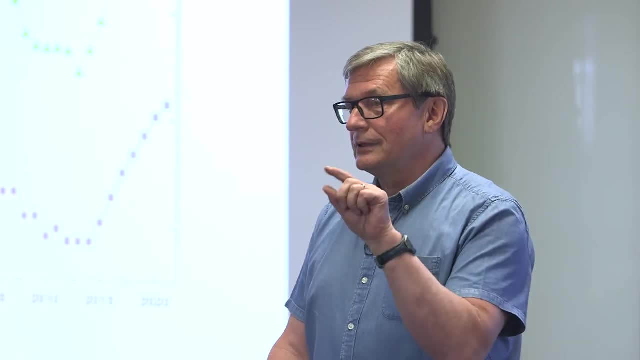 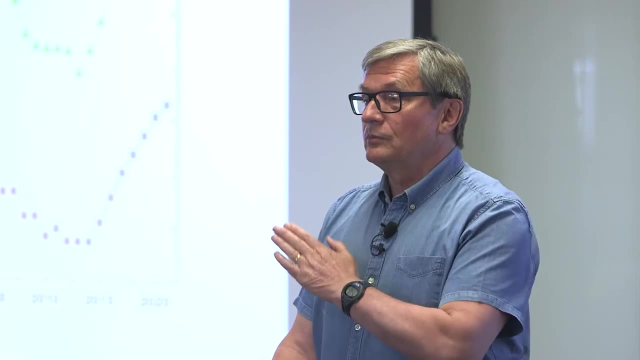 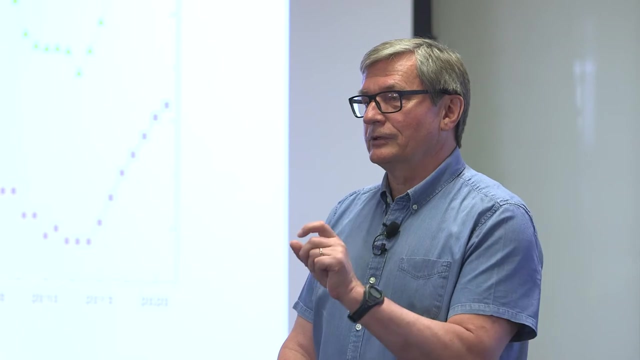 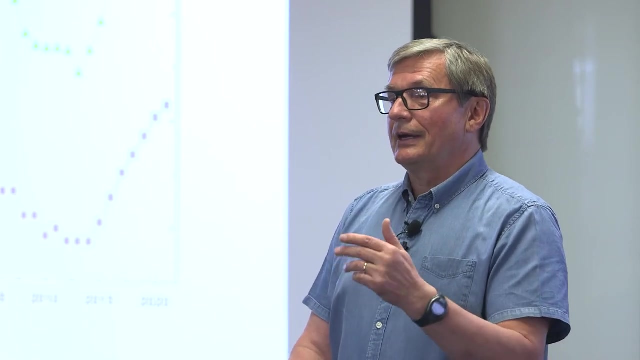 in silt ice in in between the- you know- granules of the material starts to to melt Even below zero degrees Celsius. That's very well known physical fact Because of water in this case it has no free water structure, So it's actually melts. ice melts at a little bit lower temperatures. 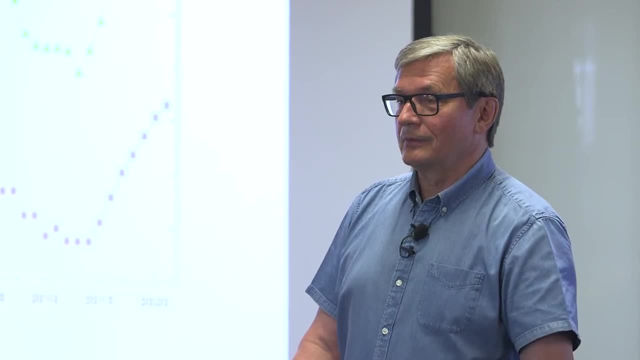 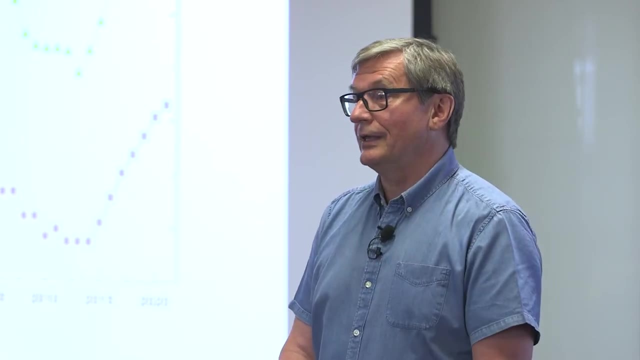 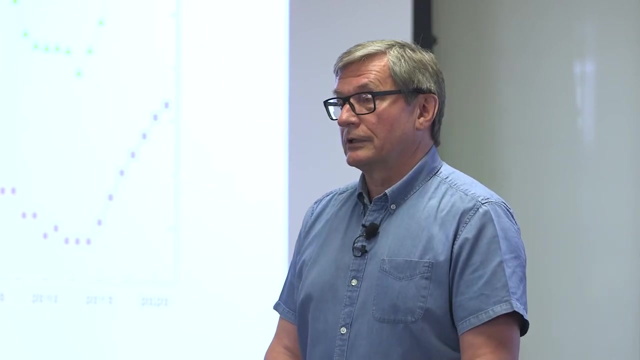 The same is like under pressure, The same is like some impurities: It all make ice melt Like sea water. for example, it freezes at minus 1.8 degrees Celsius. Another zero sea ice because of the inclusion of of sea water in it. So, and because of 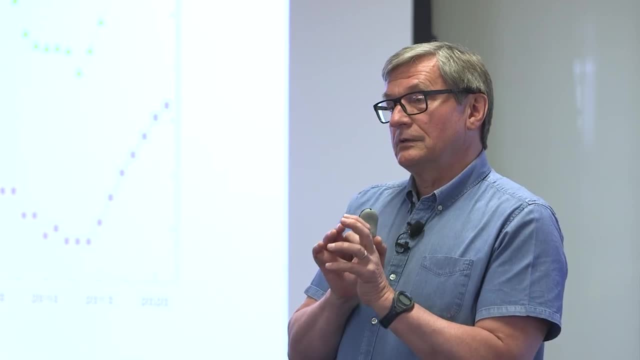 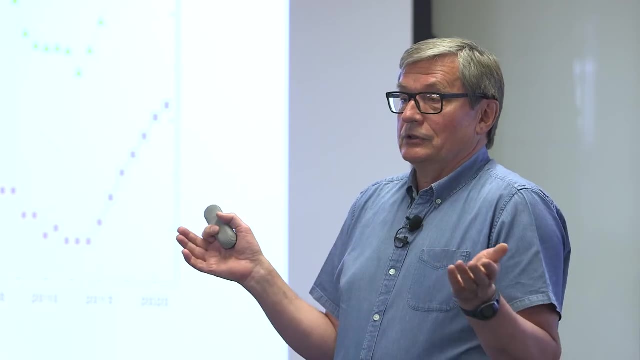 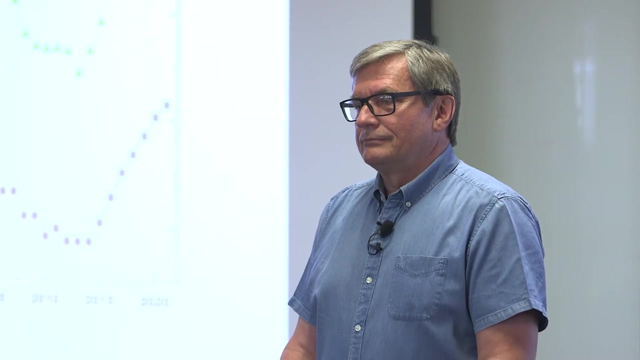 that and this minus 0.7 is enough already to start to melt ice partially a little bit, But lots of energy going into this process and temperature doesn't change. It's the same. is the same as say I don't know. in school our teachers always say this: You have a cube. 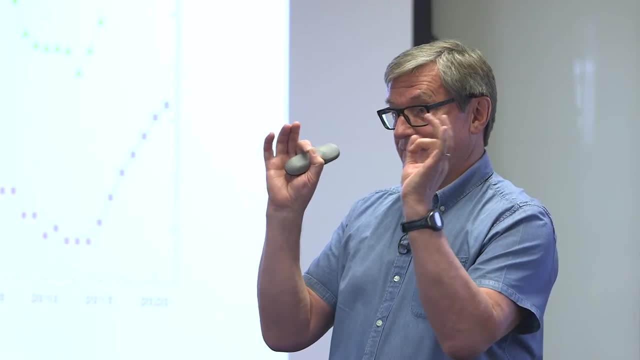 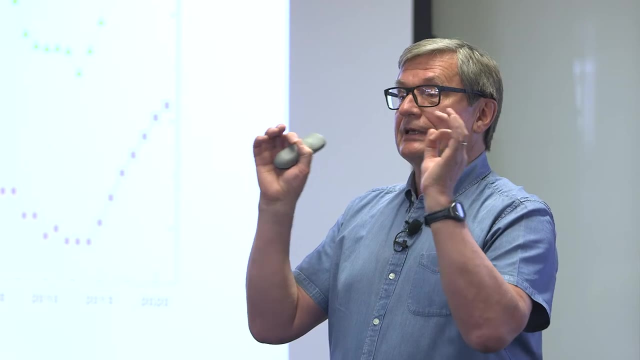 of ice and a cube of water, exactly the same size, exactly the same, And both of them are zero degrees Celsius, And you start to warm them with exactly the same amount of energy. So what you will see: The water starts to get warmer and warmer, and warmer The cube. 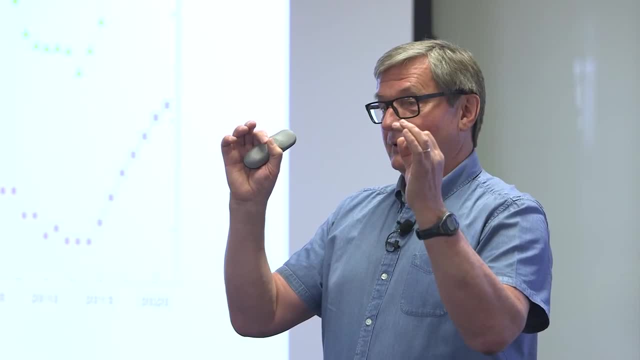 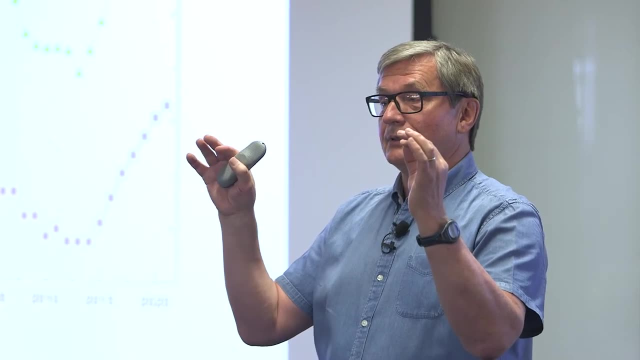 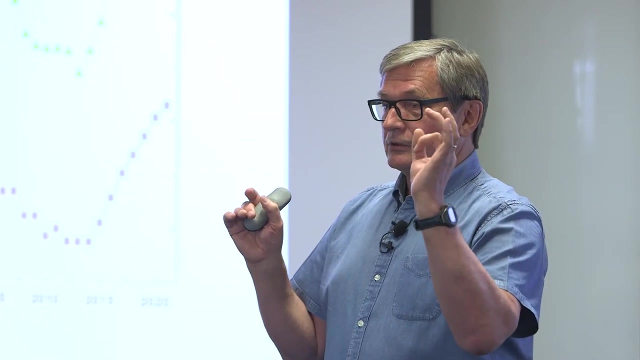 where ice was. it's kind of start to melt, but temperature is still zero, zero, zero, zero, zero, until all ice melted and became water. You know what? By the same time, the same amount energy, the water cube, which was water originally, it will be a temperature. 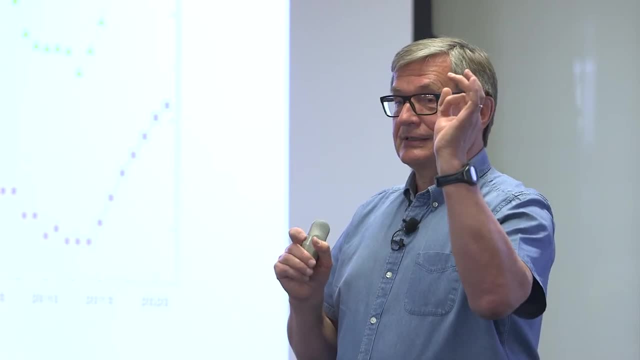 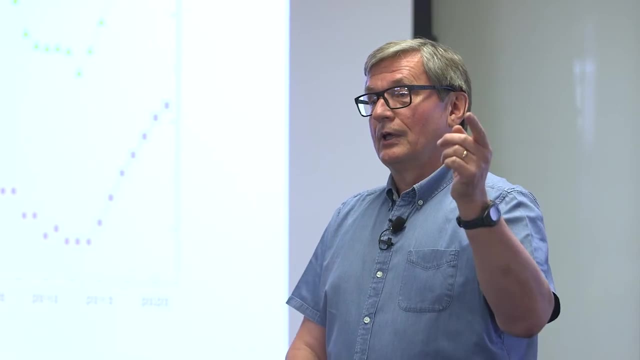 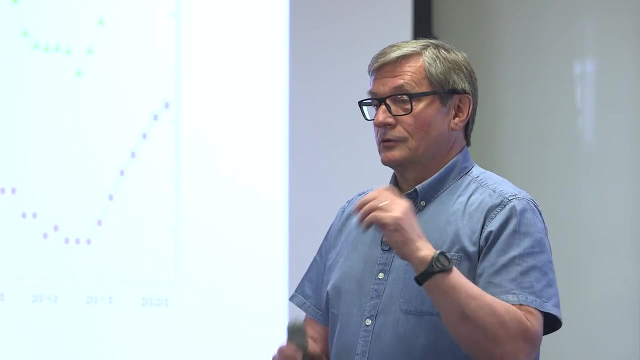 plus 80 degrees Celsius. 80 degrees Celsius: That's the difference between how much energy you need to put into ice to melt, Compared to how much you can put energy you put to water or any other material to make it warmer. So big difference. So that's why even small amount of ice turning into water, 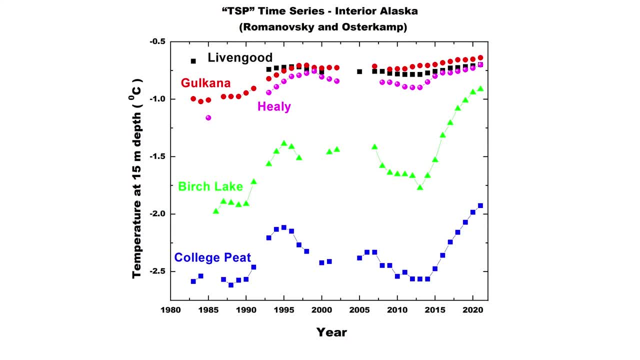 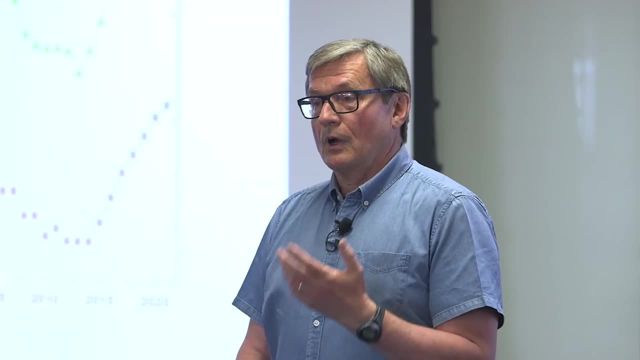 takes pretty much all this excessive energy which goes here in warming of permafrost And that's why temperature is kind of warming but not really. In this case temperature is not good indicator Of the state of permafrost. probably we should- and we start already- measure the liquid content. 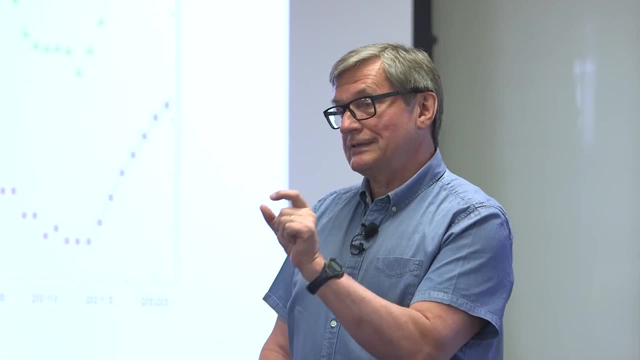 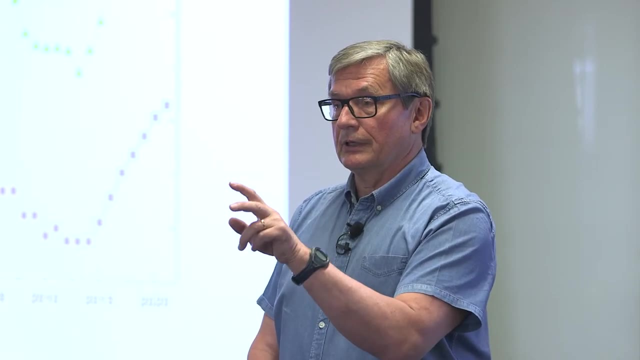 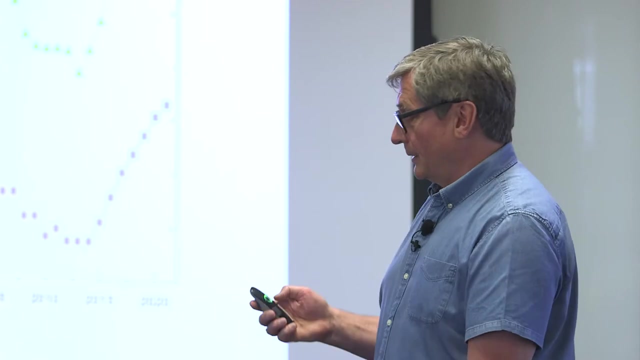 So how much liquid water is there? And we obviously see that, with temperature not changing too much, the liquid water content, portion of water and ice water is increasing and ice is decreasing, So that's probably a better indicator what's happening there, Maybe too. 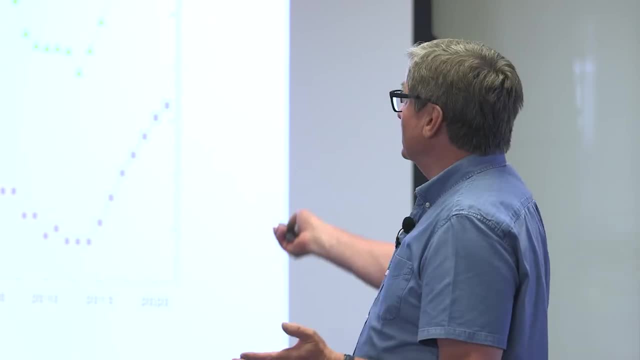 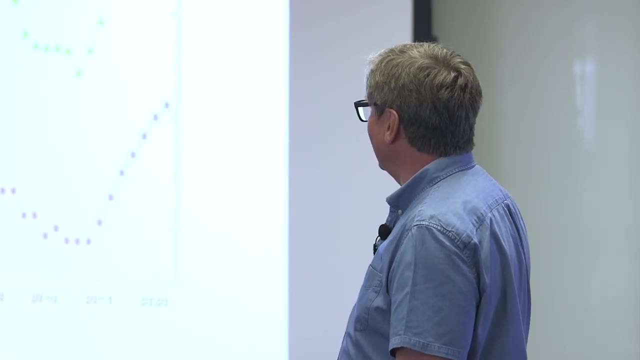 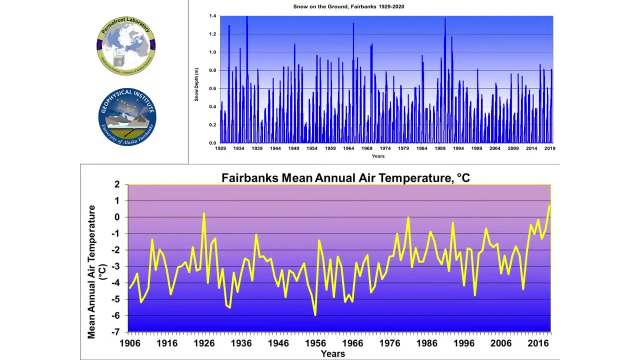 much science here. But that's explanation. I'm trying to explain, Because question is why there is not changing anything And here is so much change. That's because of that. And again, if you look at the forcing air temperature, mean annual air temperature at 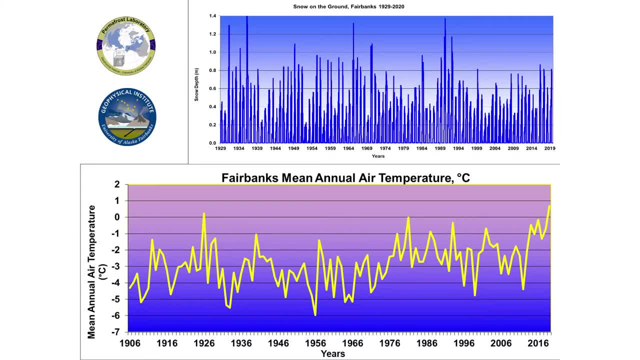 Fairbanks Airport Med Station, which we have records actually since beginning of 1900s. So it was again similar to actually a little bit earlier warming here, then cooling and then step-like jump in about mid-70s. Since then it was actually not that much warming. 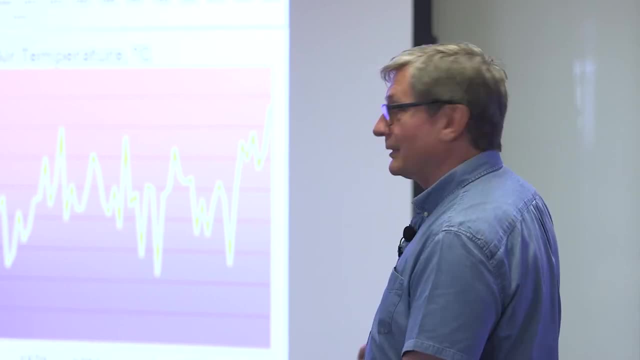 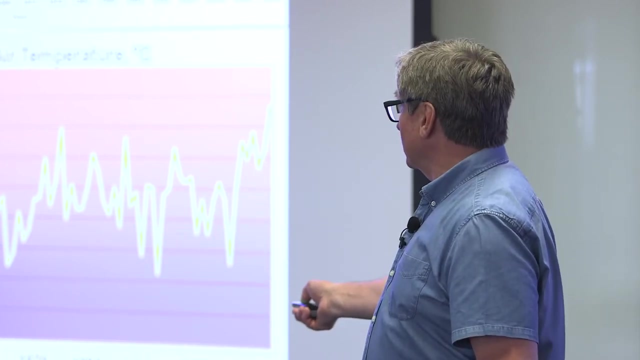 even a little bit of cooling, And only again about 2013,, 2014,. we have new wave, new wave of warming very similar to what we had here, So we don't know if it will sustain or it. 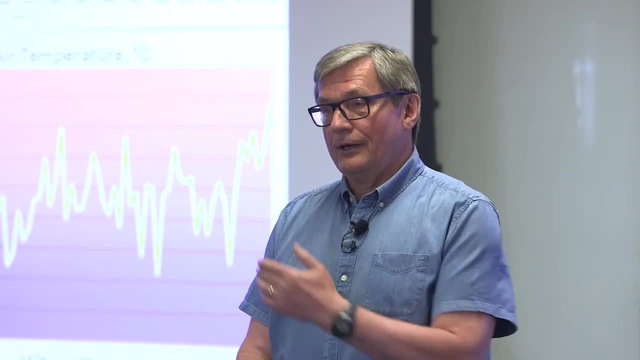 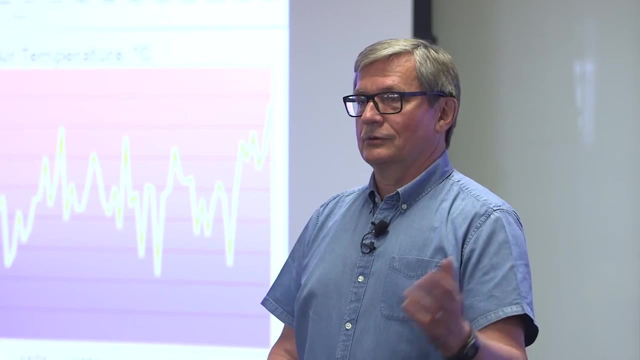 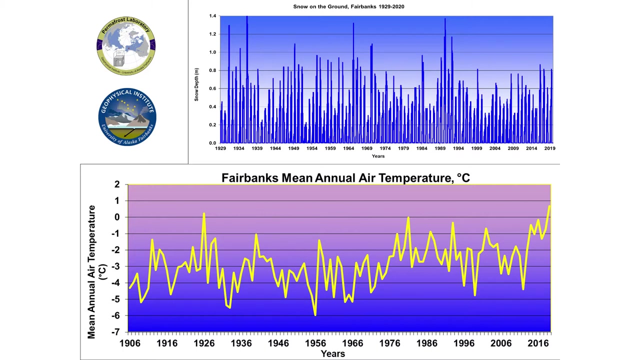 will you know go, But at least up to now we have very, very strong warming and increase in air temperature, And that's how permafrost react. It's also get warmer and more excitedly. of course, snow is also important and that's why, for example, in 1990s- who remembers beginning? 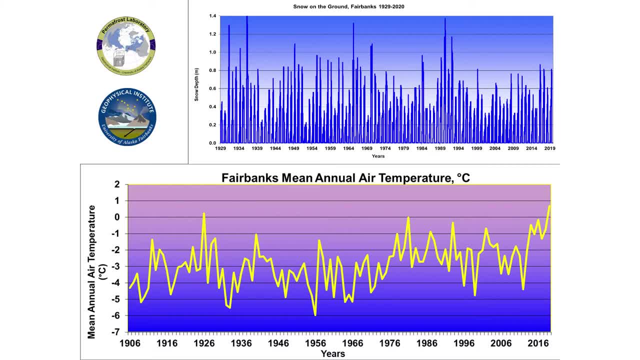 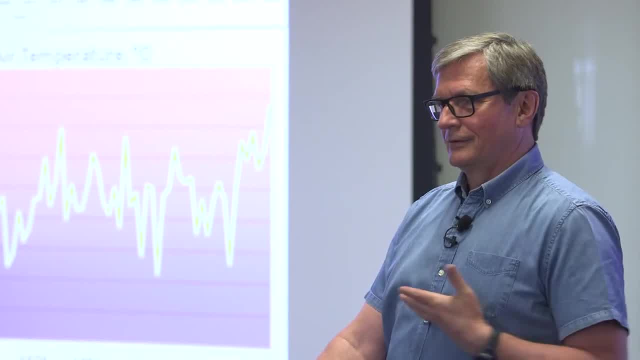 of 1990s, it was lots of snow, much more than even last winter, which we always say. oh, it's lots of snow last winter. Compared to 1990s, no, It was like a meter and a half. 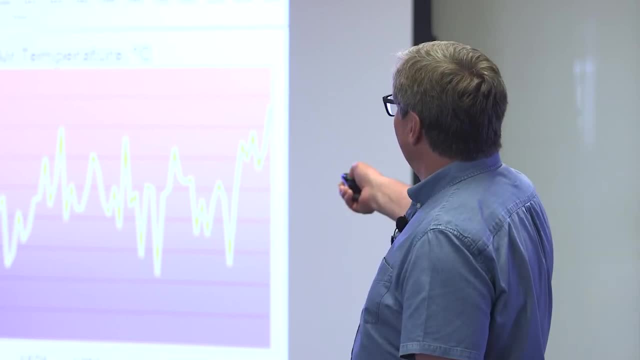 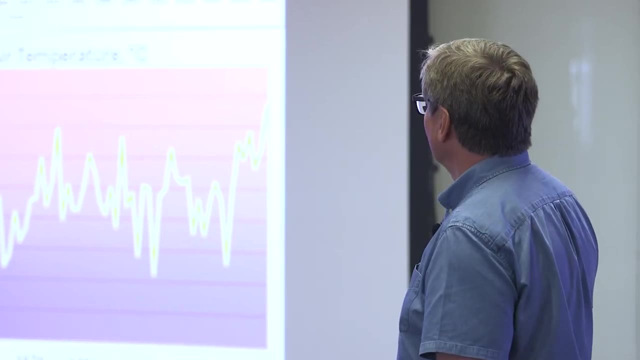 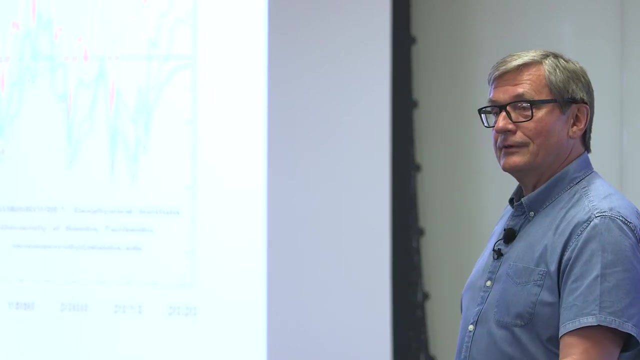 That's when I bought my snow blower And then I got, in the beginning of 2000s, Almost no snow. Anyway, it's still useful Again, OK. so now what's happening here is very different from what happened in North Slope. 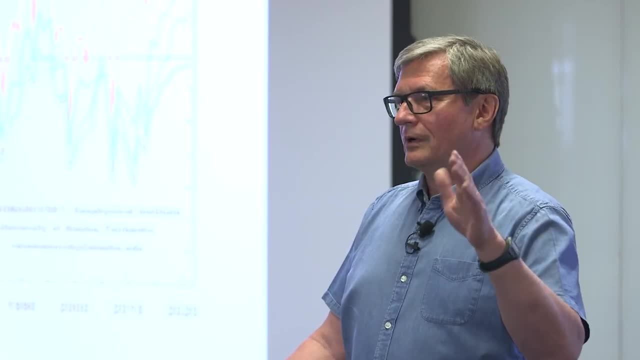 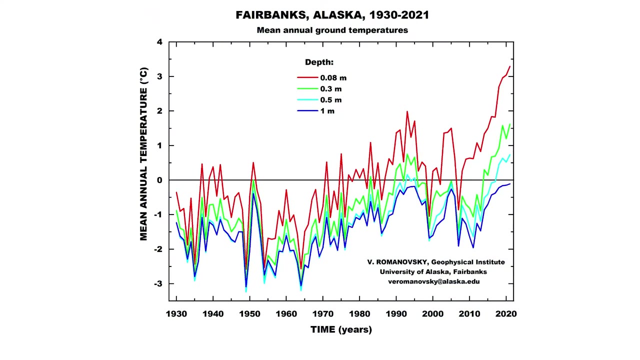 Even with all this warming, we still remember minus 4,, minus 5,, minus 3, but still minus. So around Fairbanks it's LTR side, Bonanza Creek, LTR Temperature at 1 meter in permafrost. 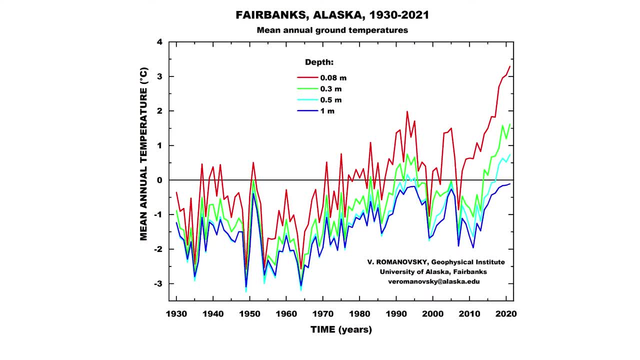 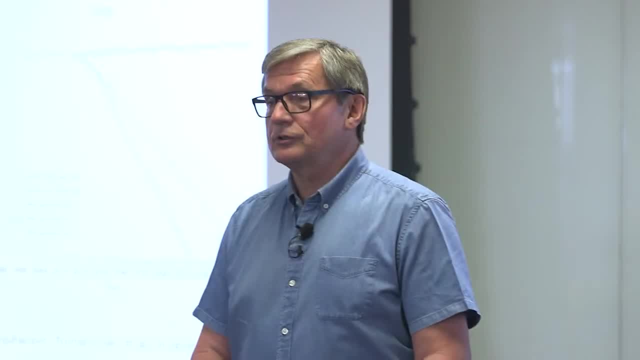 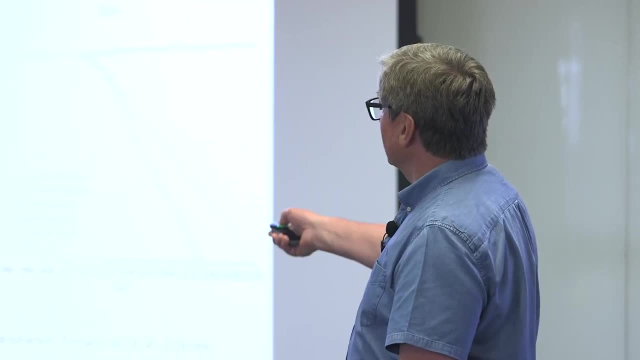 is really really critically close to 0 degrees Celsius- very close- And because of that actually permafrost started to thaw. So it's a little bit complicated graph, but let's look at this part- very exciting part, Because there's all this warming. 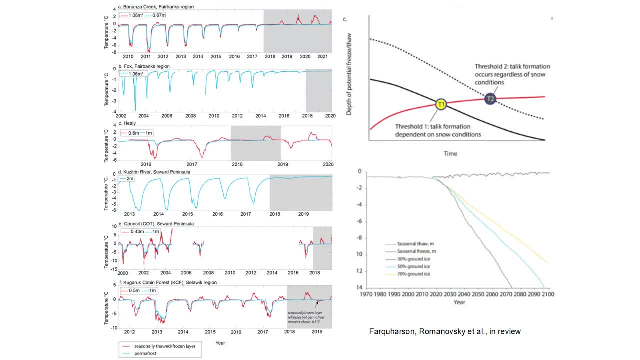 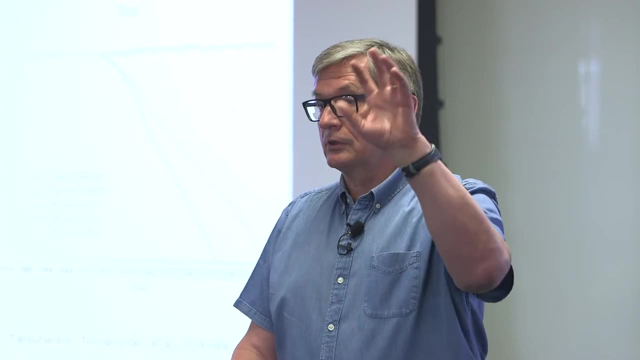 people in media would ask: there's lots of warming, lots of warming. What is the thawing of permafrost? They said: well, it should come, just be patient. Finally, this last warming wave in Fairbanks, and not only in Fairbanks, but in all interior. 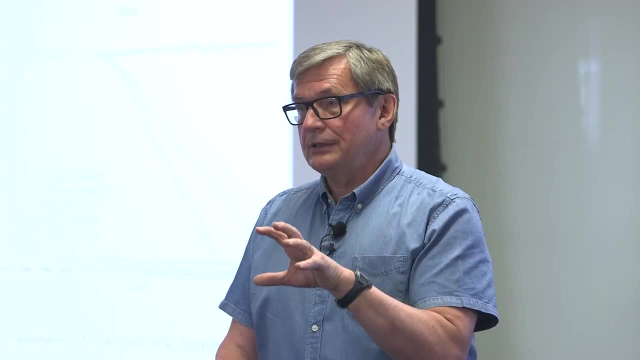 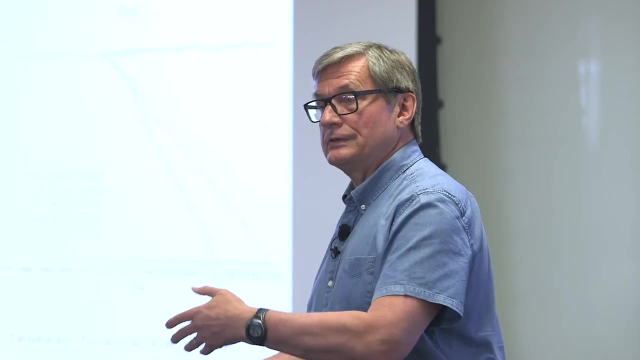 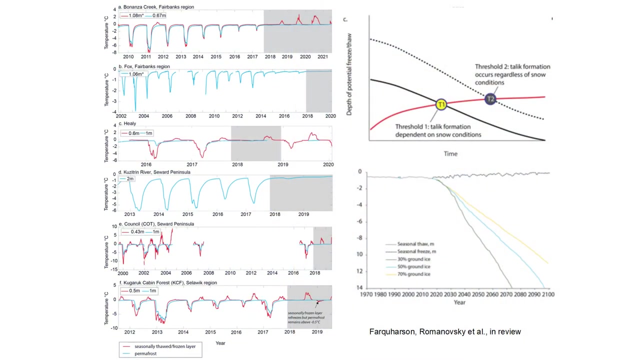 including Seward Peninsula, create the conditions where permafrost start to thaw, And this layer of thawing now is deeper than winter freezing. Look at the left side of this graph, which is showing the temperature at a little bit shallower depth. 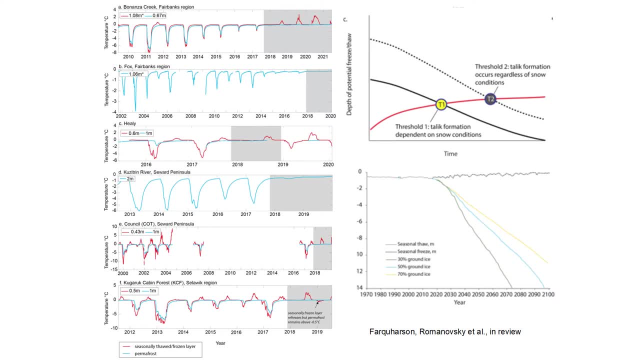 and a little bit shallower depth, a little bit deeper depth, And you see that in the past this is kind of normal behavior of stable warm but stable permafrost Every time you have warm and thawing in the upper part, which is active layer. but then during the winter it freezes, completely, completely frozen, everything frozen. And by end of the winter, if you drill hole from the surface of the ground down to, say, 15 feet, it will be all frozen, no thawed layer. 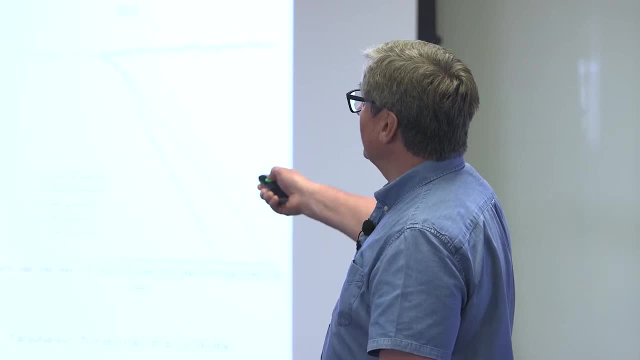 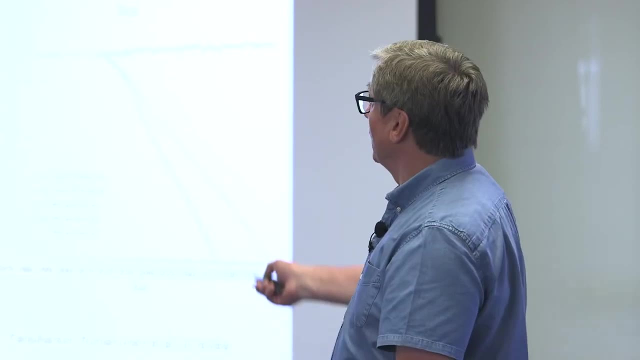 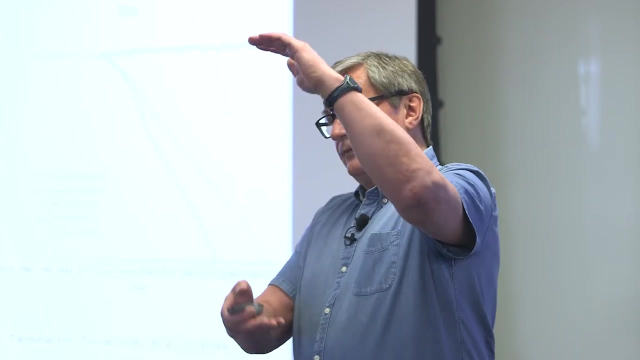 What will happen when this second warm wave came- and that's actually happened massively in many locations- I will show on the second graph that it stopped refreezing completely And by the end of the winter you'll see the frozen layer not reaching permafrost. 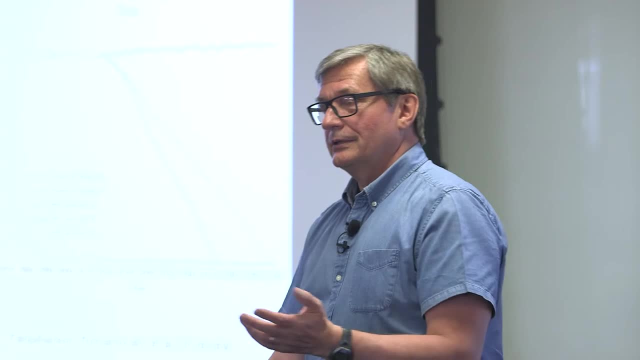 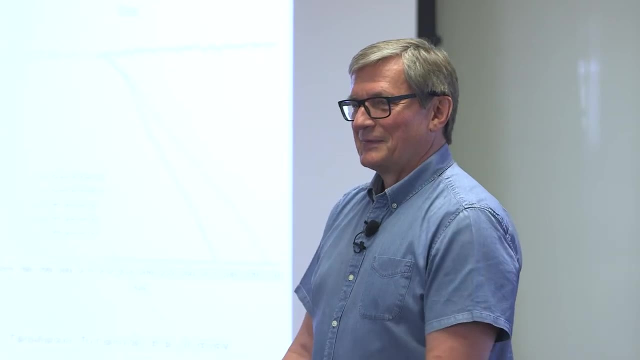 And there is some layer in between. We call it talic- Talic- it's actually a Russian word And now it's a scientific term. It means simply not frozen. Tali. not frozen, But that layer survived over the whole winter. 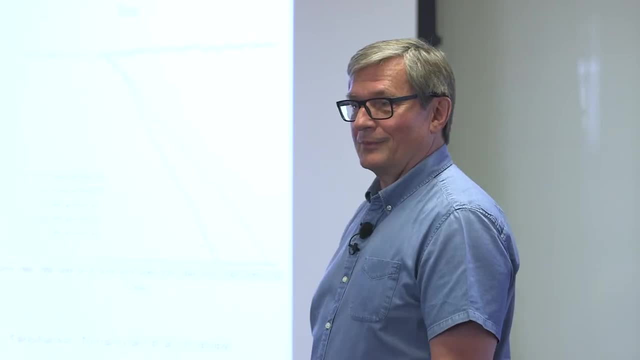 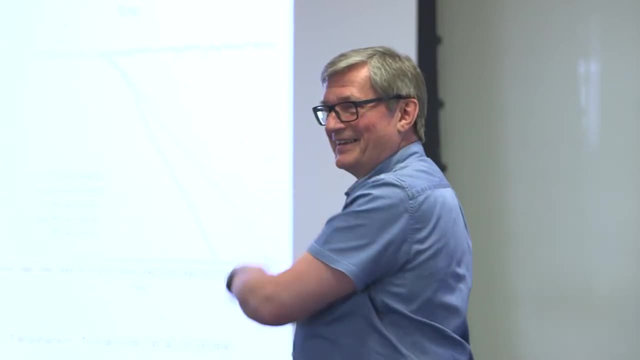 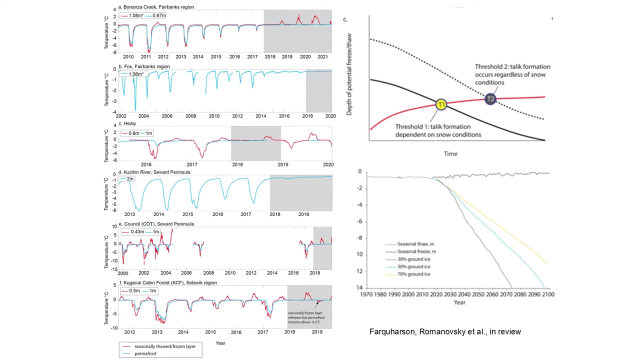 And you can think about this as a cardiogram of permafrost: Ding ding ding, ding ding ding, Eh Kaput. So that's indication of that permafrost will start to thaw and develop this layer of non-frozen all over the winter. 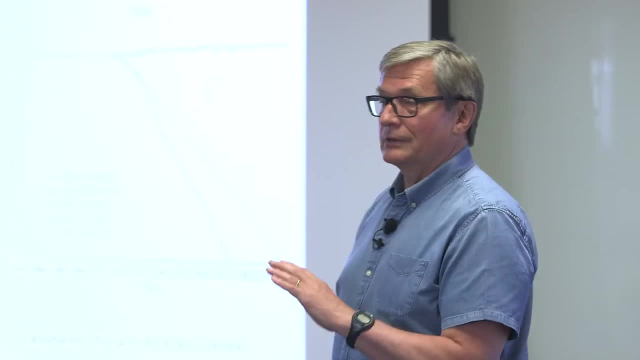 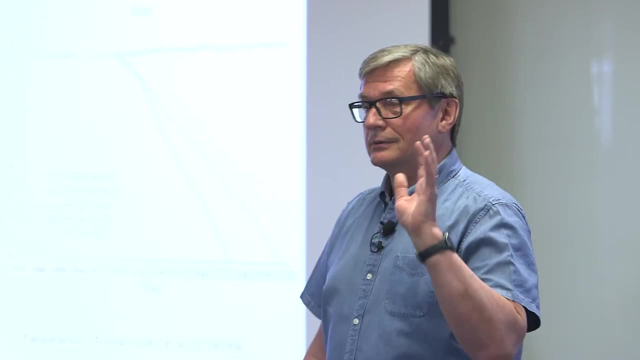 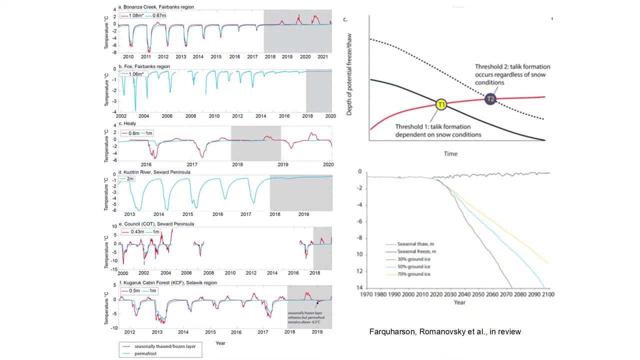 or year-round actually, And of course implications for that are huge For microorganisms, for water, for vegetation. lots of interesting things happening And eventually, if it will continue, this is already our modeling, this talic or layer which 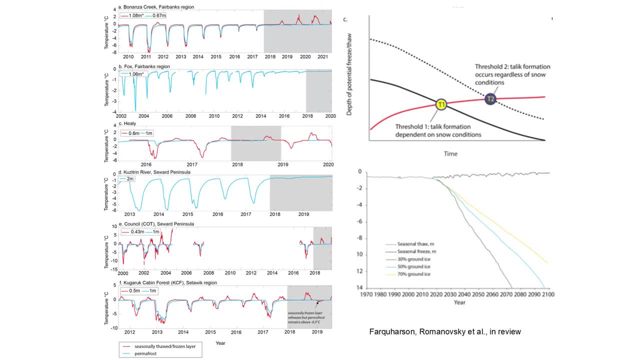 is not freezing at all- will be getting deeper and deeper and deeper And by the end of the century- this is again- but not the crickets Fairbanks site- what I showed- data Depending on how much ice is in permafrost. 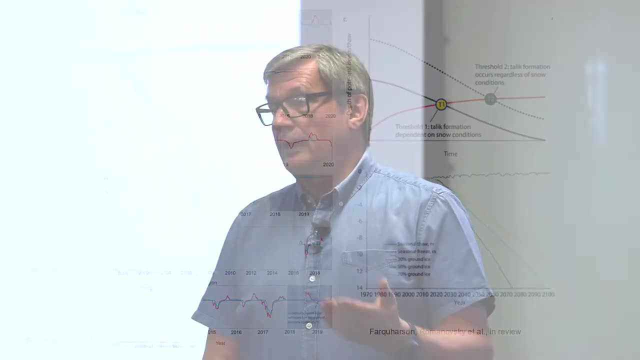 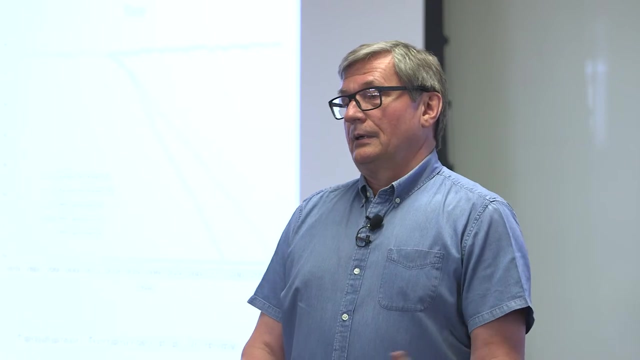 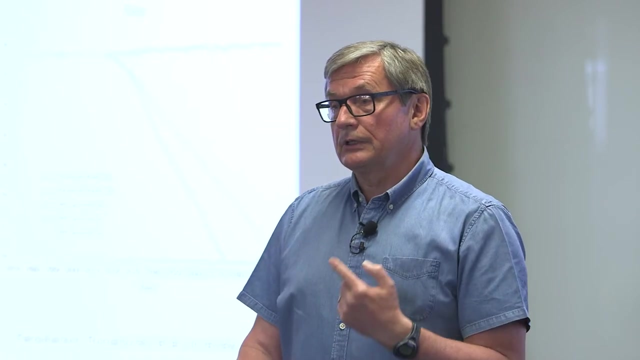 it actually can be thawed by 14,- 15 meters, which is 45,- 50 feet not frozen And most of the ice- what we discussed before. most of it is in that upper 50 to 30 meters around Fairbanks. 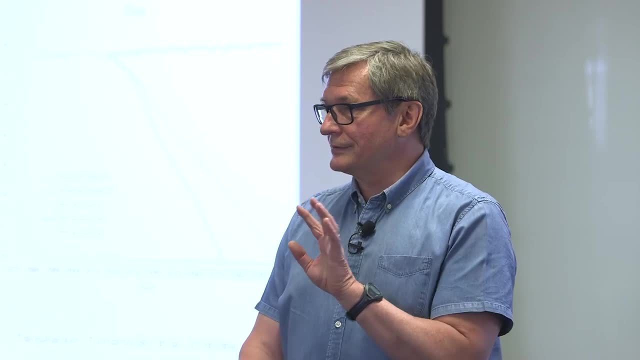 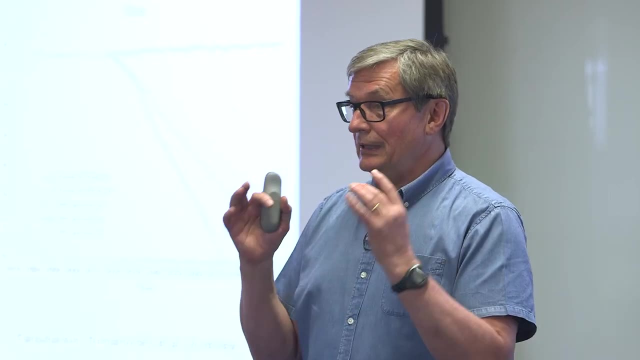 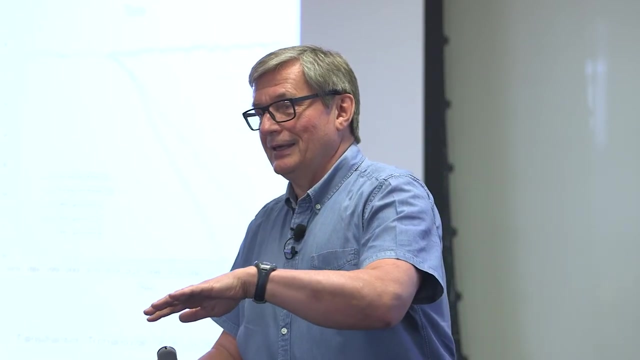 So it means that- and this is case where no ice like massive ice, ice bodies- We didn't consider that, Because in case of ice, there will be completely different story, Because surface will be subsiding and thawing will propagate much faster actually. 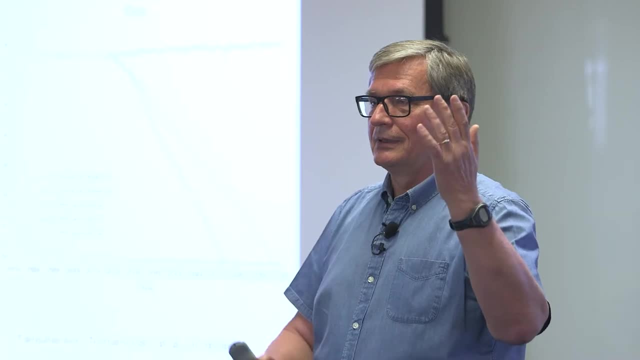 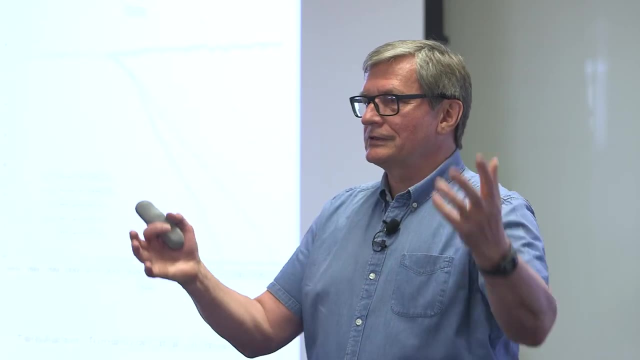 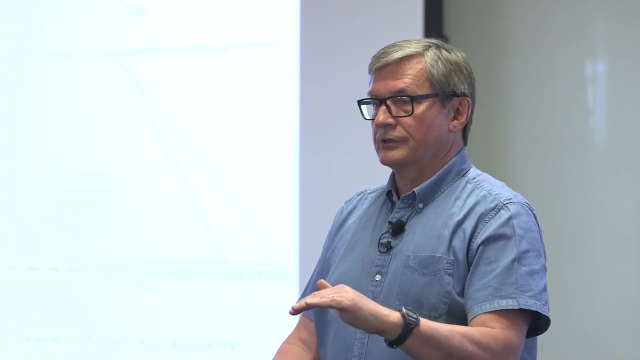 destroying pretty much all landscape which is sitting on it. I don't know if anybody visited permafrost tunnel, right? So in permafrost tunnel, imagine how much ice is there, And it's all somewhere like between 7 and 20 meters depth. 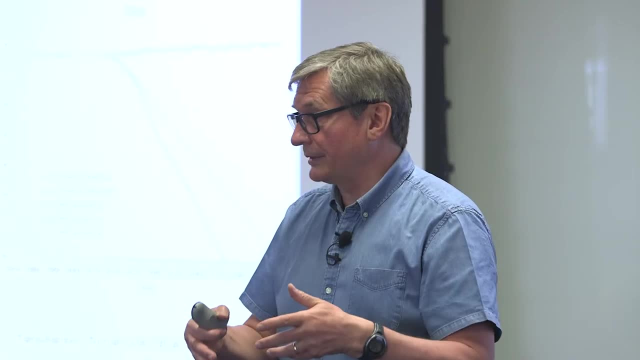 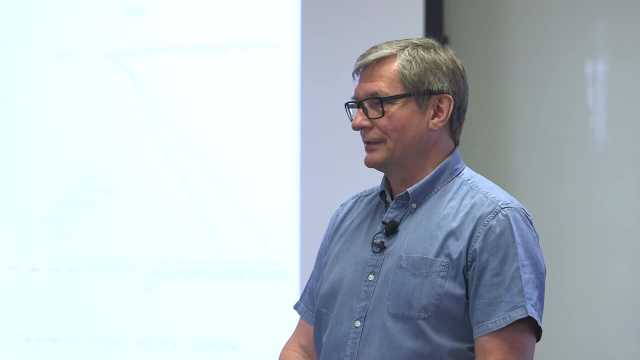 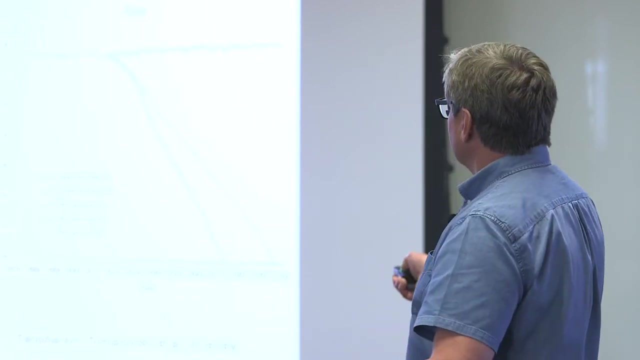 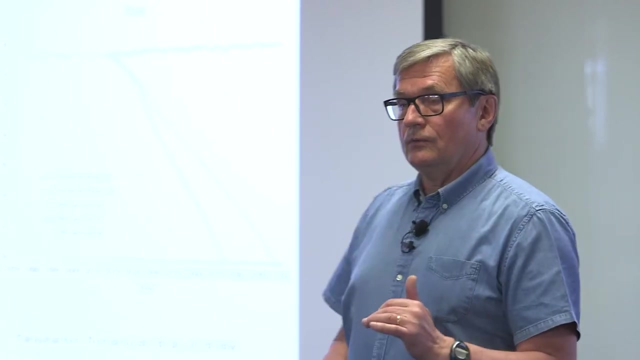 So if this thaw will penetrate in this ice and it will melt, that will be complete reorganization of landscape. I would say So it will be turned into muck, just So. that's what we are saying. Again. we are at threshold where cold winters, low snow winters, 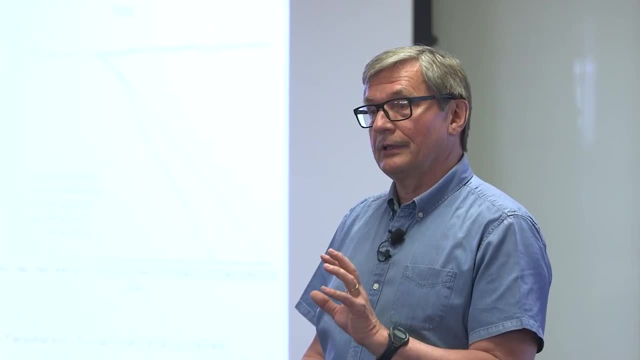 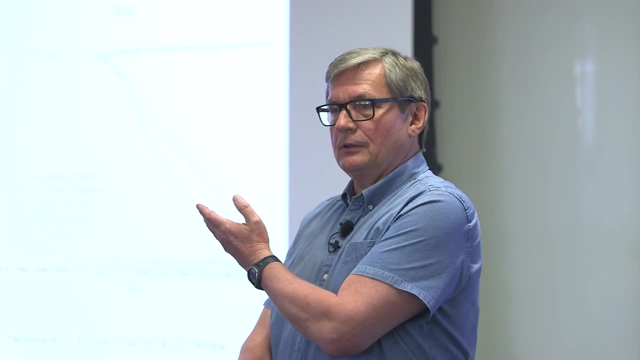 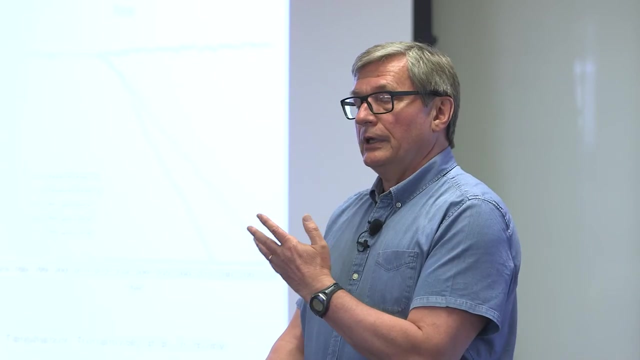 still refreeze this stalag, this new developed stalag. It's still possible, But a little bit later. OK, Later. if warming will continue like it was, having happened before this point, then we will go into the area where, no matter what kind of snow you have, 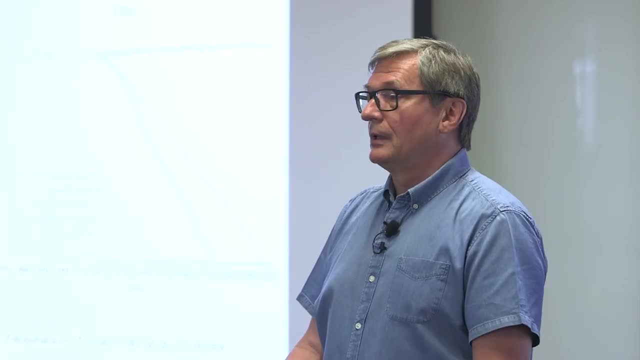 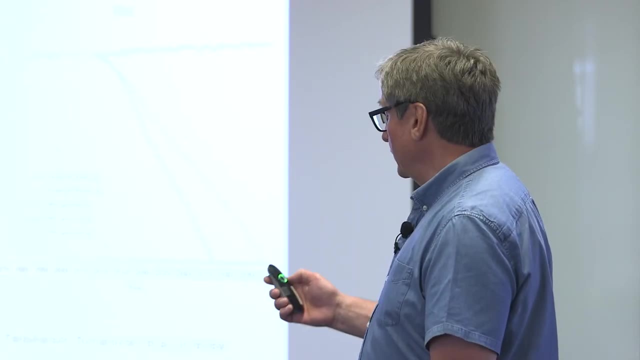 no matter what kind of cold winter you normally have, stalag will survive. And in this point it will continuously grow and grow and grow deeper and deeper and deeper. So that's pretty much kind of diagram to illustrate. So when permafrost is still there, 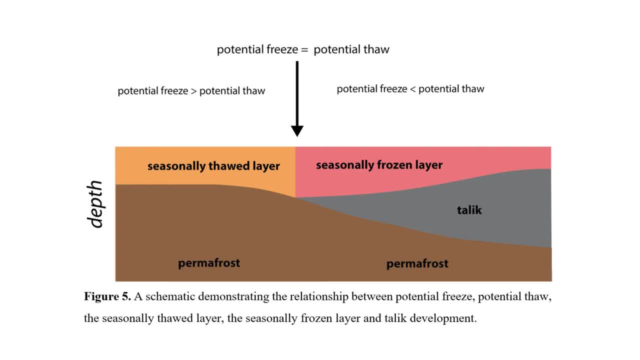 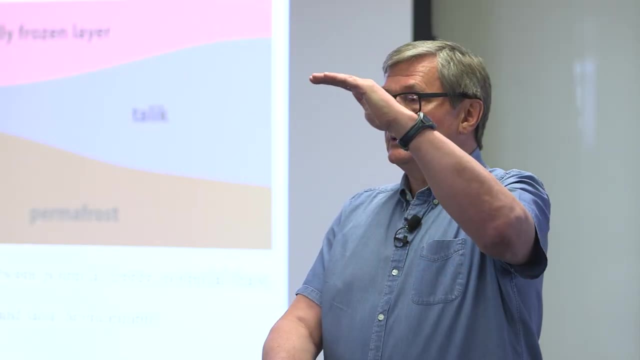 when this is stable, you have this seasonally thawed layer. It seasonally thaws, but it's completely frozen by winter over above permafrost, And then- this is the point, what we actually experiencing right now. So a little stalag, maybe just 20, 30 centimeters. 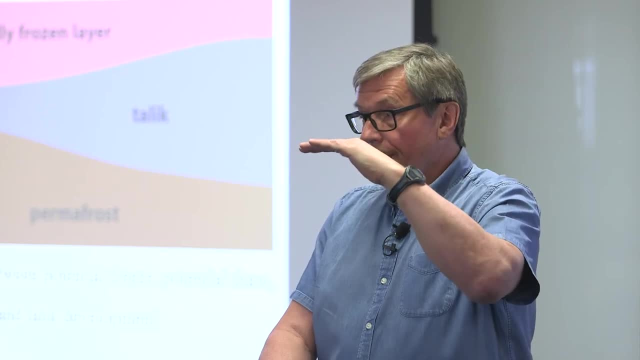 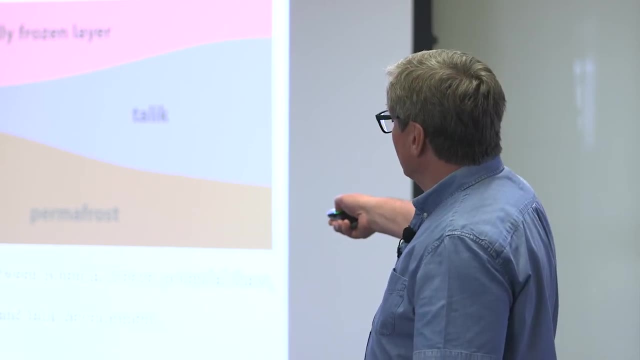 in many cases sometimes a little bit deeper, develop already. But in the future, if climate will be warming the same rate, so the, So the permafrost will, the top of permafrost will be getting deeper and deeper and deeper. And only seasonally frozen layer will be there, Because winters will still be minus 40. That's guaranteed for a long time, And during this winter of course some material will be freezing. But again there's warmer winters, which actually winter's warming faster than summers. 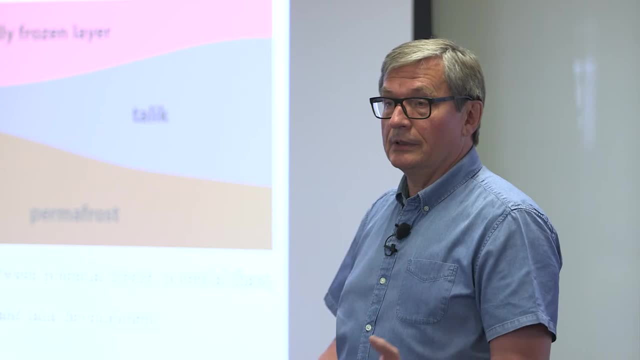 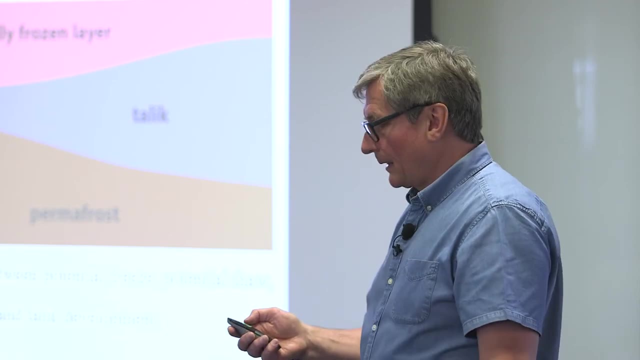 This layer thickness will be shallower and shallower, And now we're modeling By the end of the century. we have only like 15, 20 centimeters of frozen during the winter time, And that's what I promised you. So it shows where 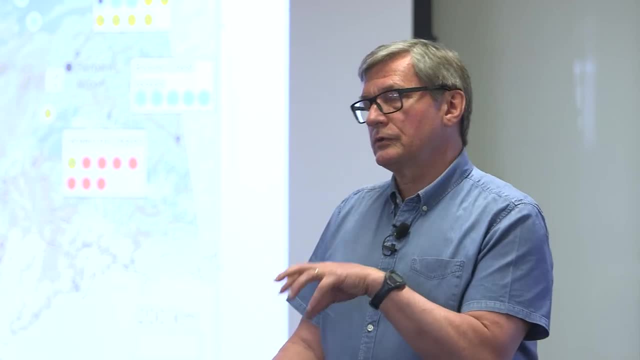 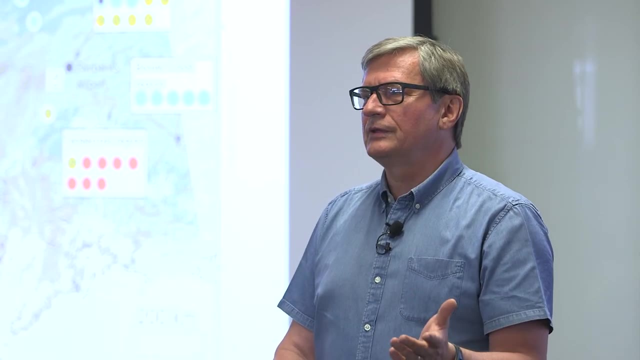 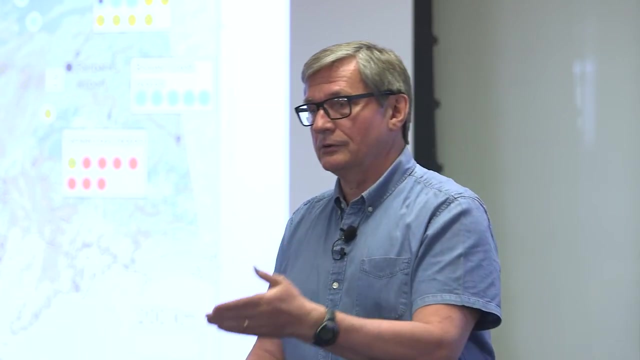 So we have many sites, Those ones with deep boreholes and that map with squares. there is kind of maybe 20 of them, But we have about 300 other shallow sites where we measure temperature at the shallow depths down to 1 and 1 half meter, down to 2, 3 meters. 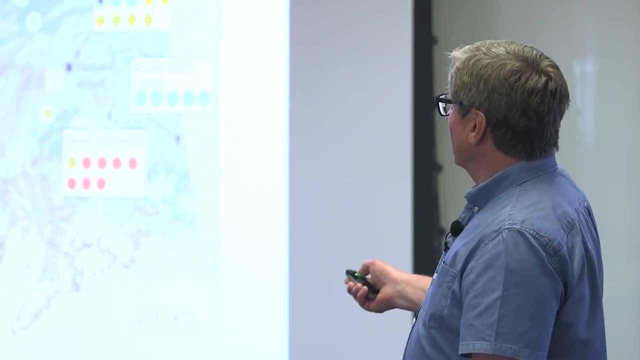 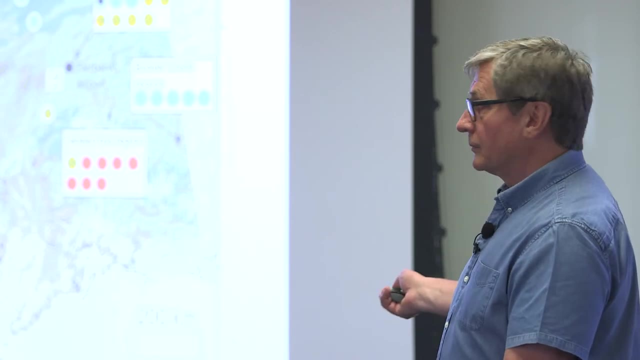 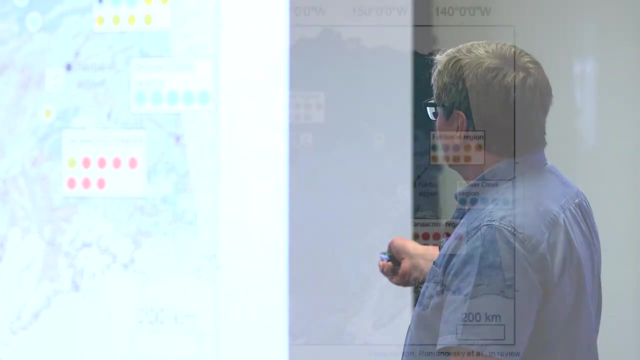 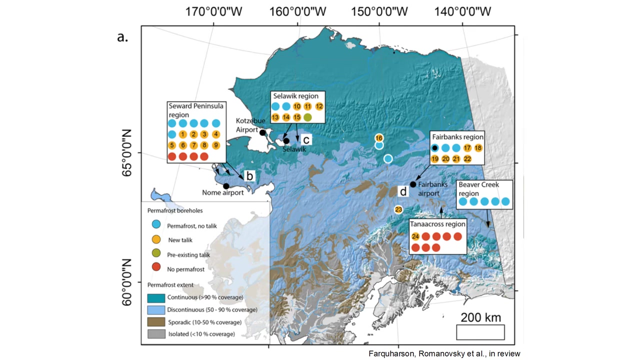 And in the latest work we just published, actually on Monday in Nature Geosciences- That's a figure from it- says in review, so it's published on Monday. So out of 54 sites we choose which before this latest: warming. 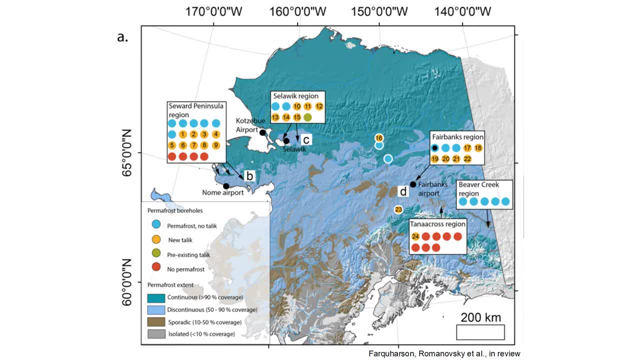 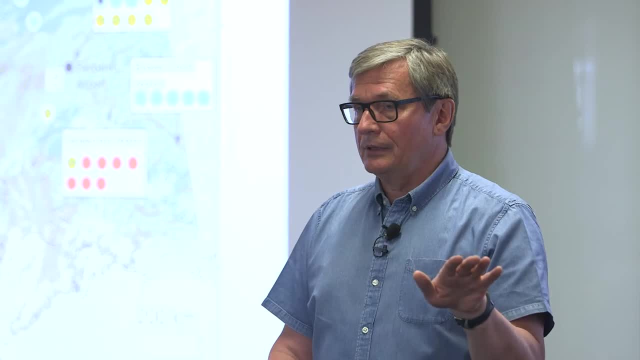 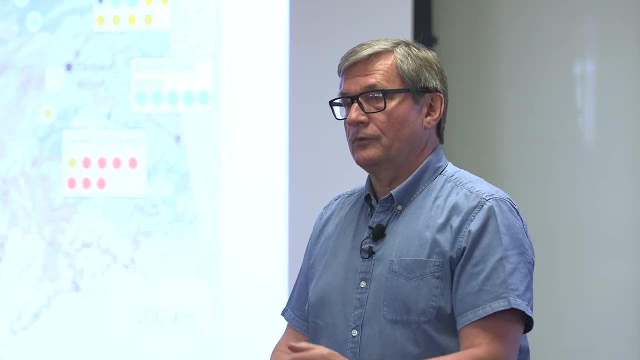 So out of 54 sites we choose where normal permafrost, where active layer was freezing completely before. 54 sites we choose not affected by any water, surface water or fire, because forest fire also make conditions make permafrost much more vulnerable. 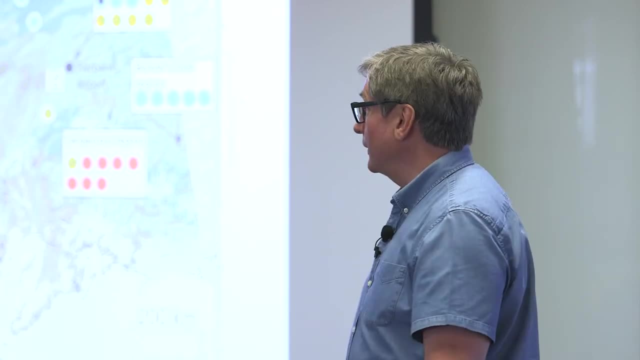 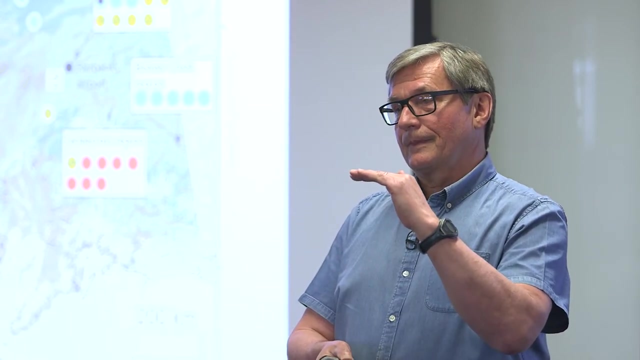 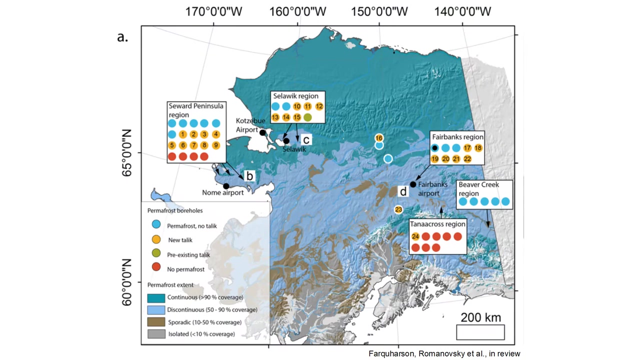 And usually it's slowing if it's severe enough fire. So out of 54, more than half of them showed this development of this stalag, And it's true for around Fairbanks, It's true also in Selavik area. true and the same. 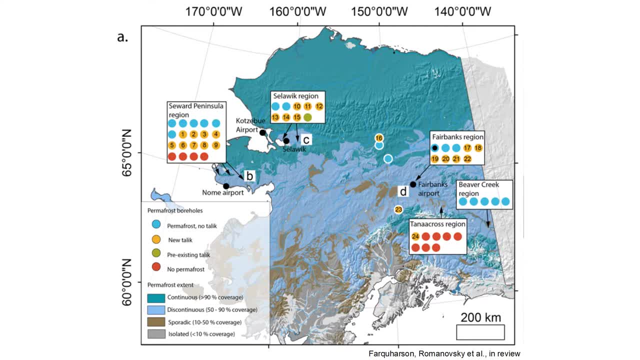 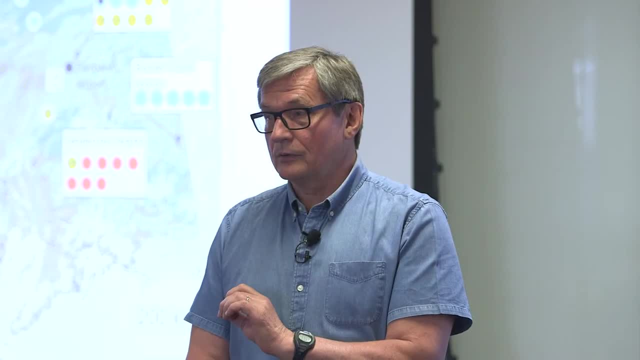 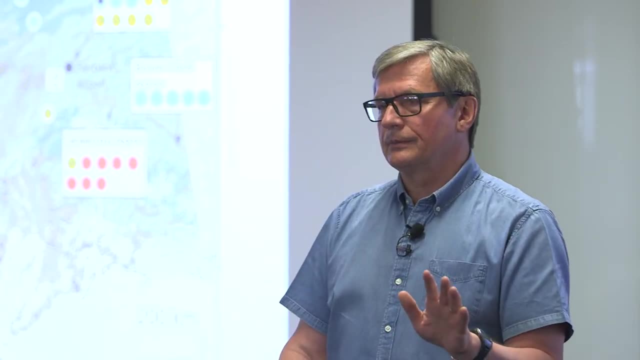 in Seward Peninsula, So it's pretty much very, very common. now Again, some of them may refreeze by now, But about in 10 years we will thread this second threshold, We will cross this second threshold And stalag will be stable and continue to. 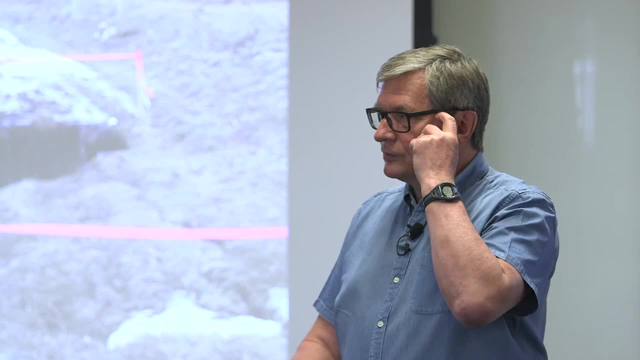 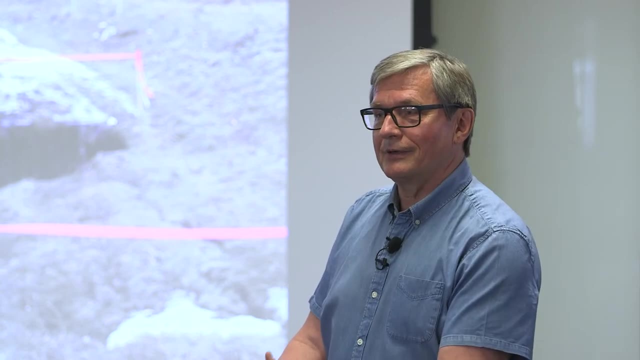 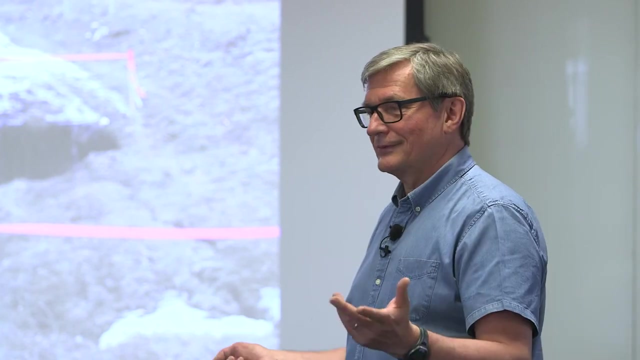 OK, I think I have a little bit more time. I have time. I mean no problem, Because typically it's an hour and a half class, You know. So I can stay longer If anybody would like to stay welcome. 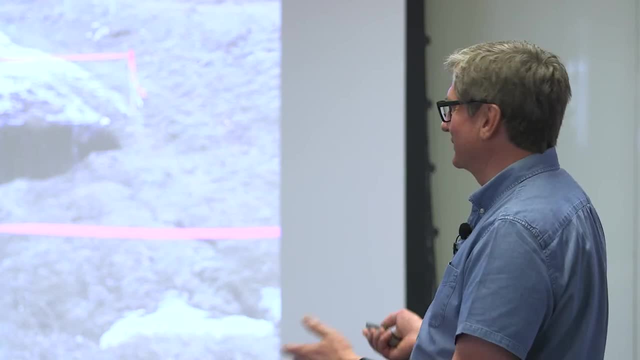 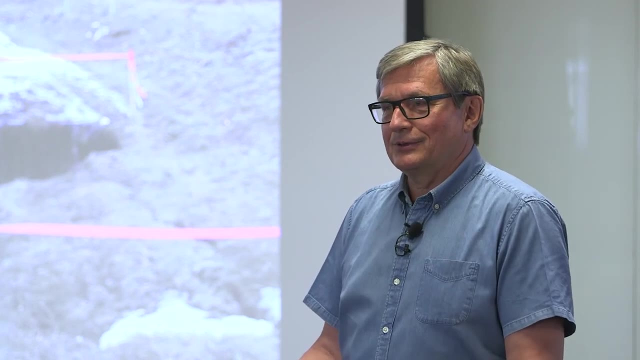 And, yeah, we need questions. I mean, we have to discuss what I'm talking about. So, again, what's for us? You know Why we should worry about this thing. Well, you know yourself. Sinkholes, for example. 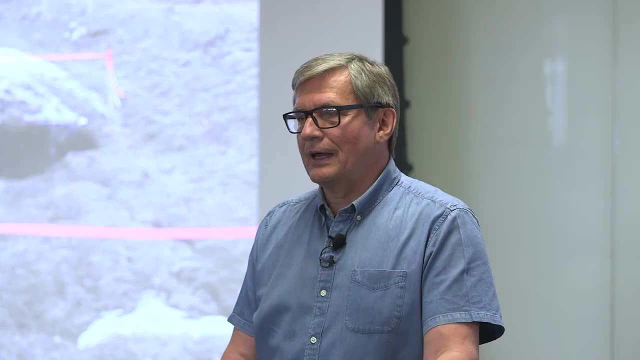 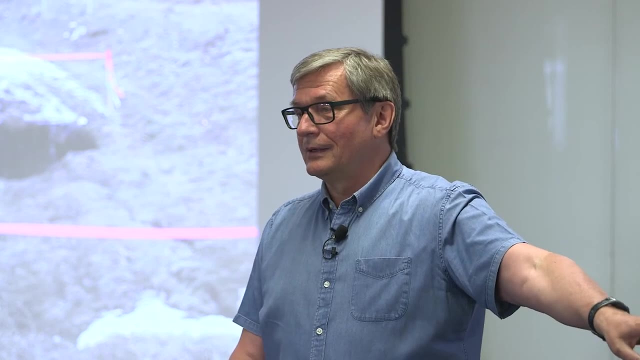 Sinkholes. it's a very good example what happened when permafrost is thawing, Most of our sinkholes. actually, permafrost thawed a little bit earlier And now they're just collapsing. So in some particular because I said it's a whole range of conditions right, And some places like what we choose. we choose actually cold places where we put our sinkholes And a lot of places have build-in sites. It's kind of typically black spruce forest with some protective organic moss layer and peat. 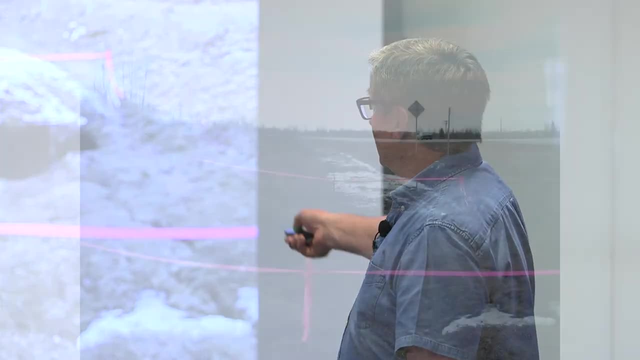 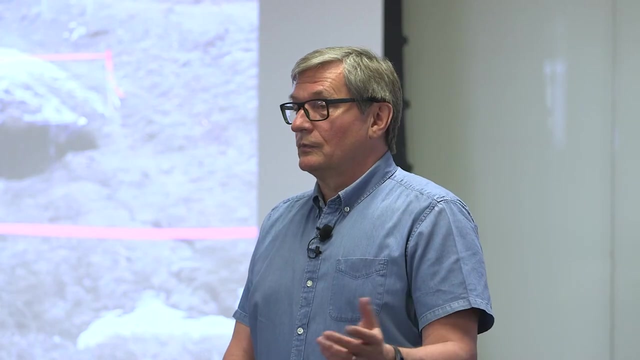 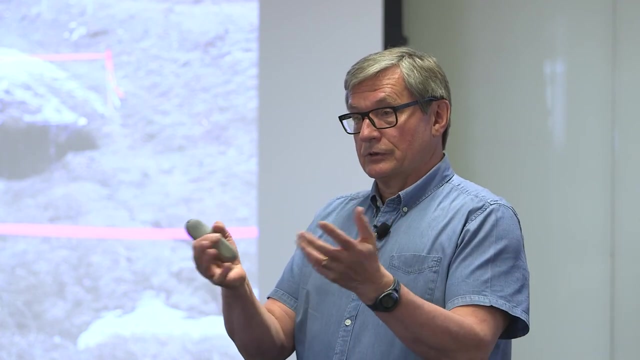 So they're more stable, But there's lots of less stable, especially on the shoulder of a road. This is the Gulf Stream Road, So there permafrost already was thawing. after construction of the road And developing this, ice was melting. 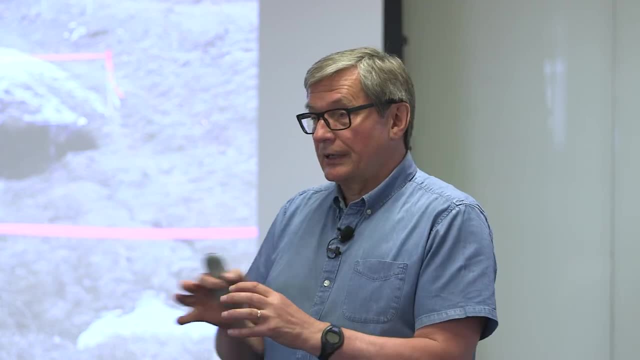 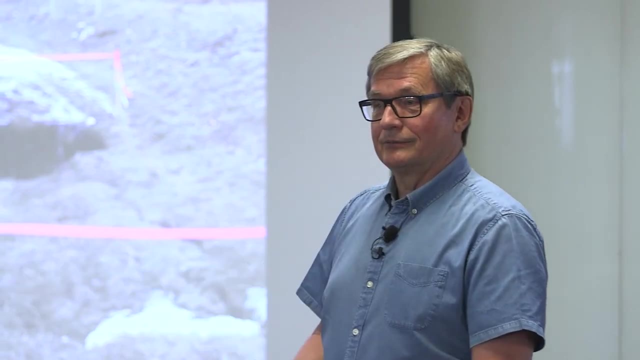 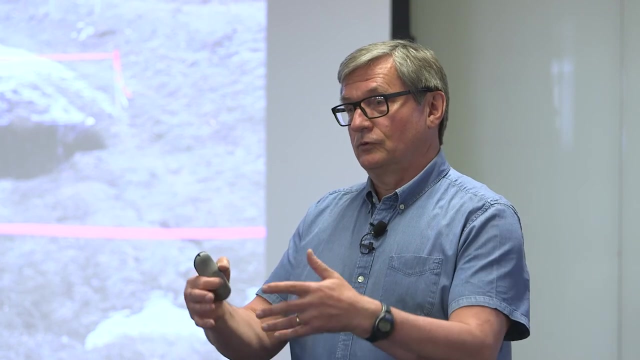 edges. It's all this kind of structure. They're connected to each other And water was just simply draining somewhere, like to cold stream, probably creek to the creek, And these voids, they devolve during some time, And usually in the spring, when this roof of these 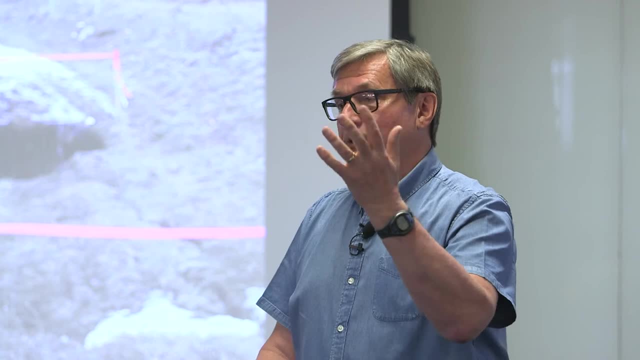 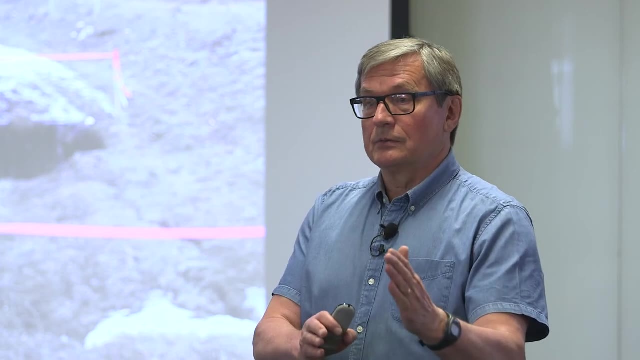 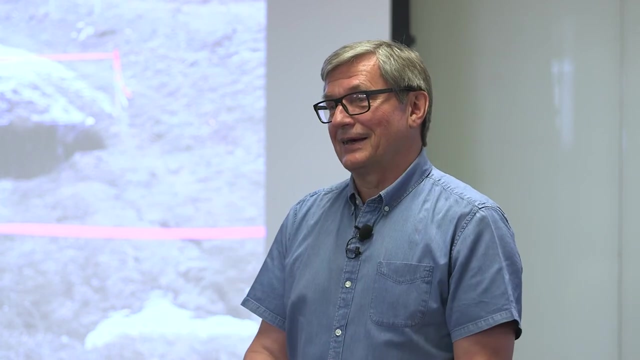 voids get not strong enough, it collapses and creates these sinkholes. But they are developing in other places more stable, in the past, right now as well. these empty volumes, We just don't see them before they collapse, But they are growing, And this latest excitement about 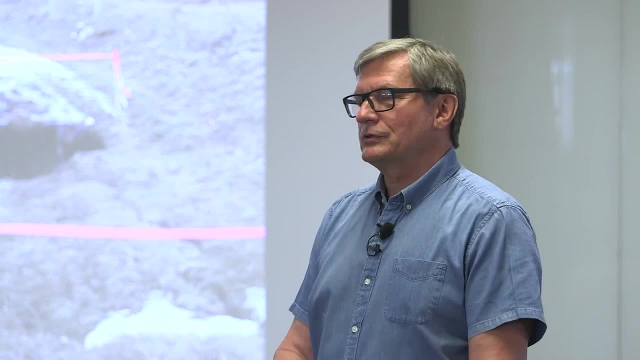 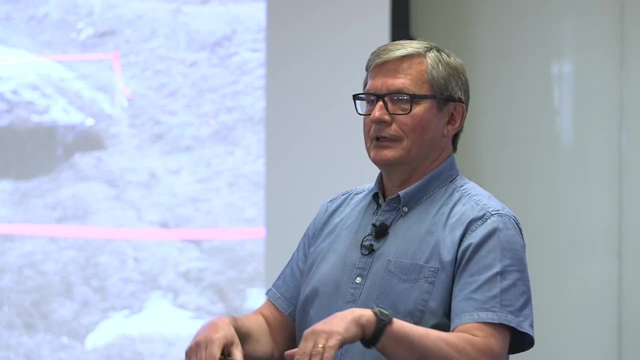 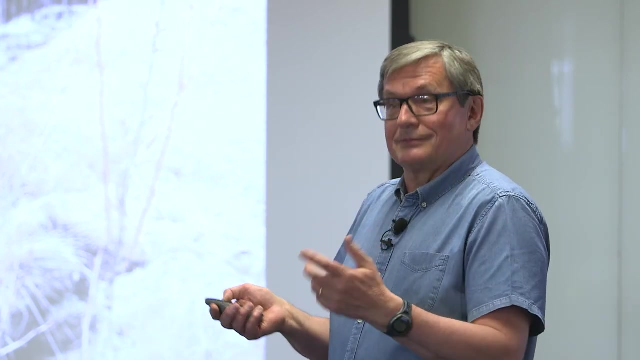 Birch Hill big one, So it was not there probably maybe 20 years ago. I mean voids. it all developed pretty recently and now it's collapsed, Water going in and disappeared, never filled, because there is some channels. 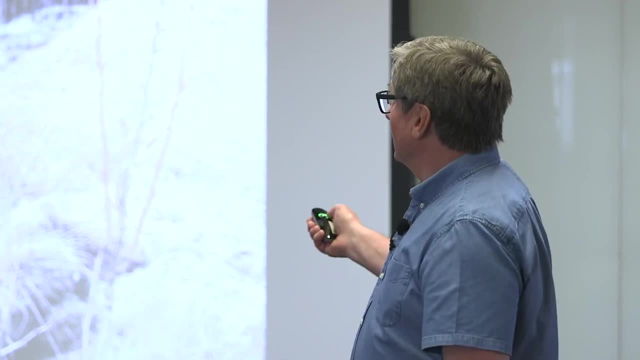 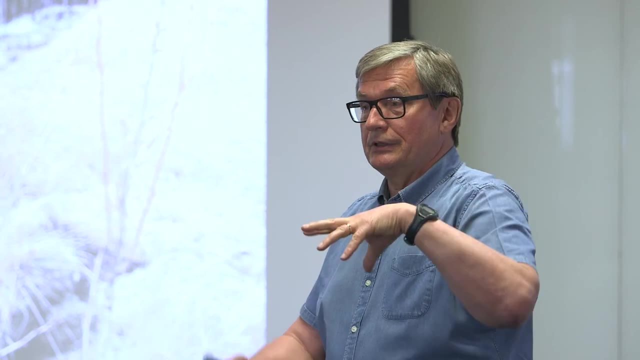 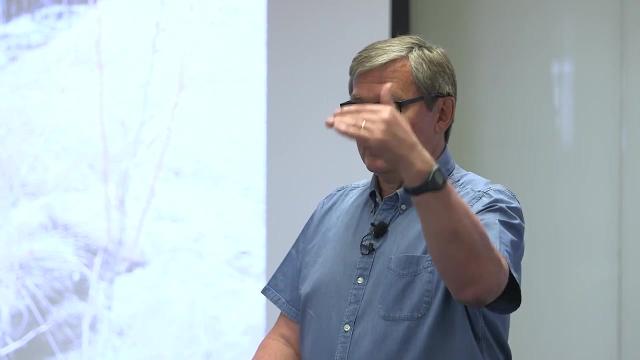 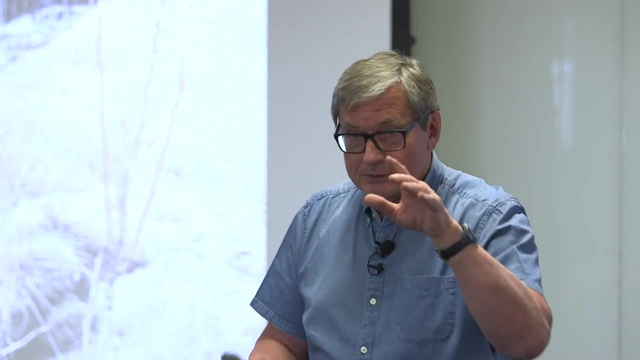 And it's not my imagination. Actually, at the Geophysical Institute, when they were building this addition to Geophysical Institute, this world called building, they dug very, very deep, deep, deep and deep excavation And we actually saw these channels there, empty channels, You can see it. 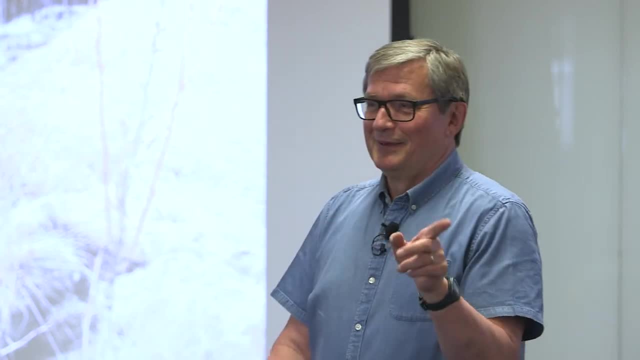 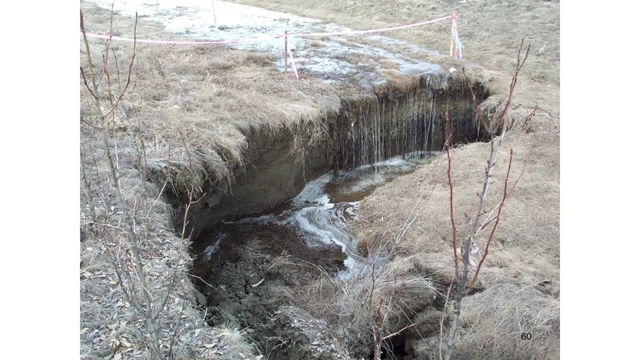 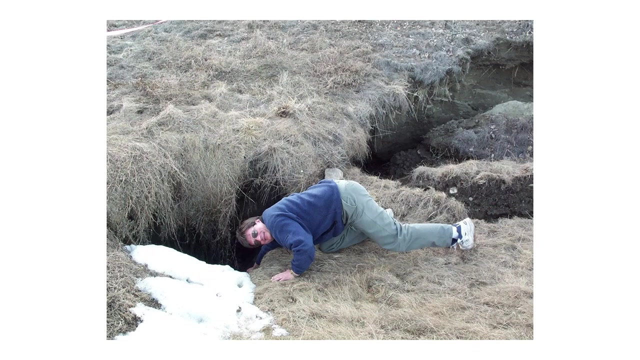 goes. Nobody was brave enough because they're not that big. Well, actually big enough for a person to get in, but better not. So yeah, it's younger me trying to reach the bottom And usually it's like: you know, you know like three meters, you know up to 20 feet. 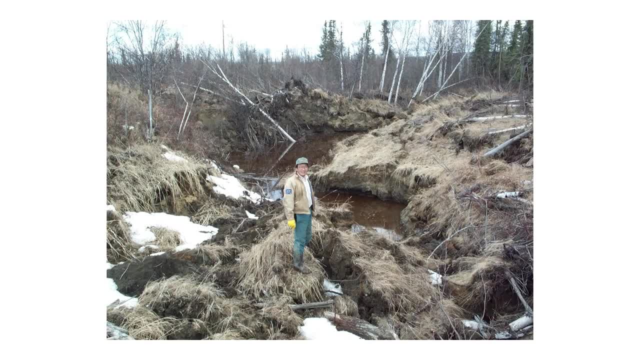 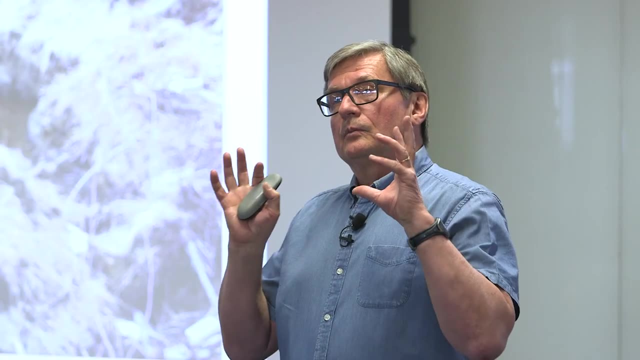 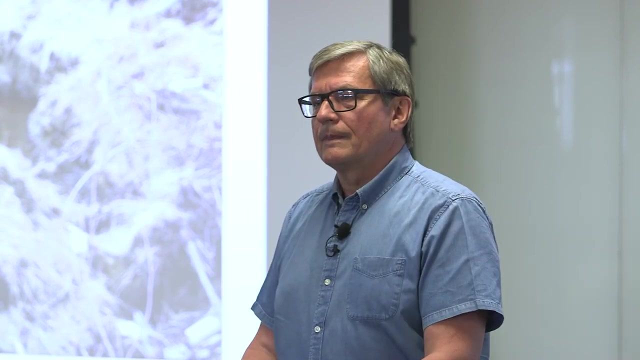 Easily Kenji again. sometimes it happen when it's big ice wedge melts. It's actually on another side of the of the Stis Highway, from that, from a pipeline exposition, Steve Reef's land- When big ice wedge close to the surface melts, it's actually 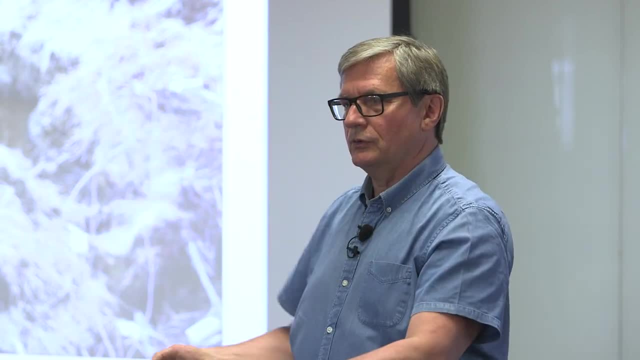 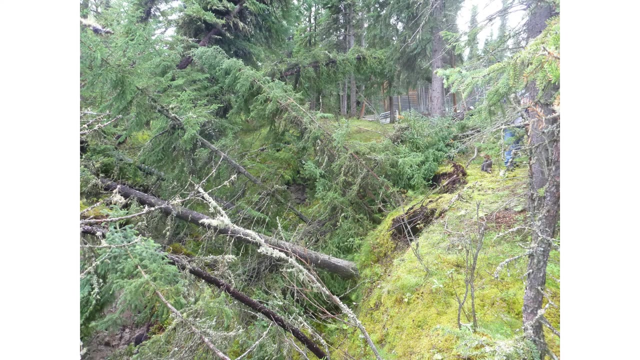 surface collapse, not just as a hole, but a whole trench, a huge trench, And we see it many, many places. That's another place, It's Miller Road extension down the hill. So that's happening, and very recently. That's a very recent thing, Fortunately for the owner. 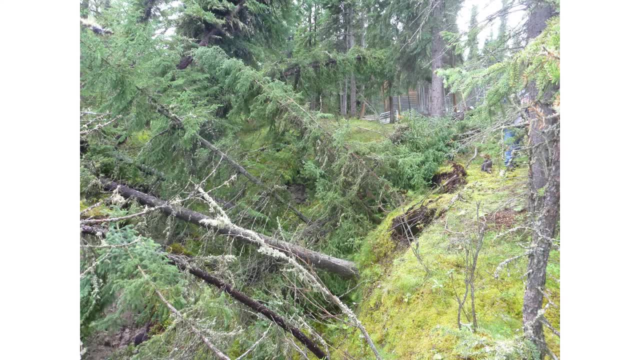 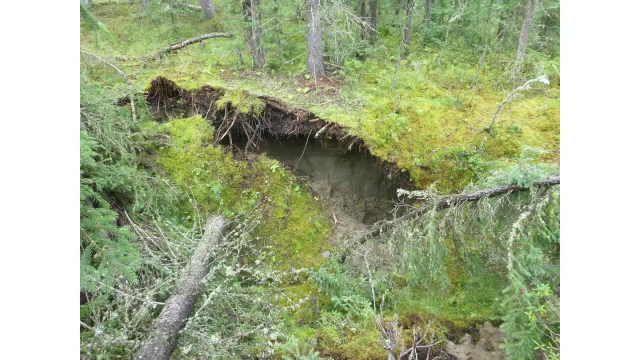 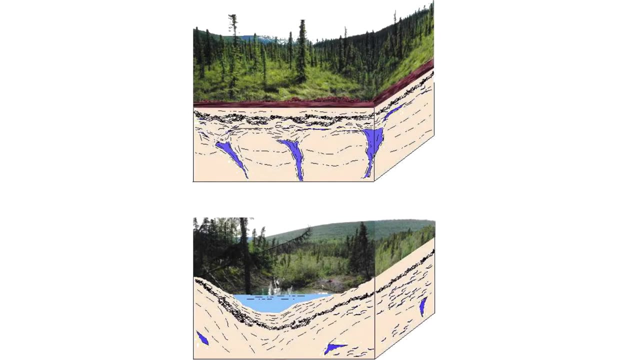 of this house. this trench happened just about maybe 20, 30 feet from his house. Yeah, that's how it looks like. Also, lakes, of course. Thermokarst lakes are cold When ice melts and there's no drainage. 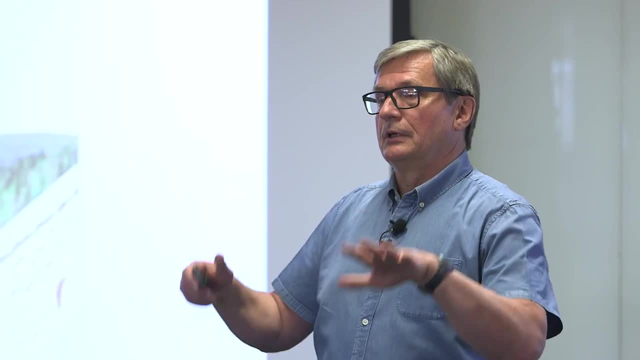 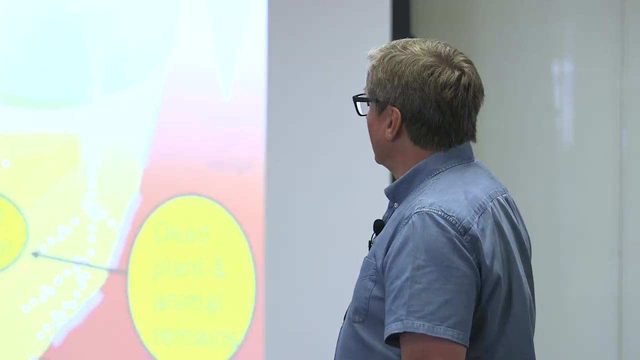 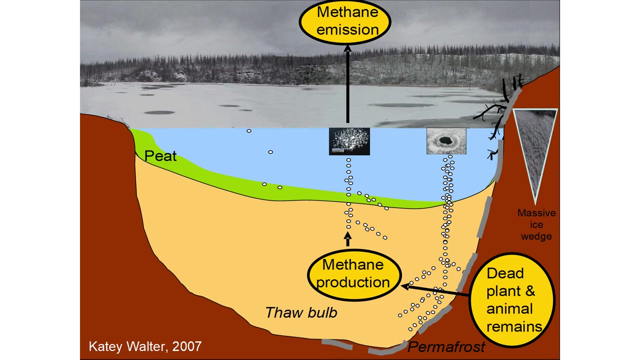 then water accumulates and subsidence creates this depression and water collects there And water of course makes permafrost So even faster. And of course there's another could be a lecture about methane coming from thawing permafrost. very, very exciting thing Actually, I think. impact on infrastructure. 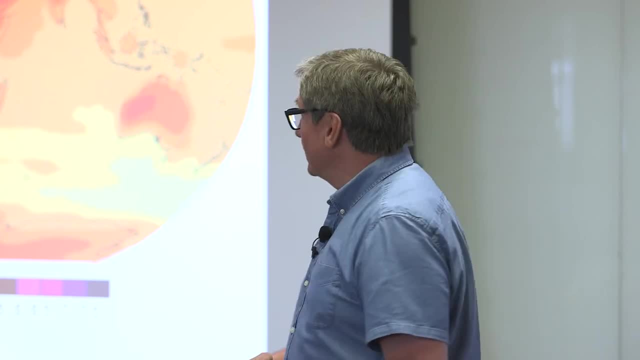 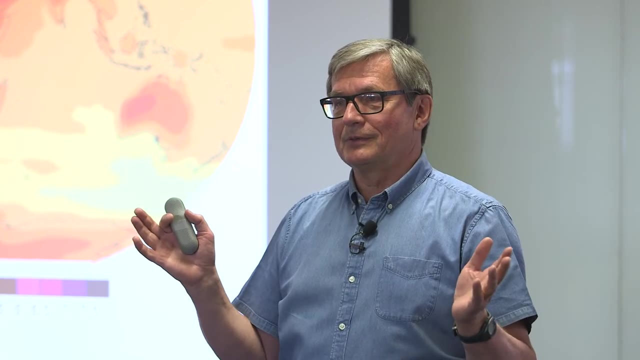 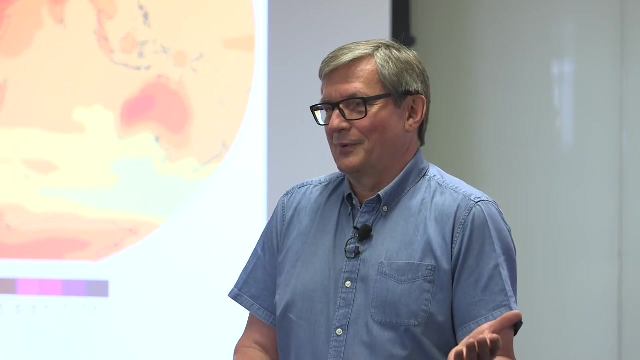 much more serious than impact on carbon. Carbon, of course, is global, So it goes out and it goes all over the place. Infrastructure: it's more local, you think. Of course, for us who live here it's maybe more important than global things, But for people who live, 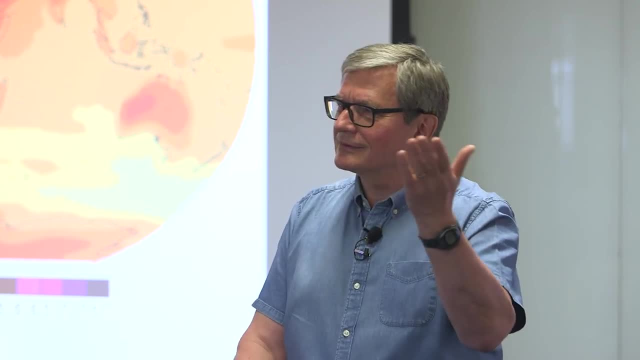 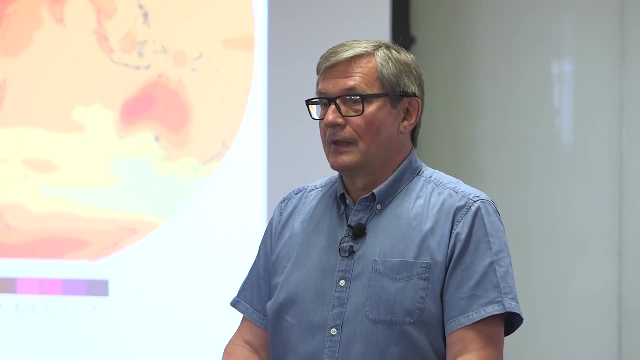 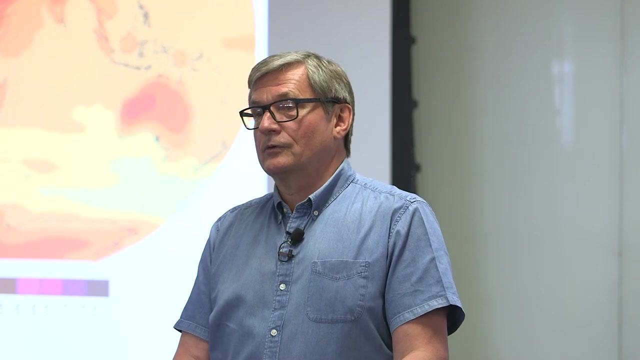 say in the low 40s. oh yeah, Alaska. And how many people there? 800,000.. It's OK, But for us of course it's much more serious. But I would argue that impact on infrastructure of thawing permafrost it could be regional. 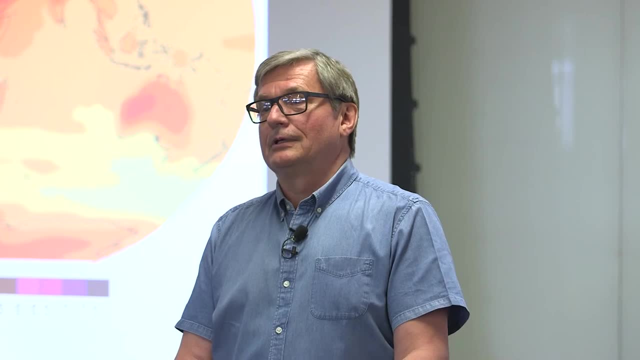 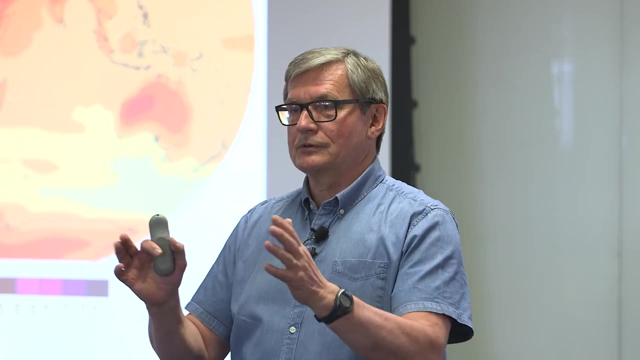 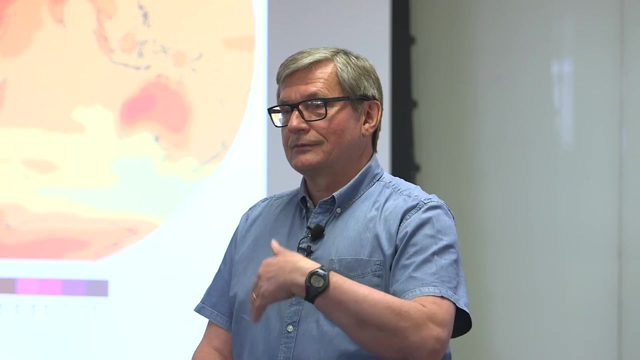 or even global A problem, Yeah, of lots of energy sources- I mean oil gas now going into the Arctic, into the permafrost, especially in Russia, but in Alaska as well, of course- And interruption of this flow of this stuff. 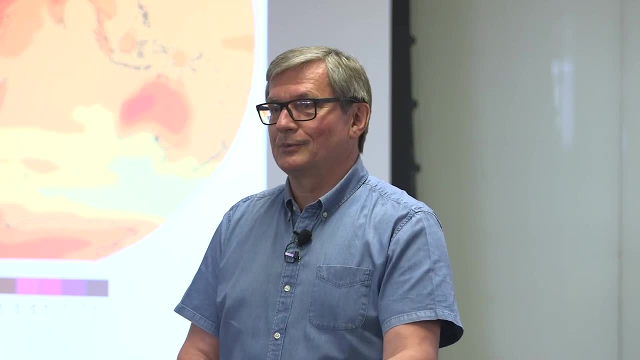 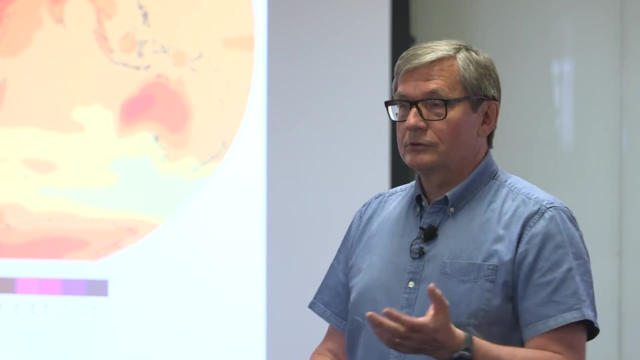 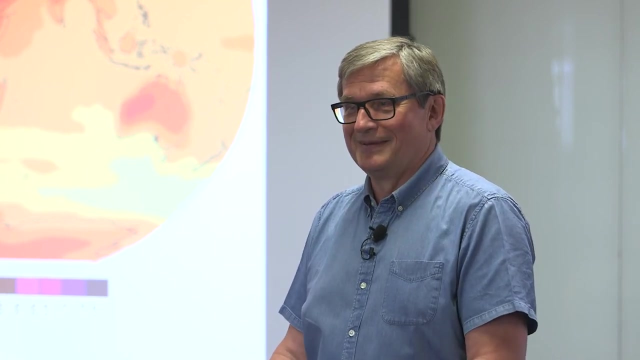 you know that it could actually have, like we have now, global consequences in terms of fuel prices. Now just a little bit to finish. What should we expect in the future? Very kind of briefly, Well, all bad news, Of course. all this bad news based on modeling. 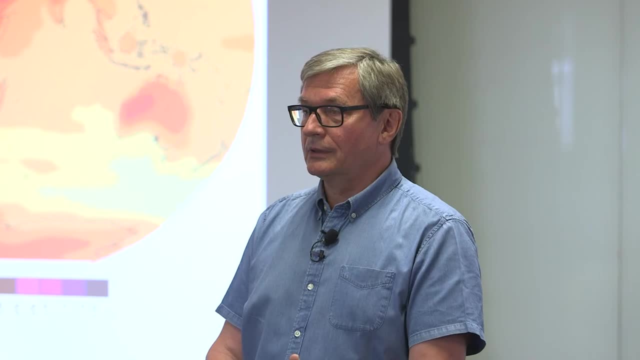 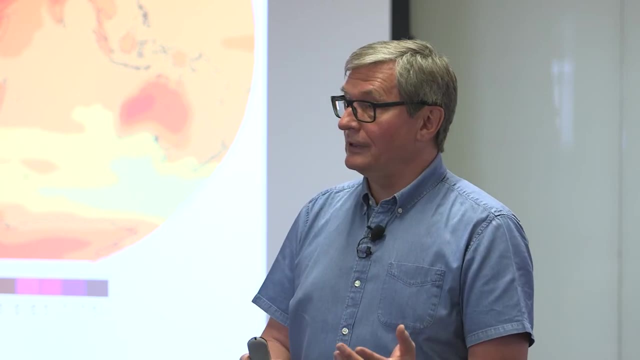 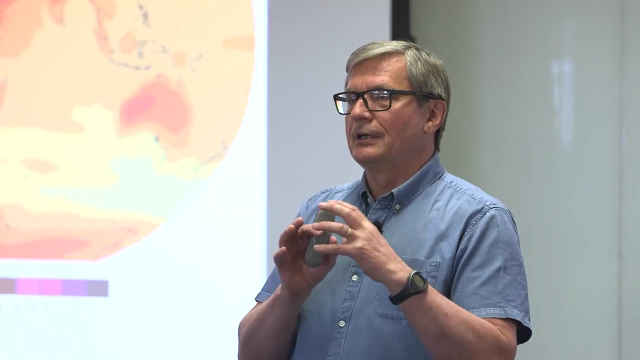 climate models and some people believe more in them, some people believe less. But, like my simple model, if everything will stay the same and everything will be changing, like have been changing during the previous 35 years, which we observe, then we should expect: 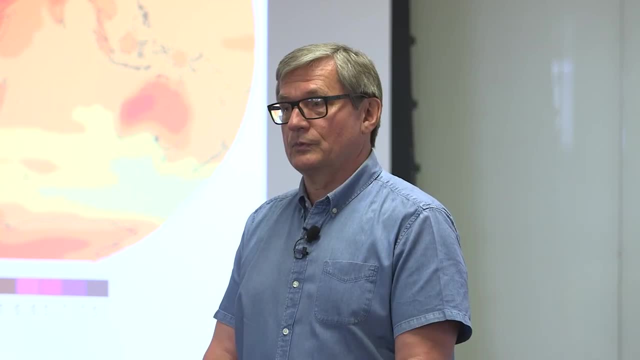 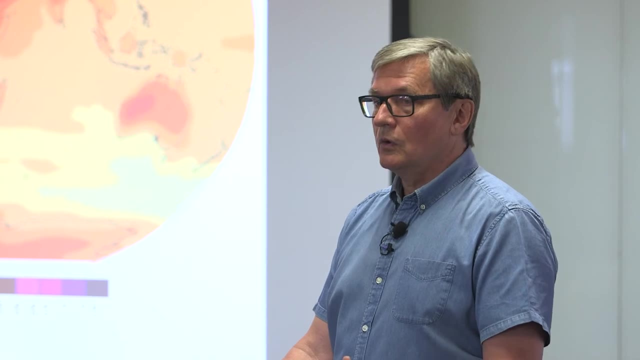 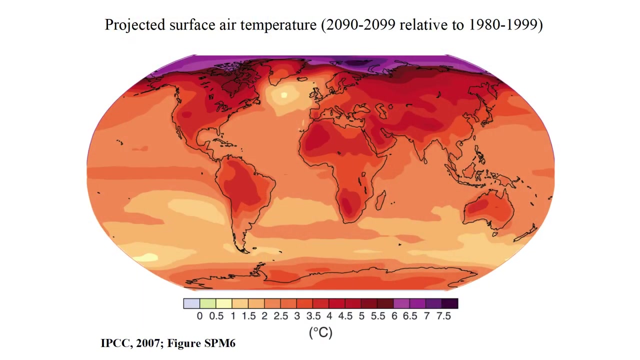 significant warming in the future as well. It could be wrong, of course, because linear interpolation of present day climate is not a good thing to do, but pretty much all climate models show that it should be warming anyway. So that's one of them and shows that. 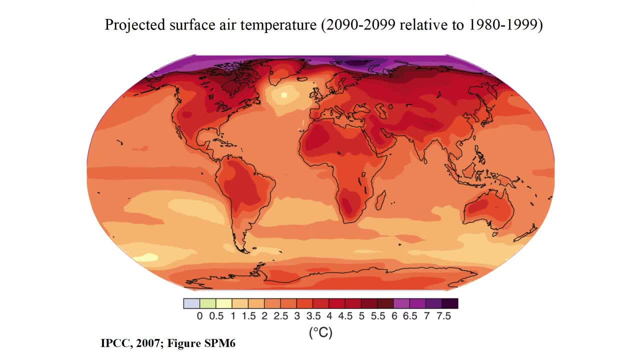 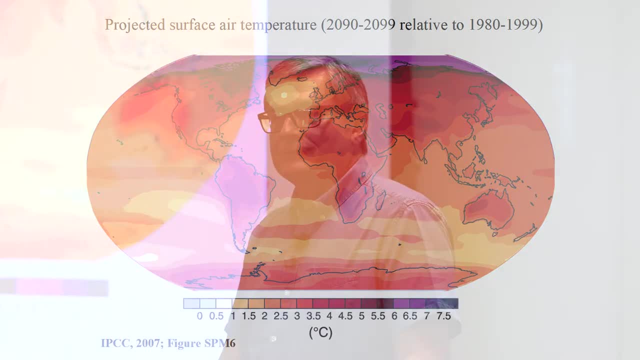 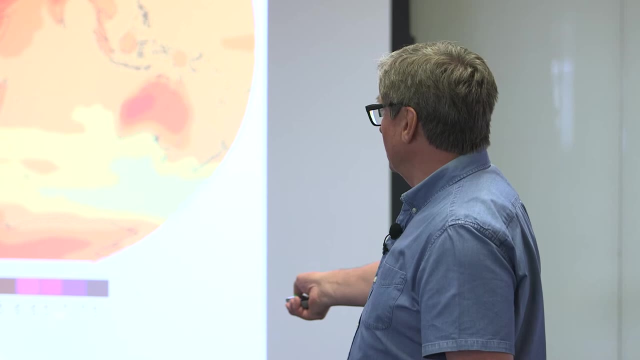 look at these numbers and this Celsius, so we should expect warming in the interior somewhere like four degrees, five degrees, so like seven, eight degrees Fahrenheit warming by the end of the century And in higher latitudes on the North Slope. 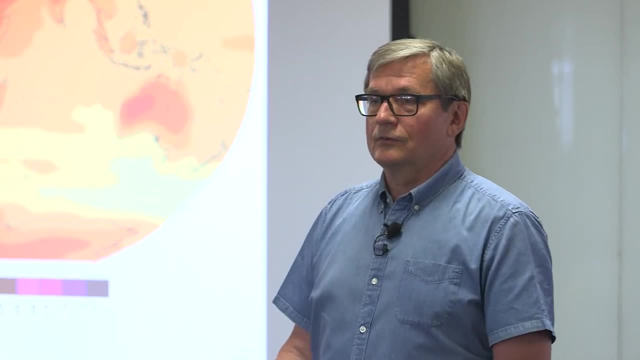 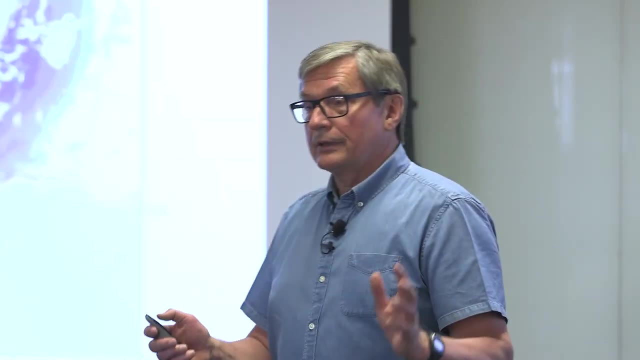 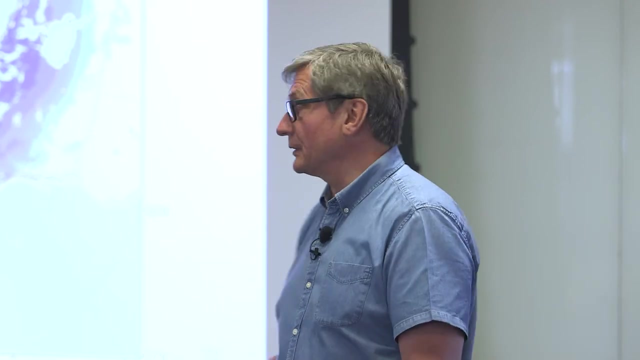 even more serious numbers. So of course, permafrost will react on that And we do some modeling, like I said, and I will show just a few examples of this modeling: in a global scale, in Alaska scale. So, going in one of our models, 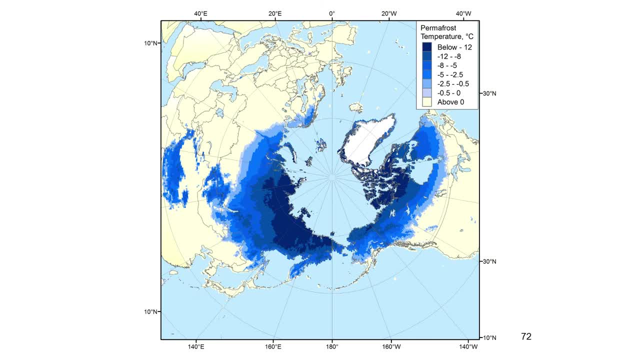 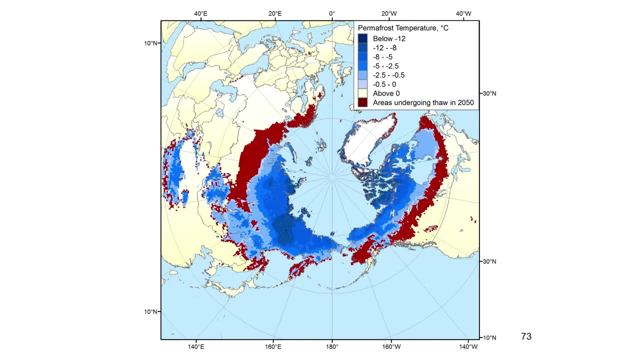 that's what we should expect. So it's present day conditions, distribution of permafrost in the northern hemisphere By 2050, all of this red where permafrost will be thawing. So it's kind of simplified model. 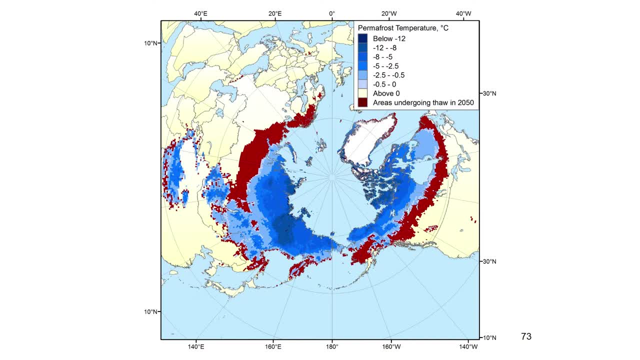 but even this simplified model shows that by 2050, interior will be pretty much thawing, Which actually, based on our data, it makes sense. And by the end of the century, by 2050, basically all kind of permafrost inсте is thawing. So this kind of simplified model- but even this simplified model shows that by 2050, interior will be pretty much thawing, Which, based on our data, it makes sense. And by the end of the century, 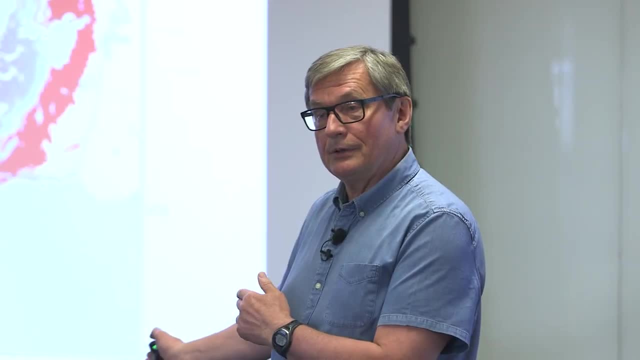 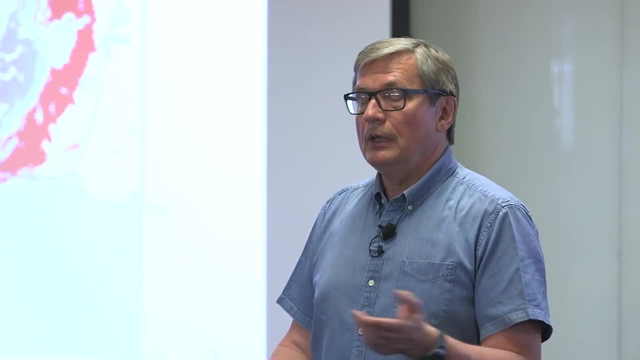 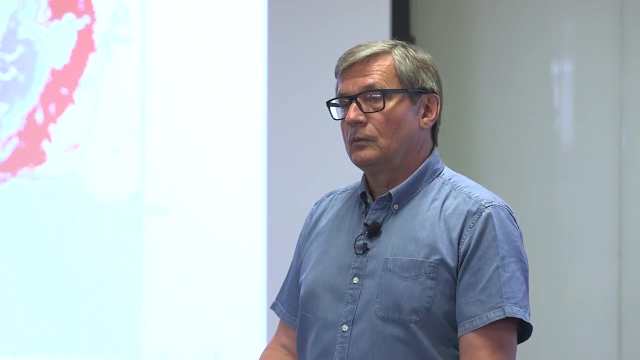 only North Slope and this simple model permafrost. it looks like still stable. However, our other more advanced models and actually warming scenario here was not extreme scenario, It was kind of average scenario. But in our more advanced models and more aggressive scenario, 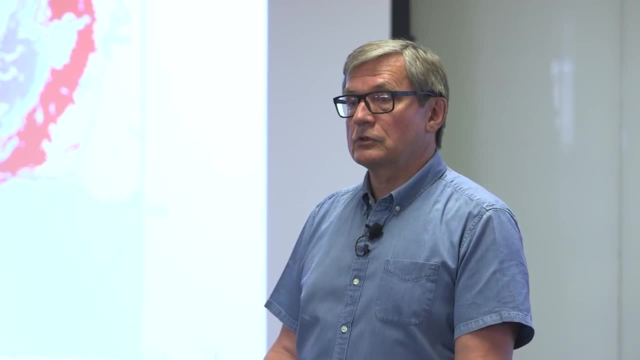 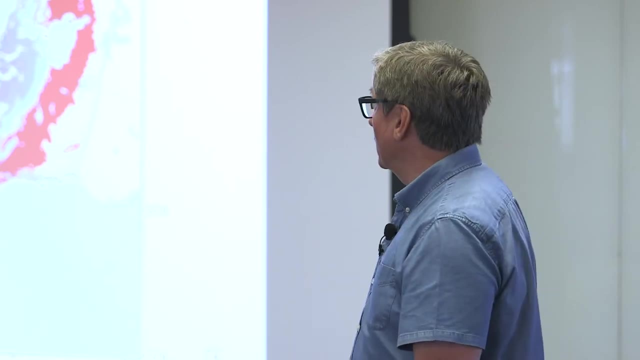 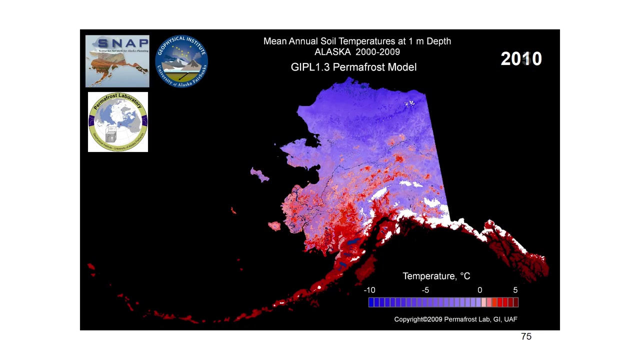 warming scenario. it shows that many places on the North Slope permafrost will be thawing Again. in agreement with my simple straight line model In Alaska itself- this is one kilometer resolution model- Shows that about mid-century again Here. we already see that. 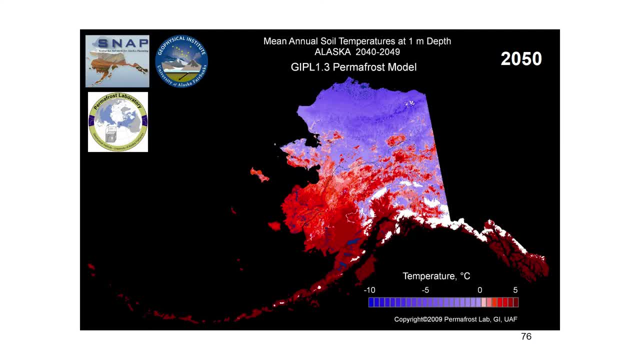 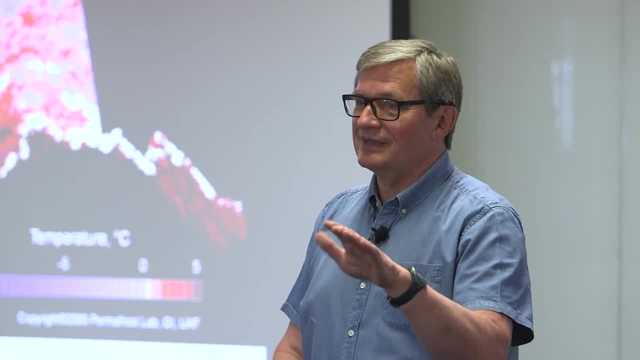 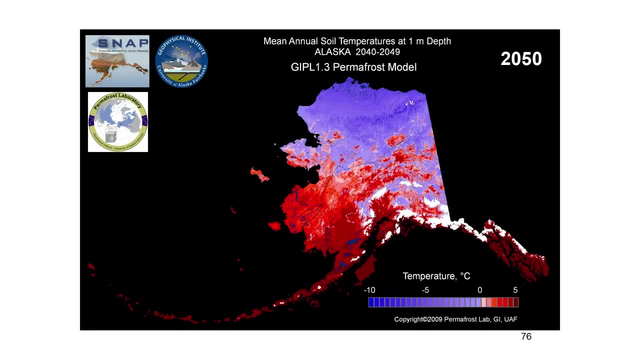 not that homogeneously disappearing. So there is some conditions where surface and vegetation and some conditions where permafrost is still more or less stable, Not really almost dying, but still. It's still there. But in most places it will be gone, And again by the end of the 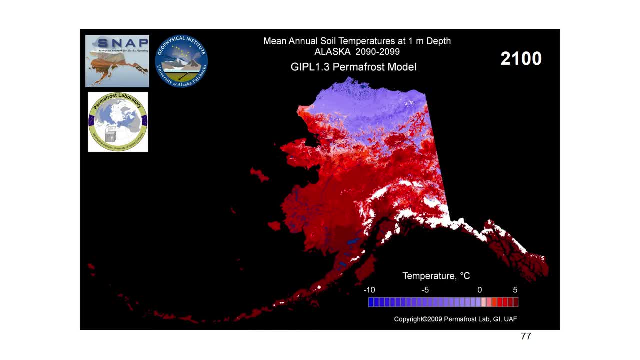 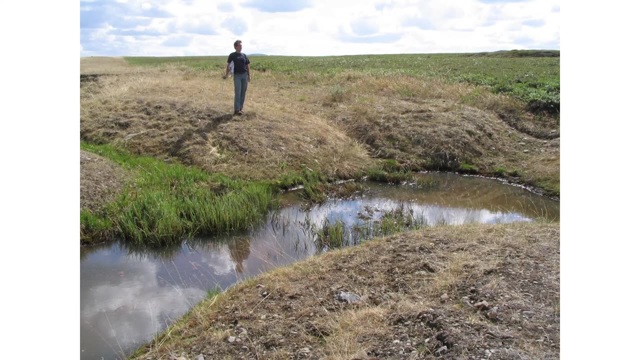 century only Brooks Range and North Slope. according to this model, which is not really extreme warming model, permafrost may be stable And of course there's consequences everywhere on the North Slope in interior for infrastructure. Now I'm talking about infrastructure will. 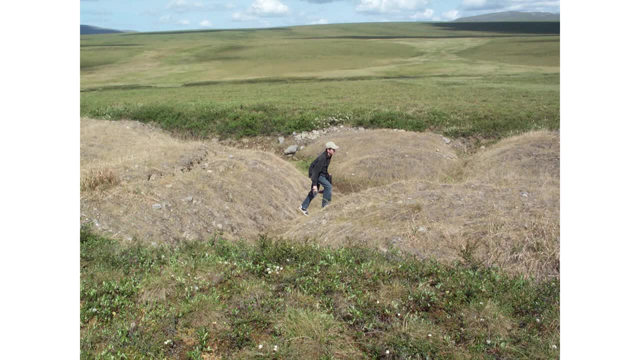 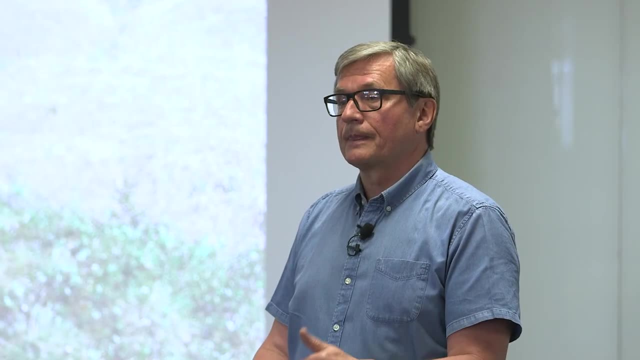 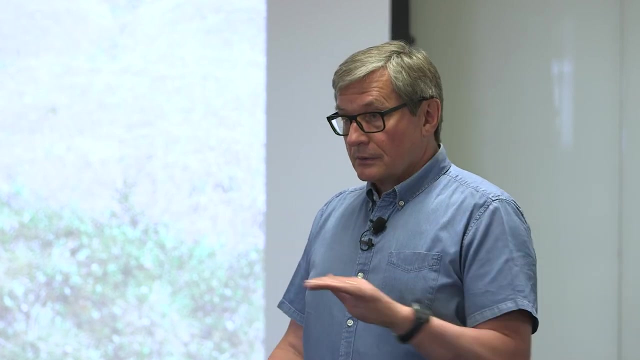 be severe. So this is access road to the material side. It was built during the construction of Dalton Highway and Aliaska Pipeline. It was used that time, about 50 years ago also, And then after that it was not used, And that's what happened to the road, if you just 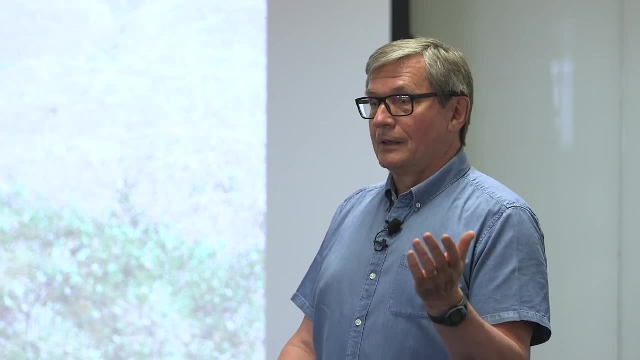 leave it like this. It's in a relatively cold permafrost. So I'm saying that if our permafrost is not used, it's not going to be stable. If it's not going to be stable, it's not going to be stable. If it's not going to be stable, it's not going to be stable. 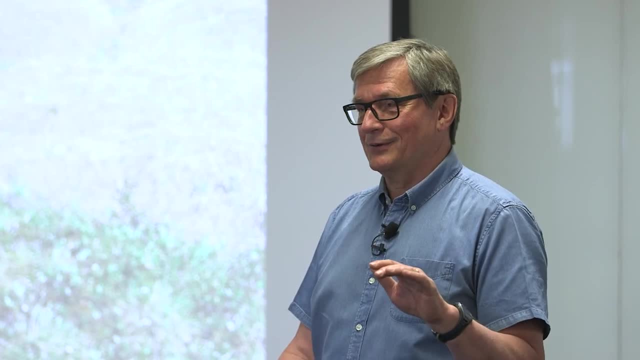 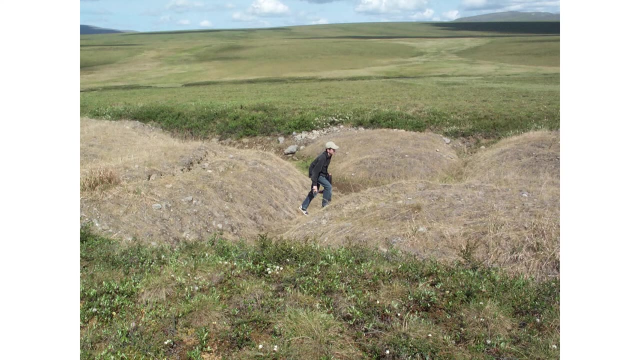 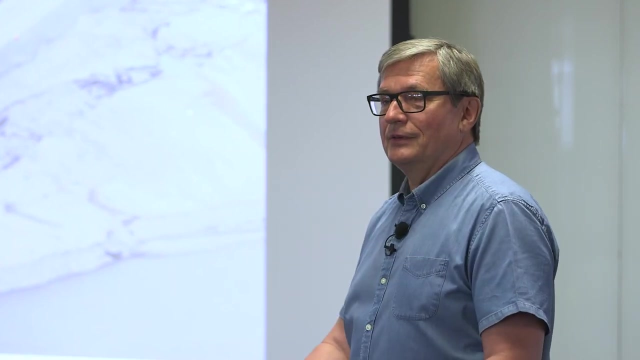 Our Department of Transportation will just give up on our roads. All our roads will look like this in about 15 years at maximum. Yeah, like this Good example. it was 2015 flood at Deadhorse- I mean Prudhoe And, of course, permafrost. 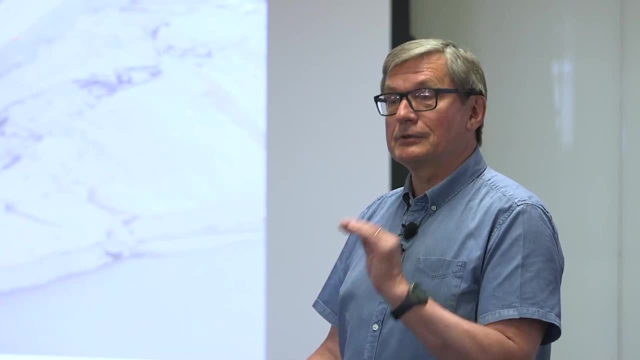 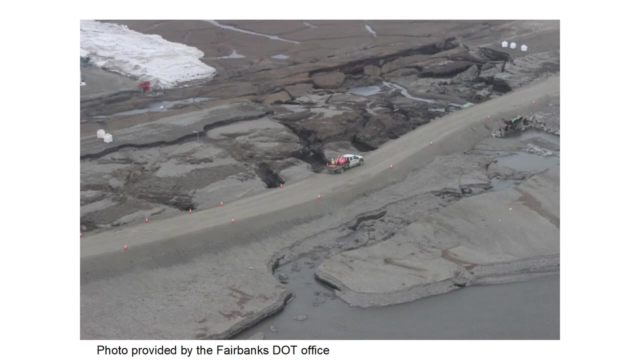 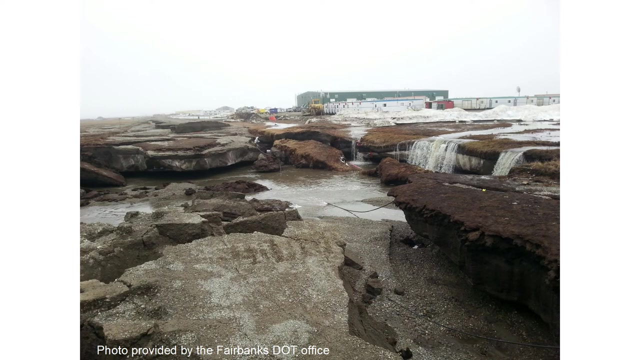 was thawed and ice melted because of this flood, But you can imagine. you can imagine what will happen if it will happen just without any disturbances, any water, just climate. It will happen the same. See, this is Dalton Highway, this one, That's Dalton Highway. 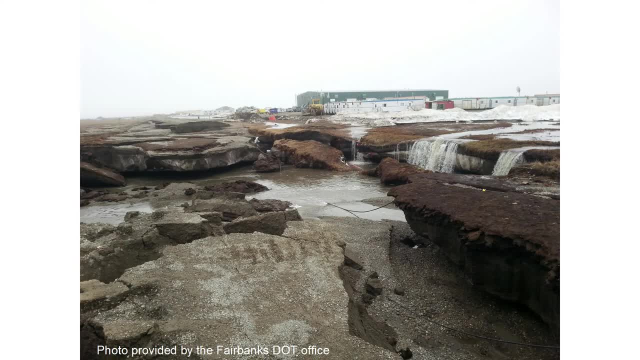 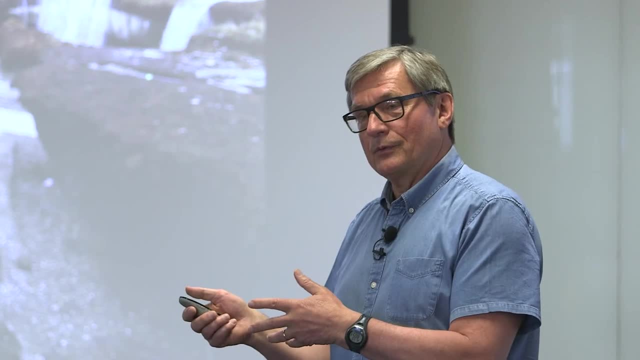 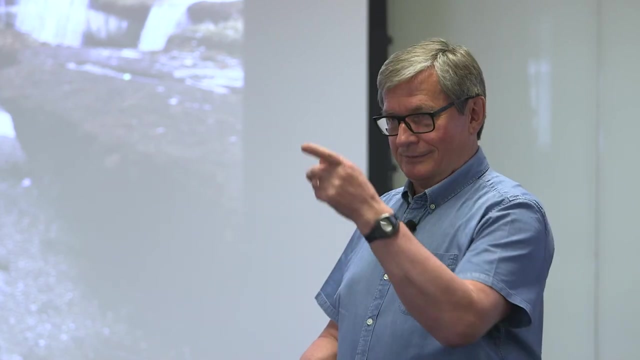 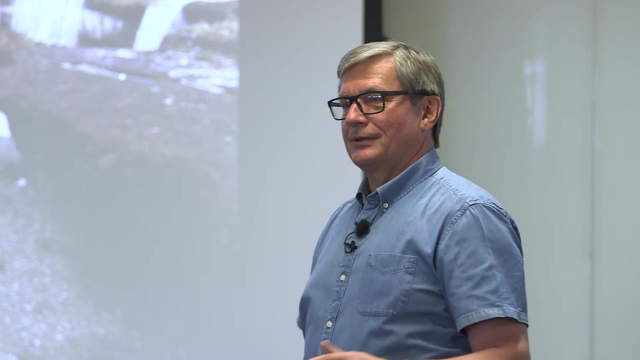 what happened to it? Of course, flooding is kind of very short impact and severe Long-term thawing. there will be some time to fix to fill Like somewhere here and around Fairbanks. asphalt layers are already like three meters, four meters thick, just filling, filling, filling, filling. 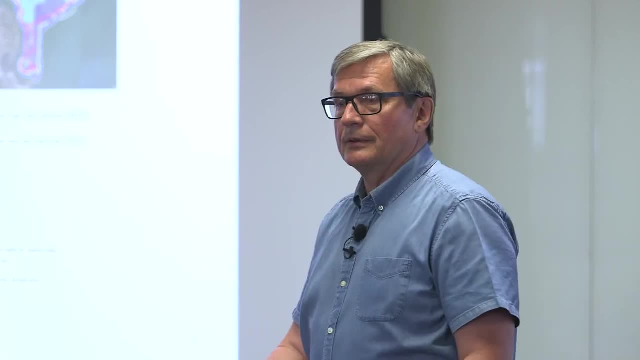 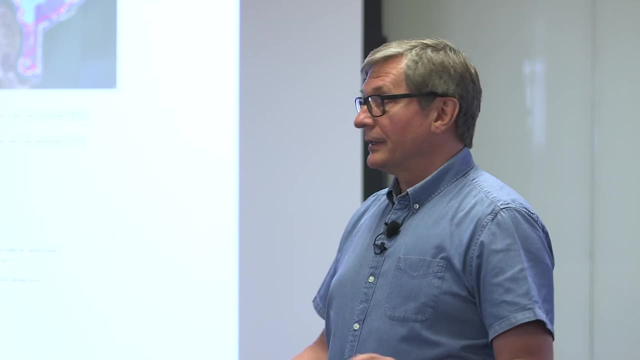 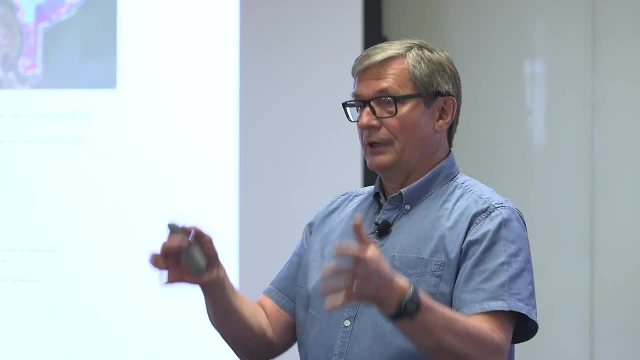 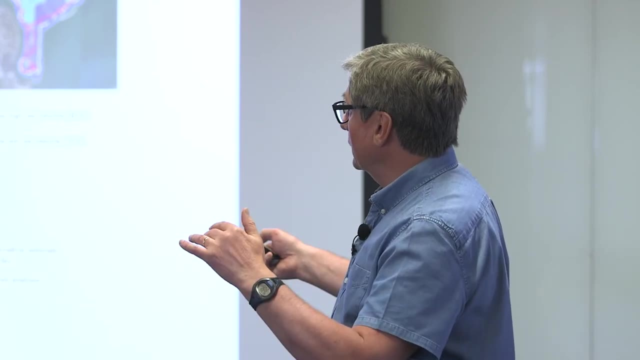 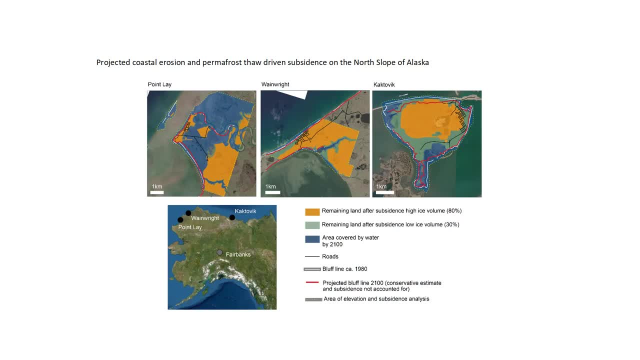 by water. So orange is what will be left of land at the end of the century. So it is potentially very dangerous, of course, because they will justwater, because they would just be losing land, Not because of coastal erosion. Coastal erosion, of course there. 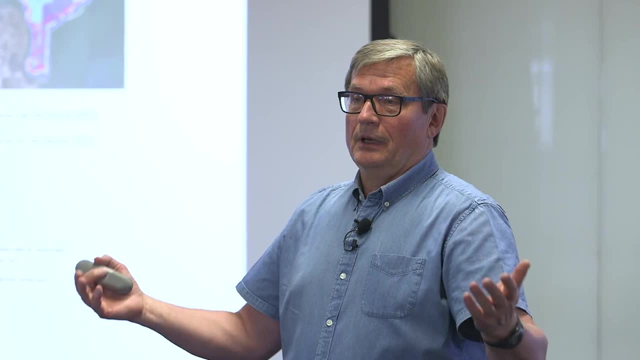 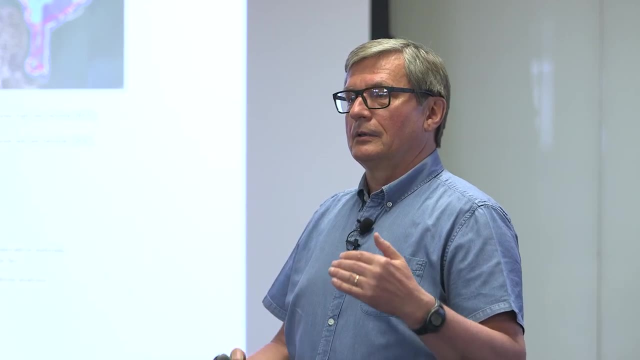 But coastal erosion maximum will be, like I don't know, one, two meters per year. Sometimes, of course, with big storm it could be more, But we're still talking about 10 meters. You know it, could you know. 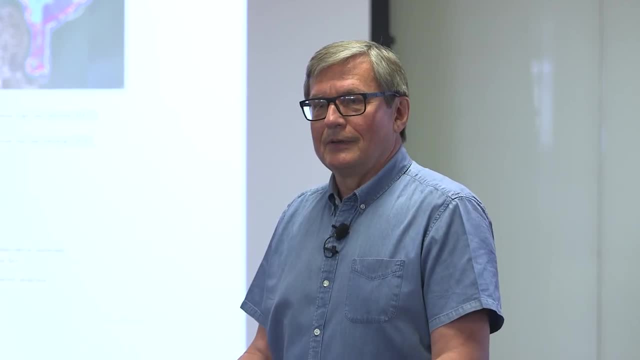 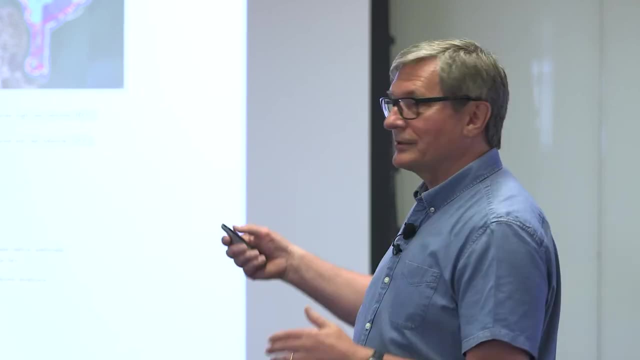 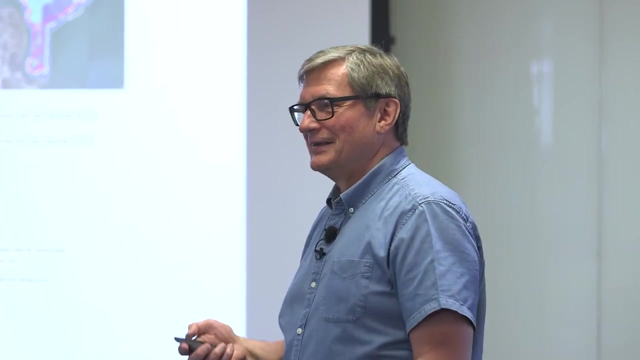 100 meters per century. Here it's. everything goes down and water from well. of course it's possible to build dams, like in Netherlands. You know, keep building and live below the sea level. I don't know, All right. 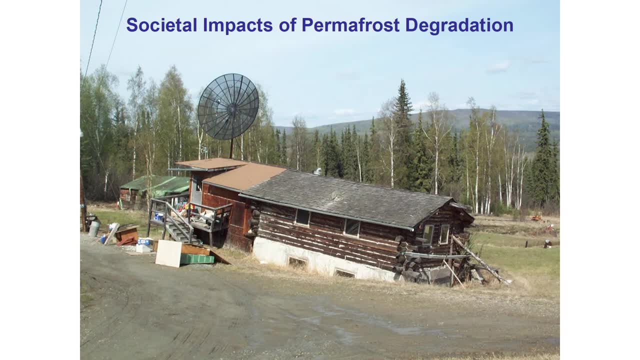 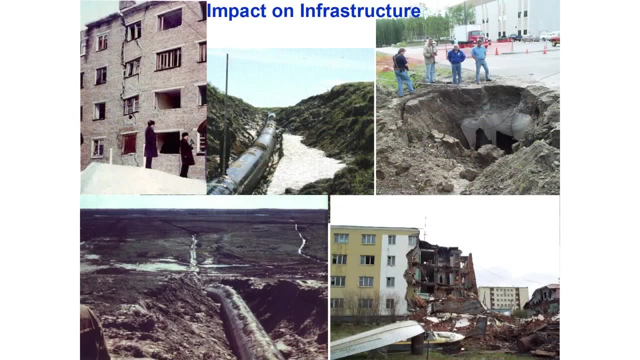 And just a few. that's Fairbanks Very famous house. It's still there. Of course, nobody lives there, but this is behind Geophysical Institute. This is Russia, also Russia. And in the end, what I would say, 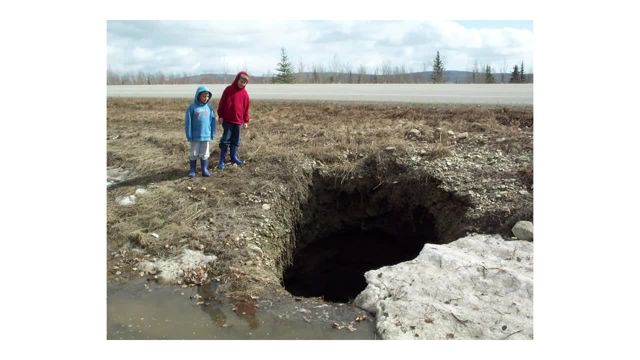 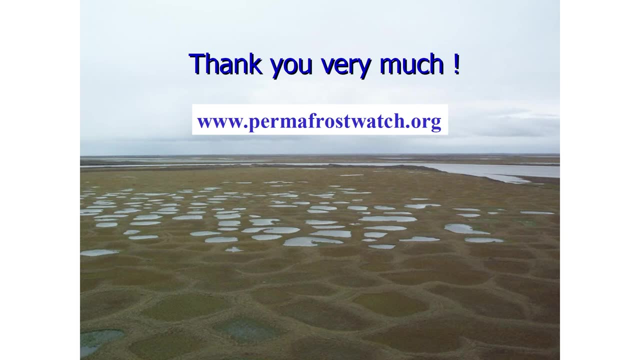 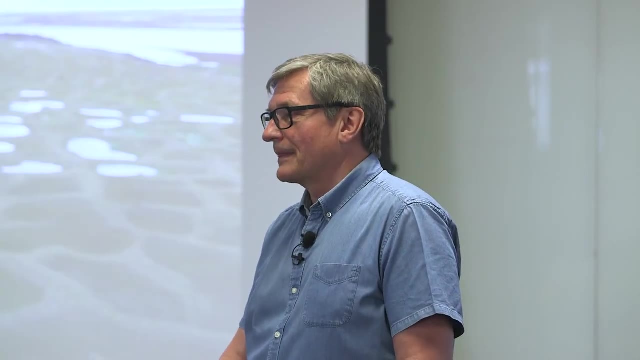 little kids, little problems, and bigger kids, bigger problems. So thank you very much, And much more information about our work could be found in. you know can easily remember promofrostwatchorg. Thank you, Do you have something sinking? 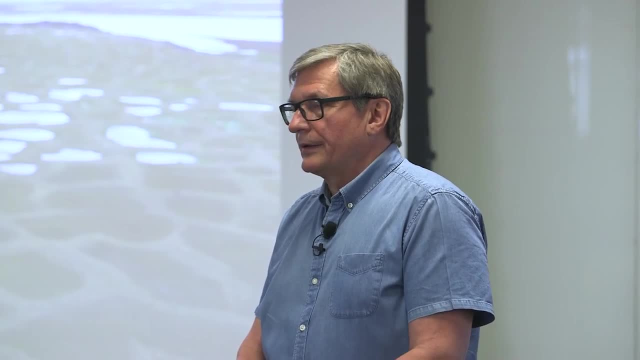 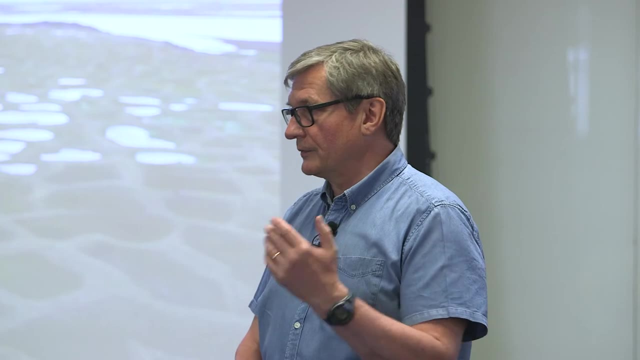 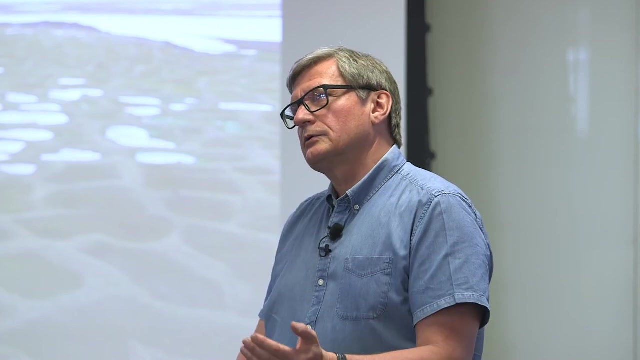 or are the heat exchangers, you know? keeping up with the issue. Yeah, The Alieska pipeline was designed with big kind of, let's say I would say better so with already assuming that promofrost could be unstable. 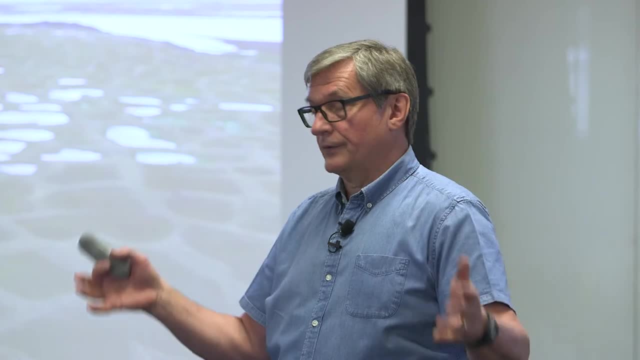 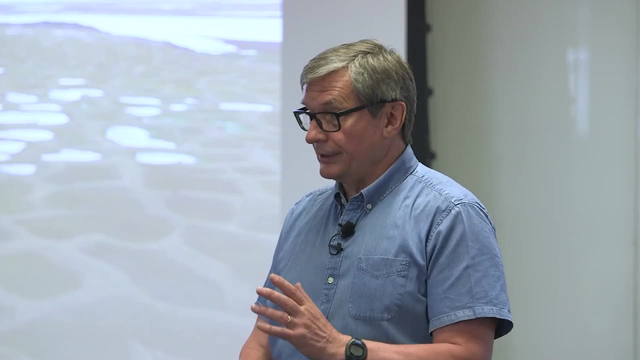 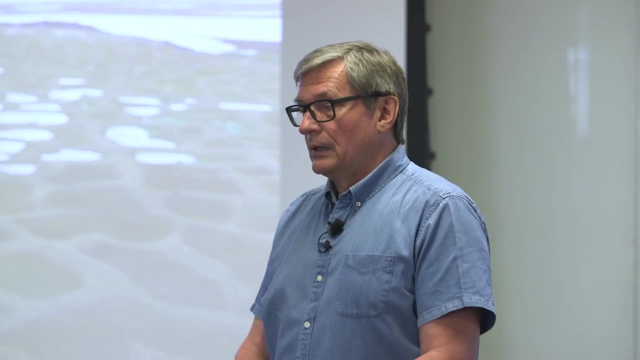 especially because of construction And these thermal piles. it's not just support members, they're actually refrigerators, without any energy, of course, but it's very, very nice engineering design. You don't need energy to make them run, So make situation much more stable. 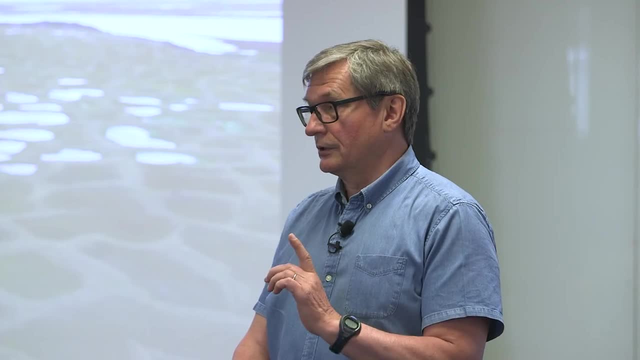 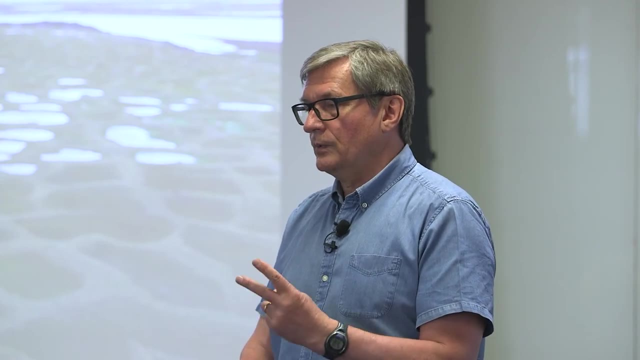 So so far there was no major problems major. There's lots of small problems constantly and they are addressing it all the time. But problem is two problems here In the future. so first of all you keep promofrost. 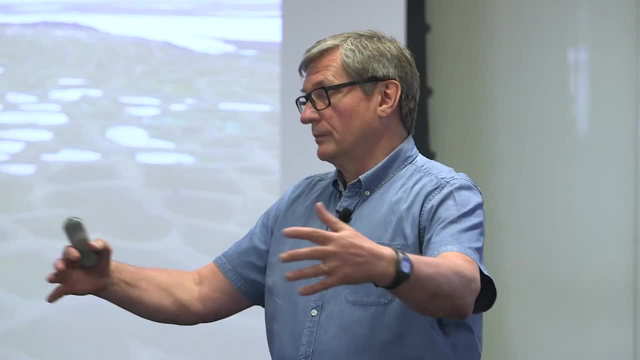 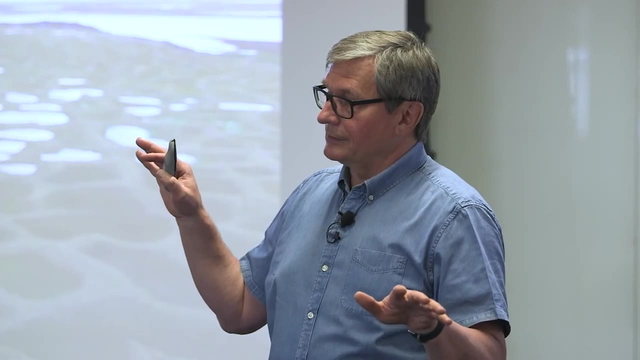 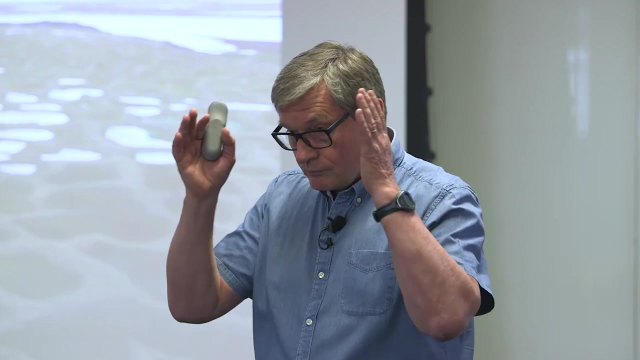 around this refrigerators or thermal piles, but it disappearing everywhere from landscape And especially in the slope area, slope getting unstable and you cannot do anything with just refrigerating your route, pipeline route. So that's a big problem. That's it's. 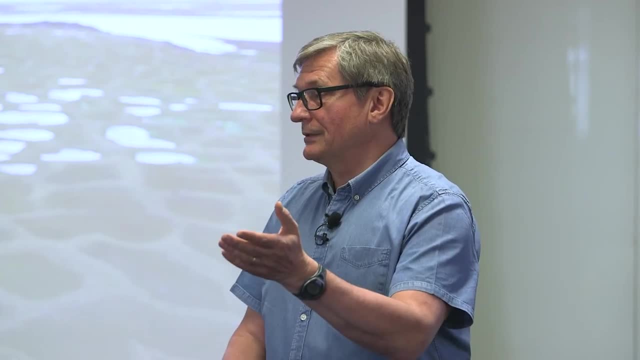 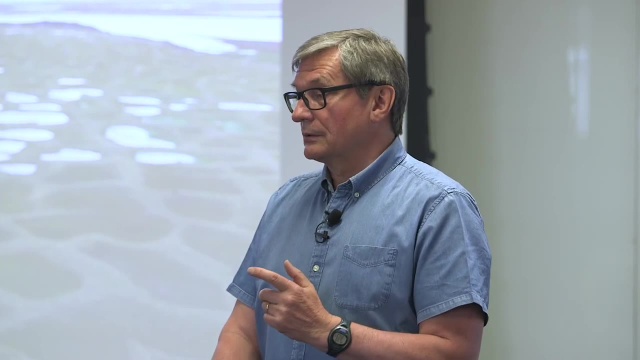 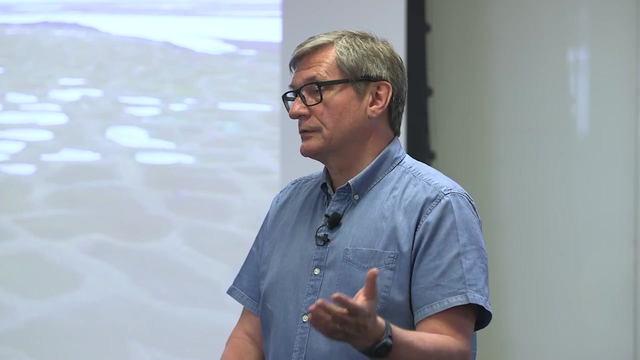 it will, it cannot, it can't be addressed as easy- well, expensive, but still easy for for this local cooling. Second, also serious problem: that winter's getting less cold So we don't have much more of this minus 40 degrees. like two weeks, three weeks month. It's already shorter And and because of that the efficiency of the cooling also decreasing. So just it's simply warmer winters, the same piles not cooling as effectively as it was during the design and so far. 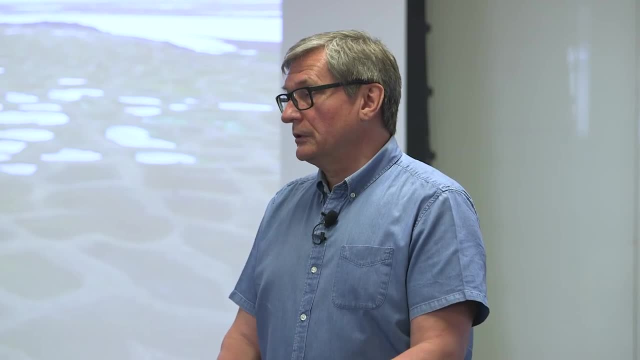 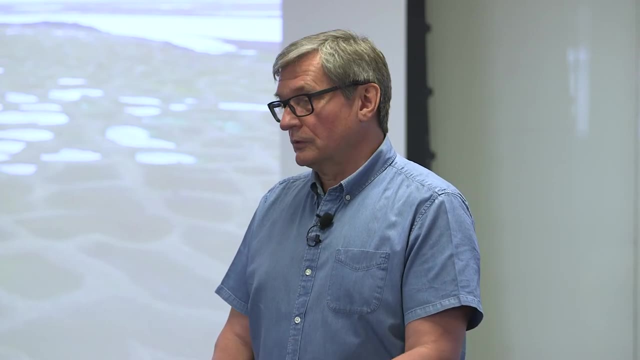 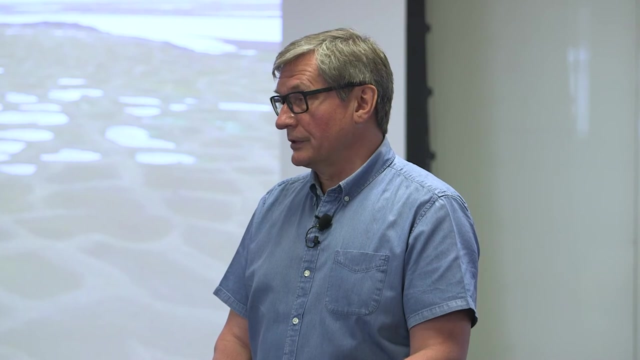 So future will, yeah, bring more and more problems. However, like I said, it was designed very well. Actually, also very interesting story because when first, the company who was designing it was from Texas, And, of course, what they do. 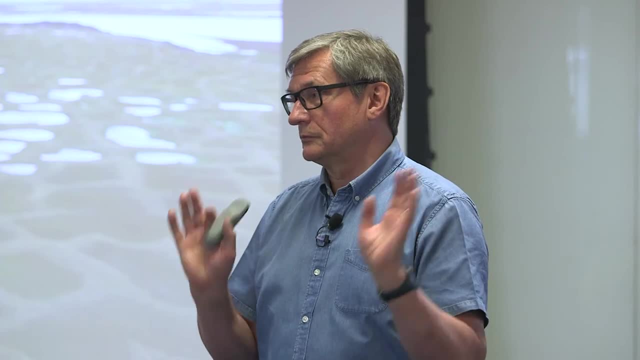 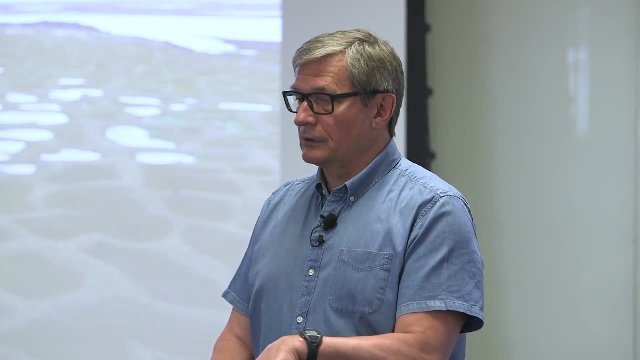 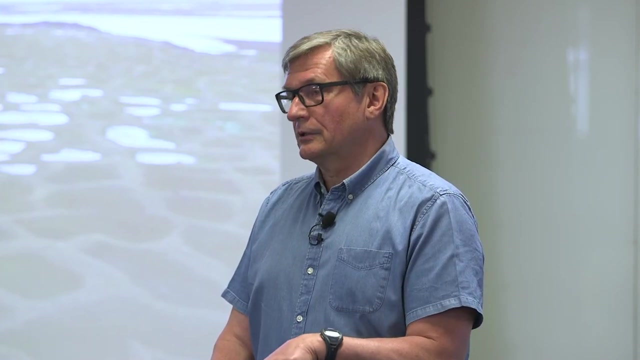 they just dig the trench And put the pipe And you know no problem And fortunately that's the. their proposal came to through this environmental assessment, through USGS, US Geophysical Geological Survey, And it was Art Lockenbrook. 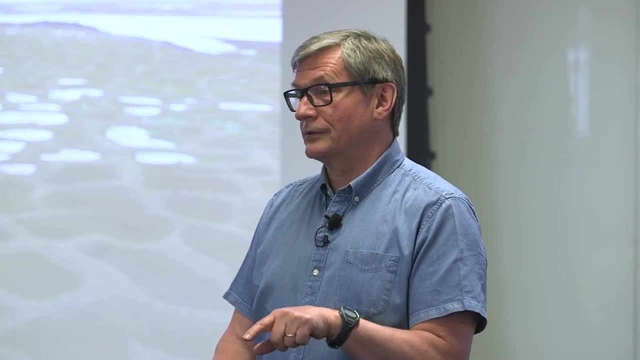 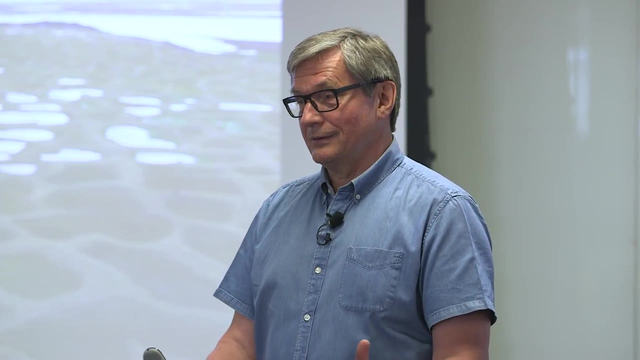 He's actually a very, very famous scientist. He's kind of one of the fathers of permafrost research in the United States. So it actually came on his desk And he looked at it and he said and he wrote just like: 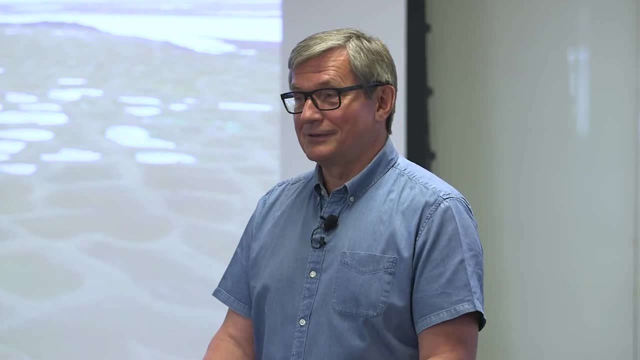 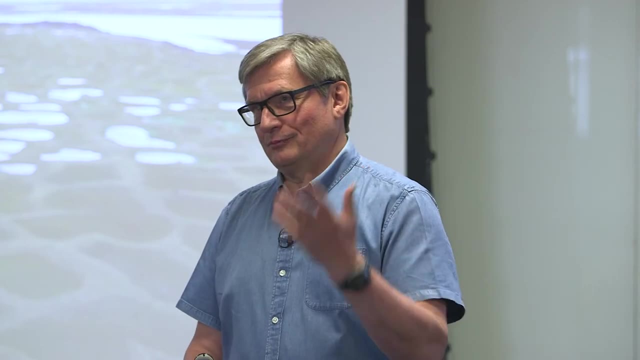 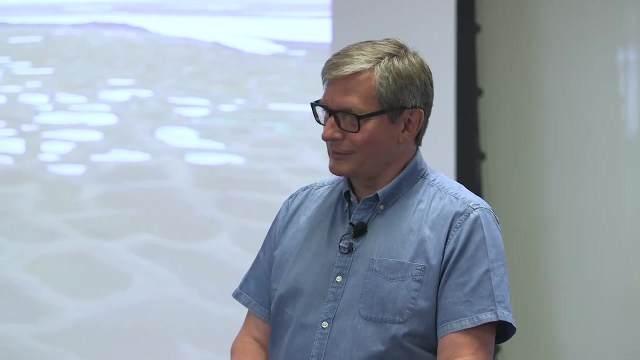 two and a half or three pages of review And pretty much it says: are you crazy? And fortunately the you know government was, you know, brave enough to make this cost of this pipeline like two and a half you know more expensive. 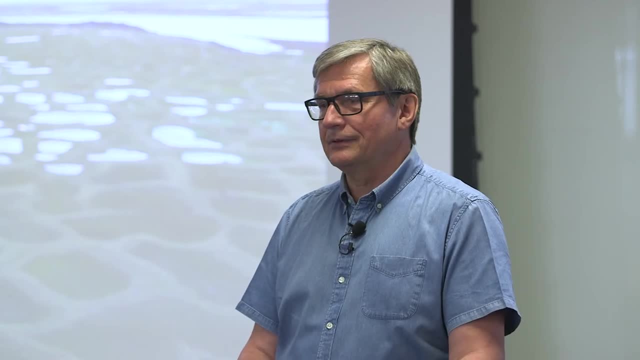 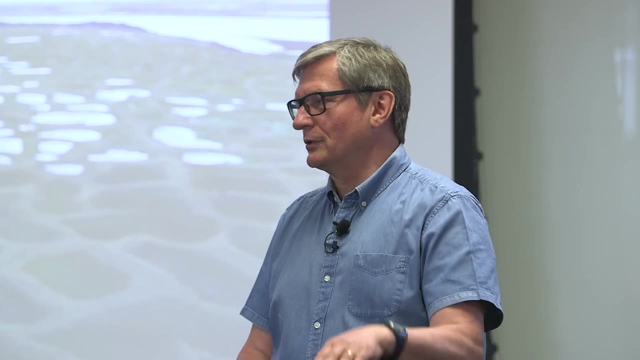 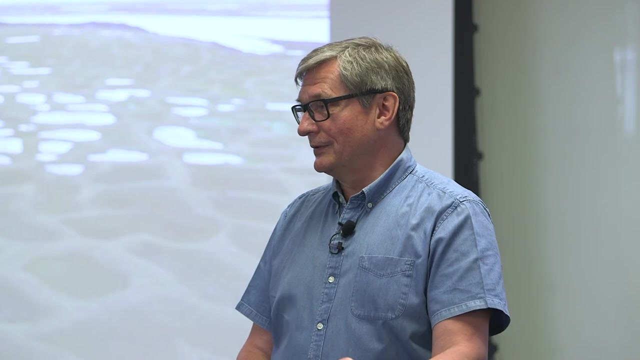 But it's still working. still And definitely. if it will be not that that will be major disaster already by now. you know much earlier than that, So it's a good example. There's many bad examples, like in Russia especially. 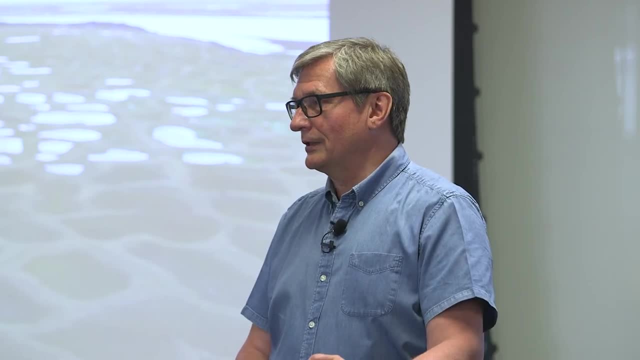 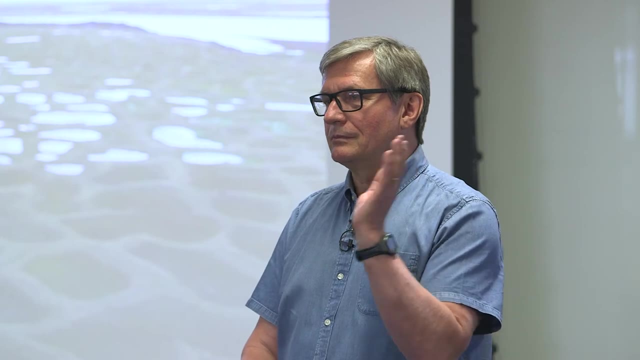 And they built this new trust Siberian pipeline to China. And they did exactly that: They dig the trench, put the pipe, fill it and there's massive problems right now. Somebody did send in a question on our forum and it's. 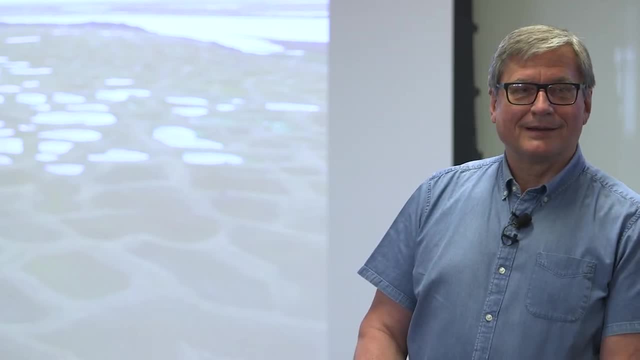 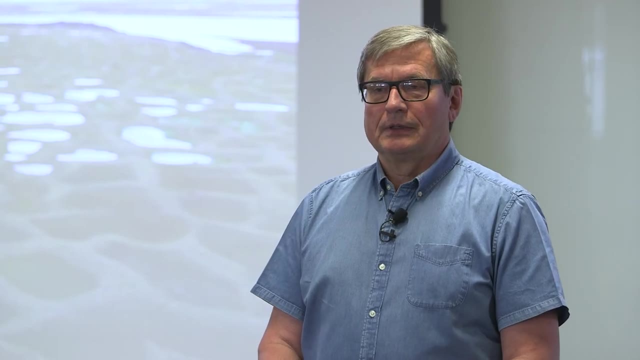 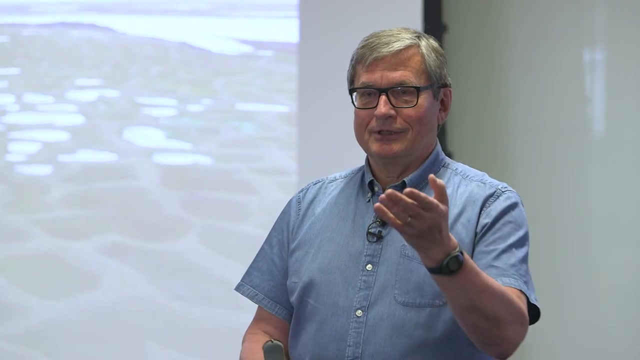 what's the difference between permafrost and Iceland's? Well, well, Iceland's, it's just some volume of ice, more or less pure ice, And you can create it in your refrigerator, So it could be on the surface. 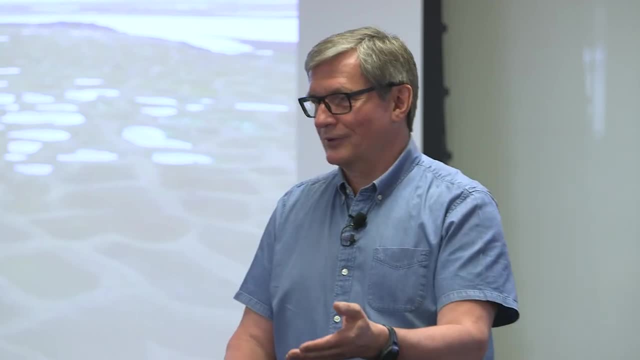 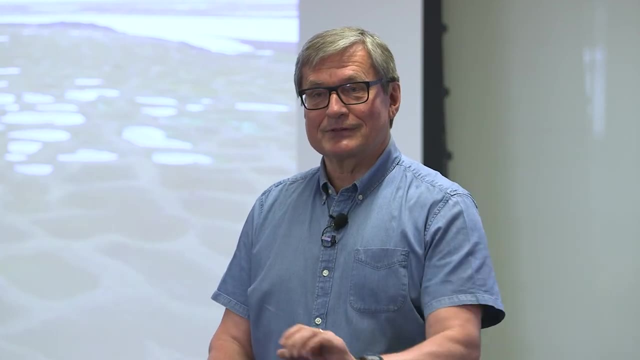 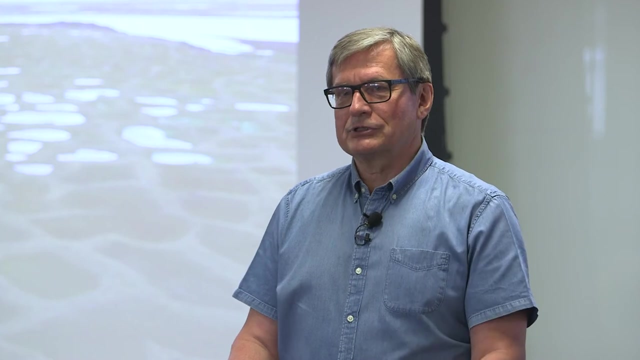 like this winter, especially when it's, you know, rain during the Christmas time, develop this huge Iceland's pretty much everywhere On the surface. It's not part of permafrost, because it doesn't fit definition. It's first of all in your refrigerator. 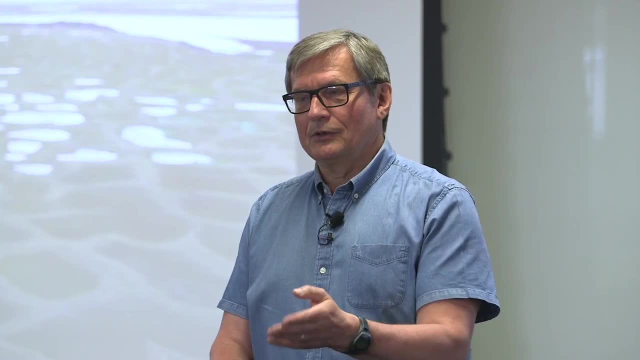 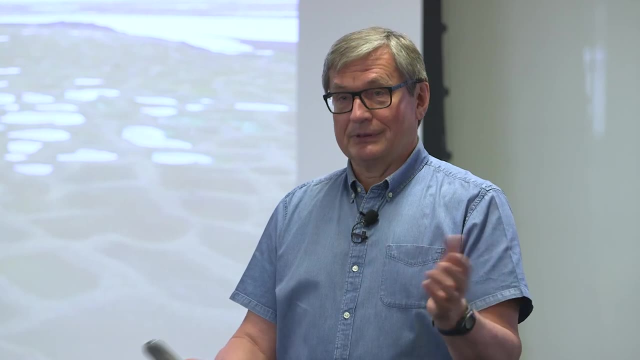 it's not natural material, It's artificial, And on the surface it's not survive one year- It's already gone by now. So what you need? if ice lands, it could be a part of permafrost, But the main thing is that. 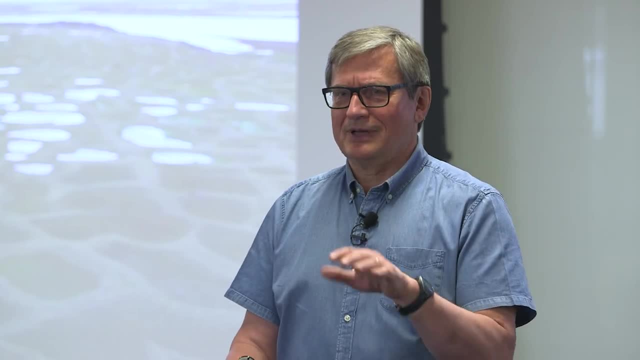 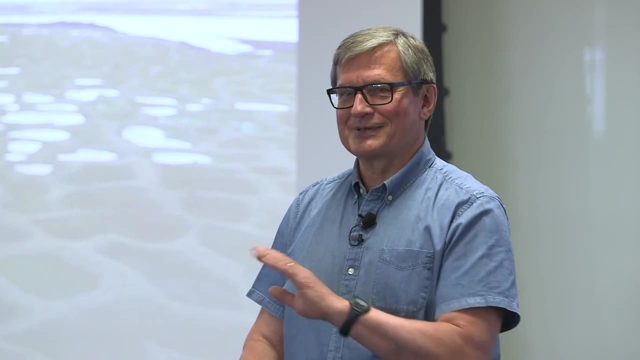 it should survive in the ground or near the ground- actually the ground better. We don't want to fight with with glaciers, no, There's much more of them. We will not win, But below the ground, If it will survive two or more years. 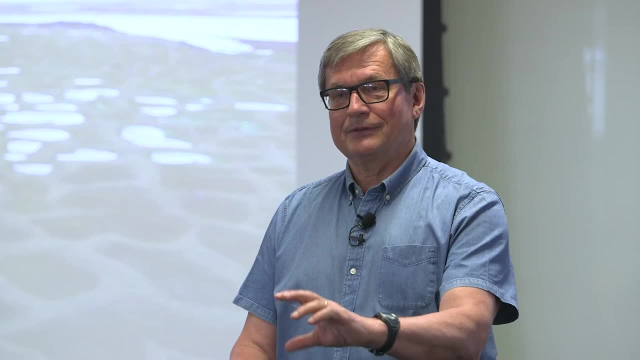 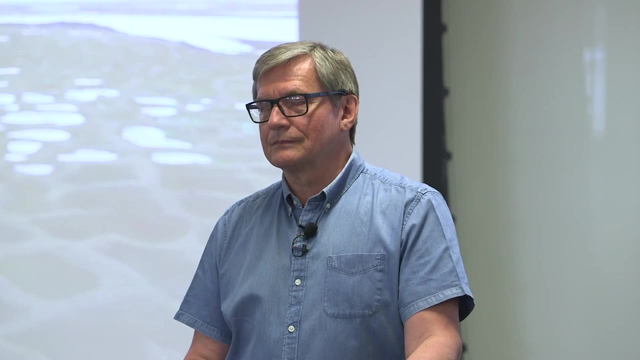 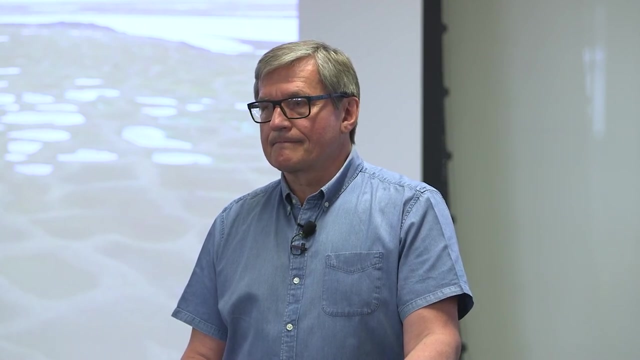 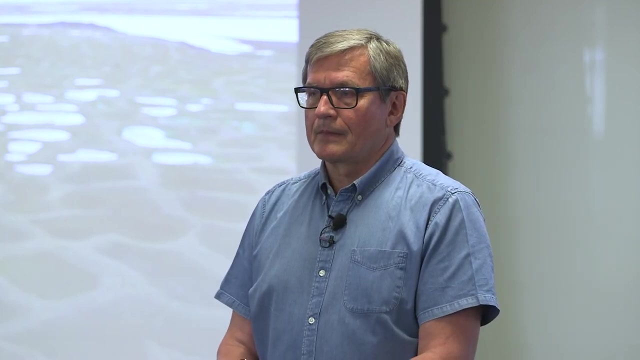 then you can call it permafrost And if it's formed naturally. So my question has to do with the air temperature data as kind of approximation of how much warming happened to the surface of the soils, And I'm wondering about radiative heat gain. 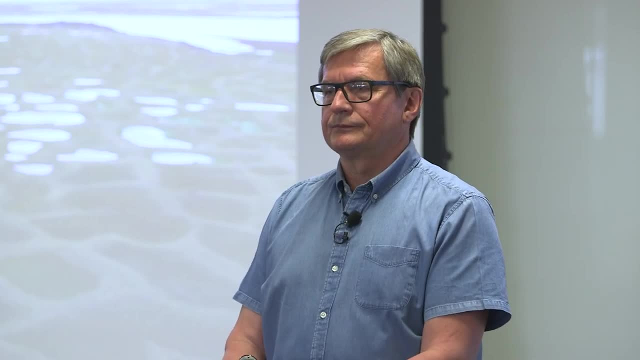 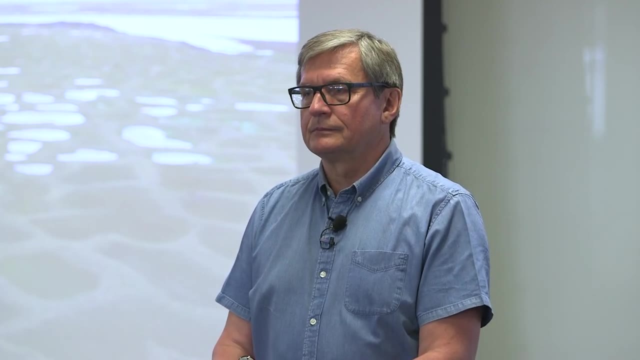 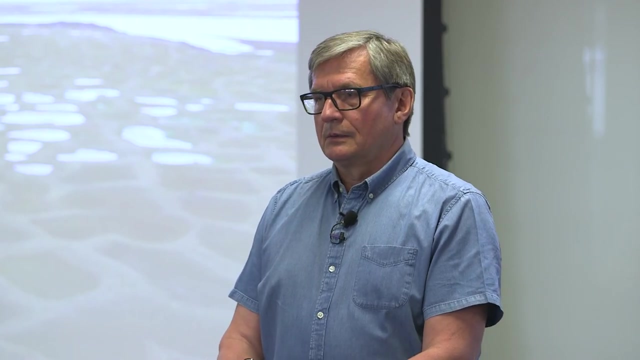 Heat gain from direct radiation from the soil And it has to do with this shrubification phenomenon that the biologists are demonstrating The increase in tall shrubs increasing radiative heat gain reasonably being transferred to the soil. Yeah, very good question. 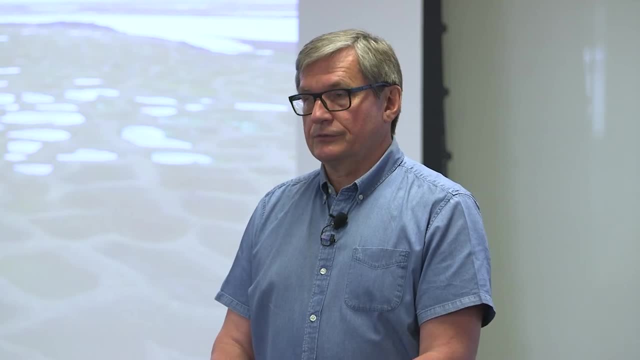 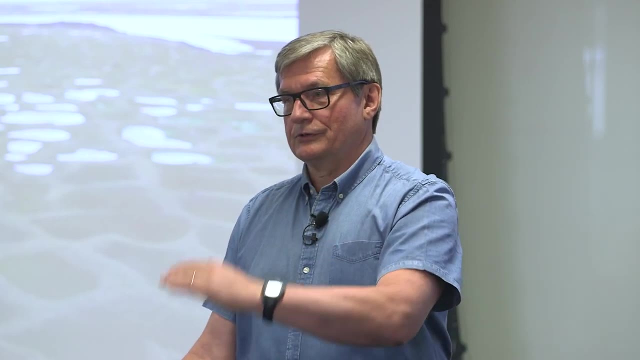 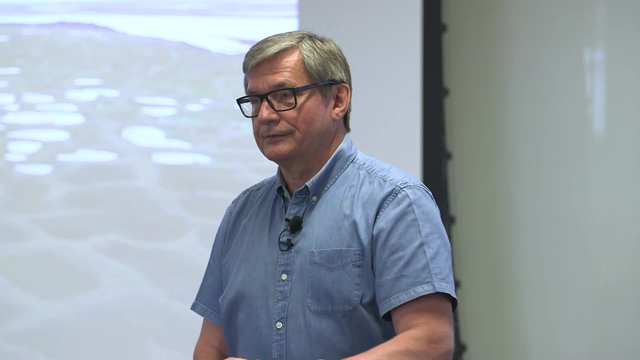 Of course the air temperature is a driving force. It's a major driving force, But between air temperature and permafrost there are several layers: Vegetation layer, organic layer, peat, active layer, material And, depending on properties of this, 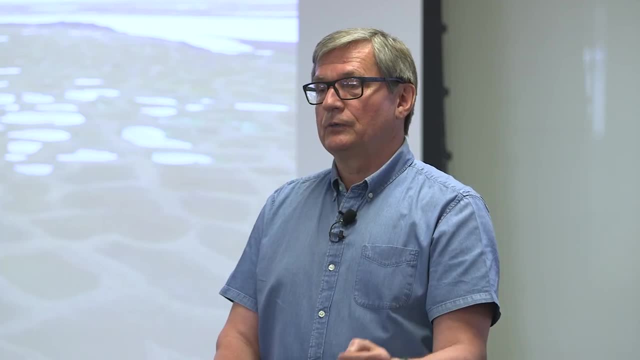 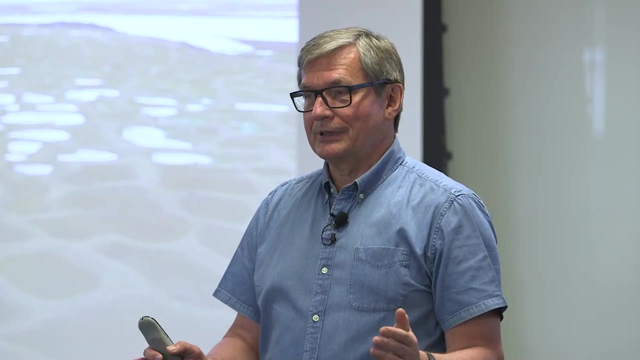 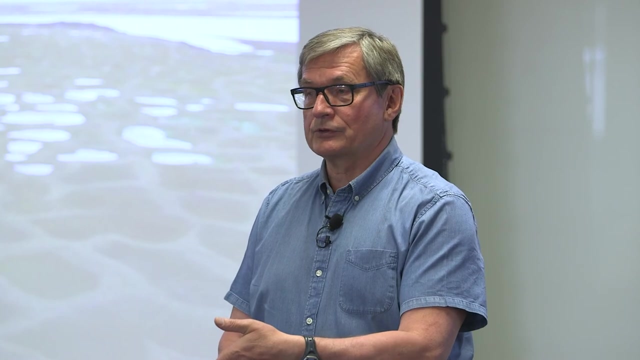 and some of them seasonal snow cover, Snow cover also in between, And each of these layers make this transition from air temperature to permafrost much more complicated than just simple. you know, the same amount of air temperature increase, the same amount increase in permafrost temperature. 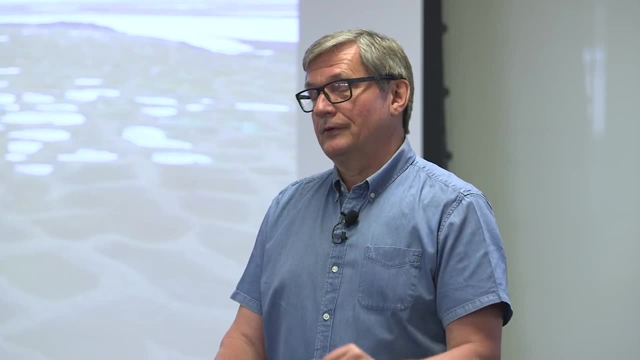 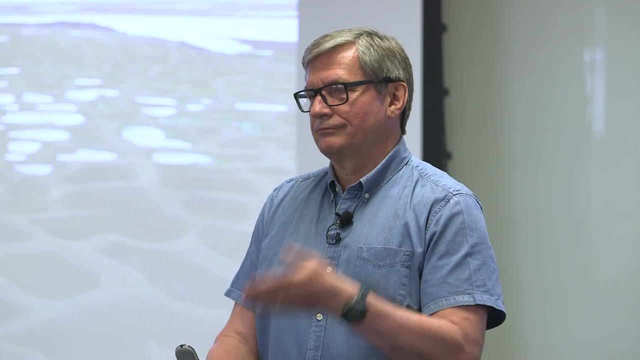 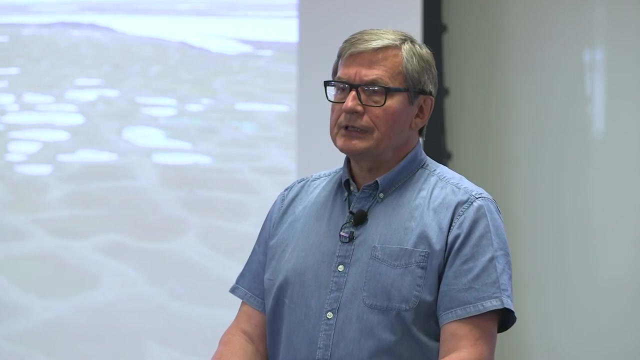 No, In some cases yes, In some very simple environments like bedrock somewhere and almost no snow, That will be pretty much the same Radiation. it could actually have some role. I would say it's still limited from, Because surface usually warmer. during the daytime because of radiation, It's colder than air temperature during the nighttime. So on daily average it's already very close. Snow surface- it's also pretty much daily average- will be very close to air temperature, So for that we can. 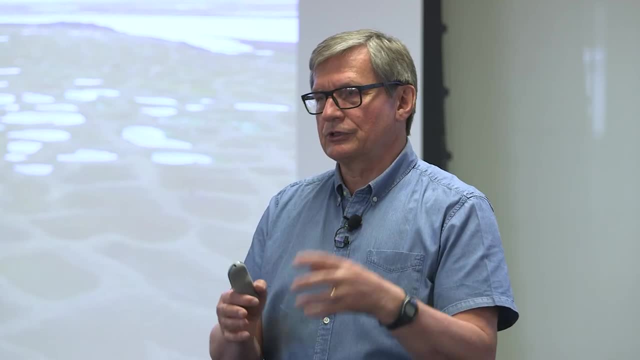 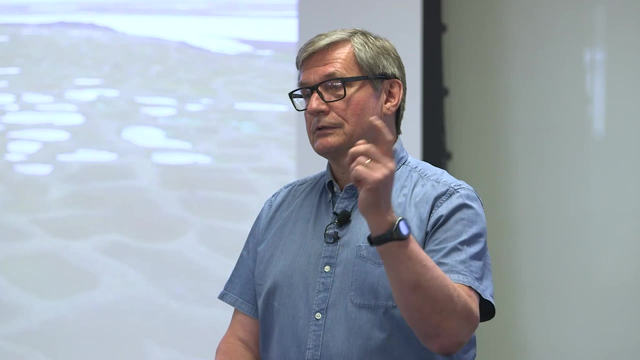 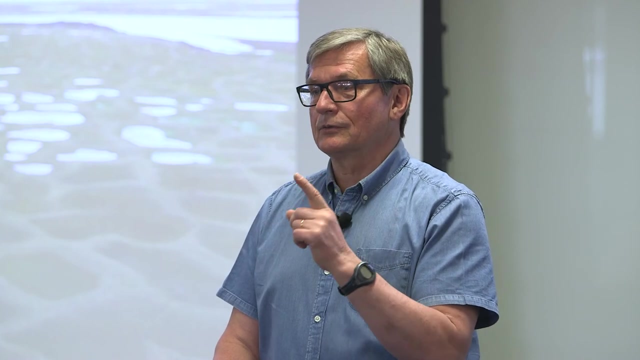 of course, in a very good model it's actually taken into account this energy exchange And shrubification. It's even more serious problem, Not only because it's changing albedo and because of that warming more, But also in more because of trapping of snow.